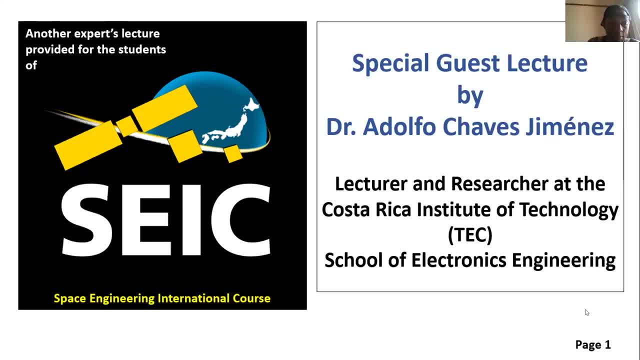 So we decided to go for carbon neutrality And we realized, working with the people from Forestry Engineering, that they need information about tree growing in places that are very remote areas. So we decided the sensors to actually measure, day by day, this information from tree growing. 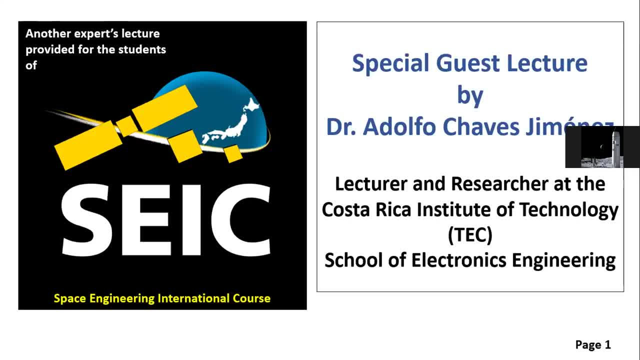 And the satellite is in a store-and-forward system. that was a proof of concept, showing getting the information every single day. so we proved the concept to be possible and actually we operate the mission completely. Testing was done by Q-TEC and actually also the. 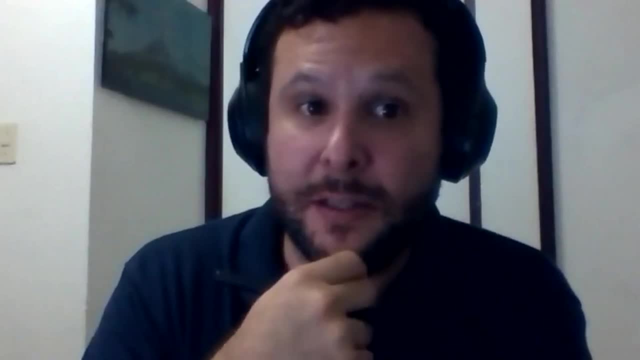 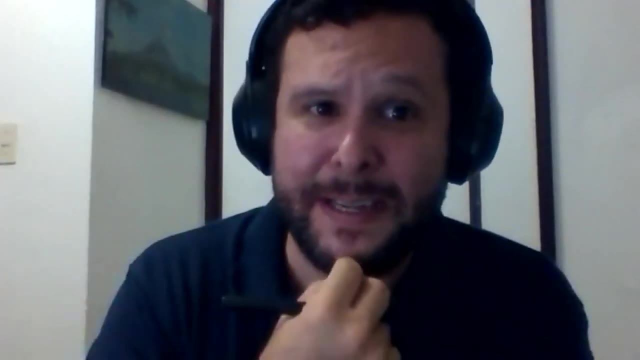 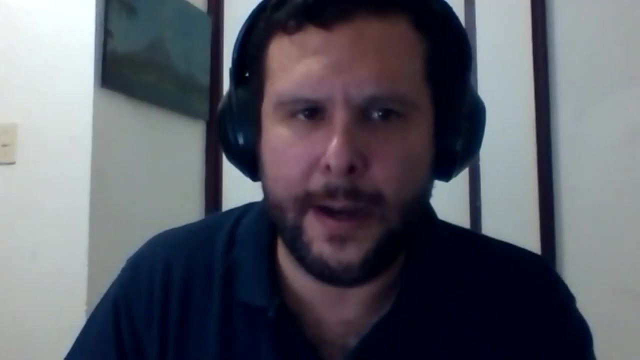 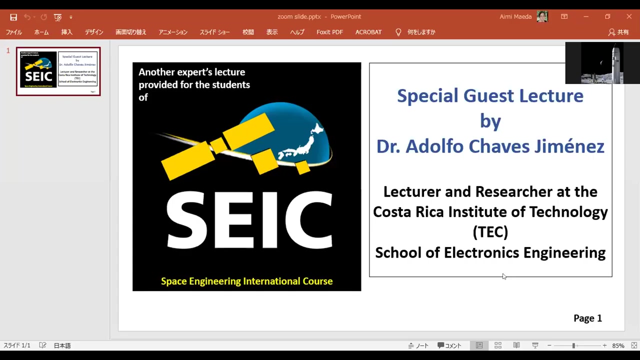 cooperation in every single of the steps for the space mission and supervision, more of evaluation of PDR, CDR and these kind of things. So satellite was almost two years in orbit. We had a period of very low atmospheric drag that you will hear about the atmospheric drag a lot today. today for you, tonight for me And yeah, 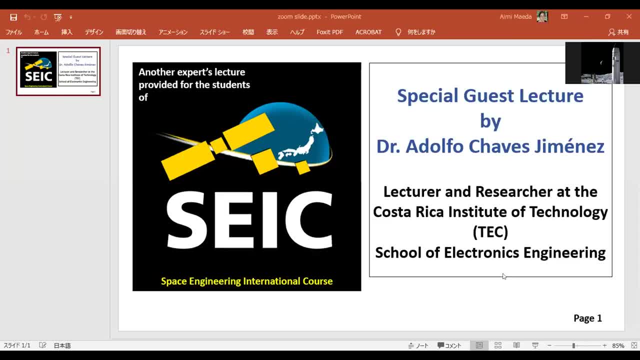 so the mission was ended around April this year And we have a very nice video that I could link you, and it's four or five minutes about the mission itself. Thank you, Rodolfo. Good morning everyone. we're going to speak into some of our floor. 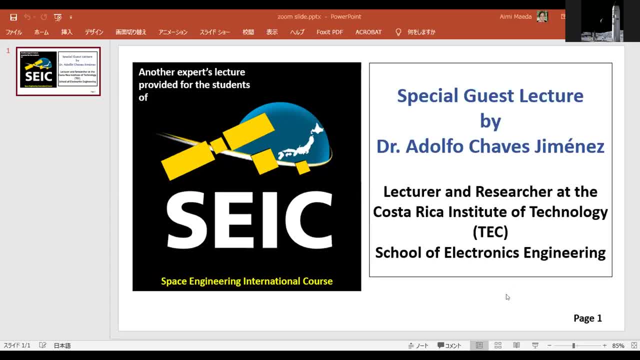 lids. but I also want to remind everyone in little bit of time- not now, just because I'm sitting on the requirings booth and trying to attend to some of what we're going to talk about Today was thenegative champion, month atraphy. 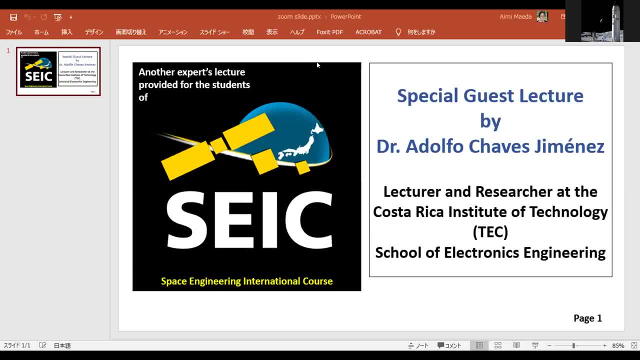 樣 board meeting and post, actually a very simple hosting conference with Rodolfo відio and with Rodolfo and and cable. So let's call, decide. okay, we're coming at deprivation and as very, We're going to start in about one minute. 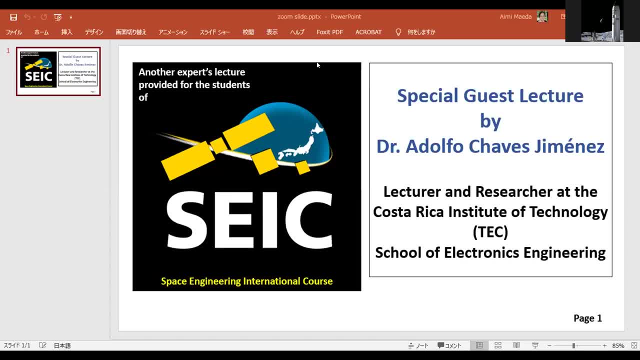 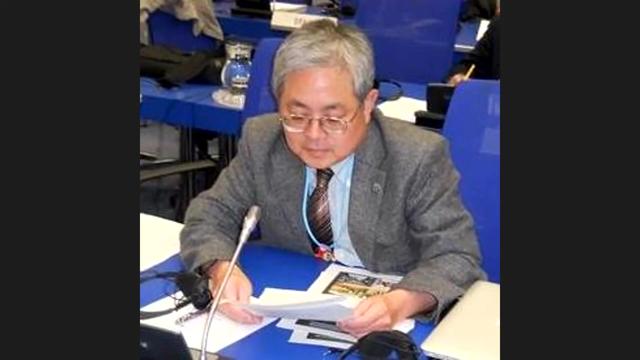 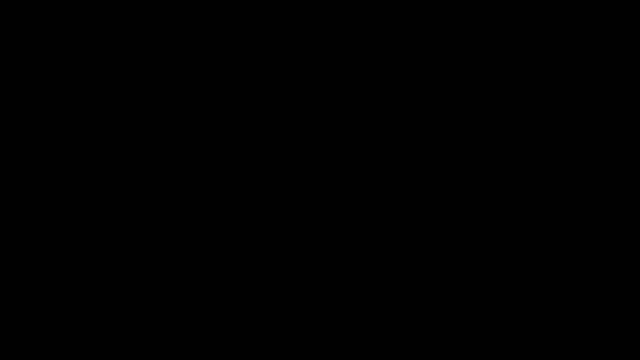 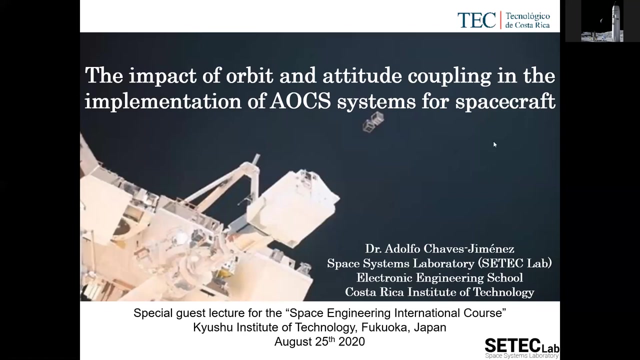 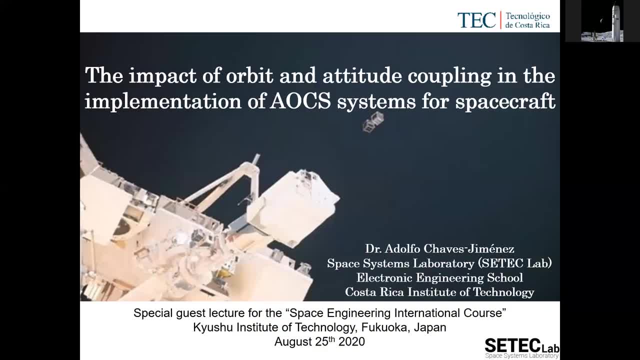 We helped test and launch their first CubeSat, which I believe is still up there. right, Dr Adolfo, It is already dead. It already burned the atmosphere. Oh, it did. Yeah, How many months was it up there? 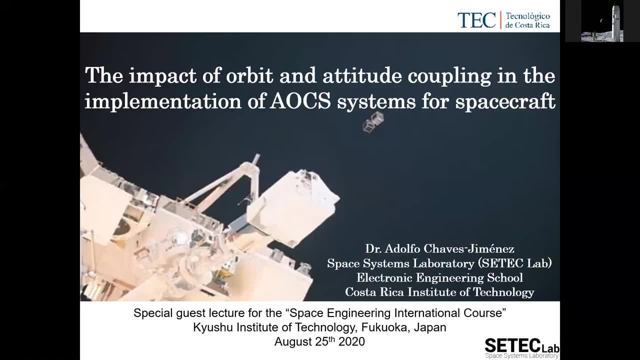 It was almost two years. It was pretty much it was a month close to two years. Okay, Well, with no further ado, I turn the floor over to Dr Adolfo. Thank you very much, George. First of all, it is my pleasure and my honor. 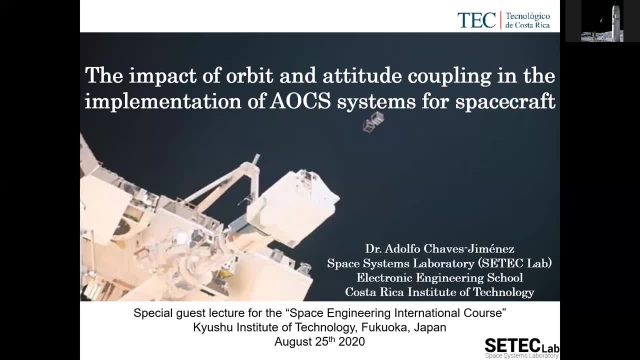 to be here with you today. I'm very happy to give a lecture for the Kirchhoff Institute of Technology. We consider our group and your group friends and we have been working together since the Irasu. But Irasu is not the only limit of our cooperation and actually giving lecturing. 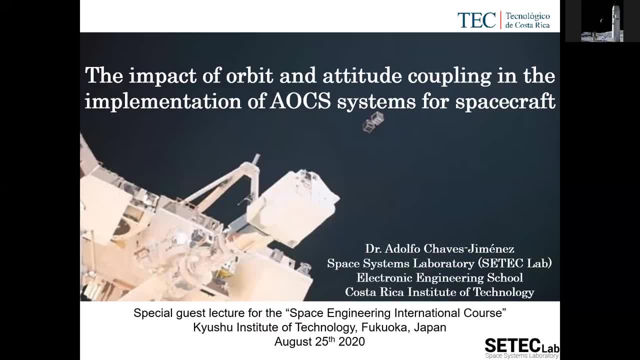 This is the first time, but we hope it's going to be many times in the future. Right now, in my lecture, I'm going to talk mostly about the things I learned in my PhD, and why am I going to talk about this? My objective with this is that whenever, especially if you work in control systems, 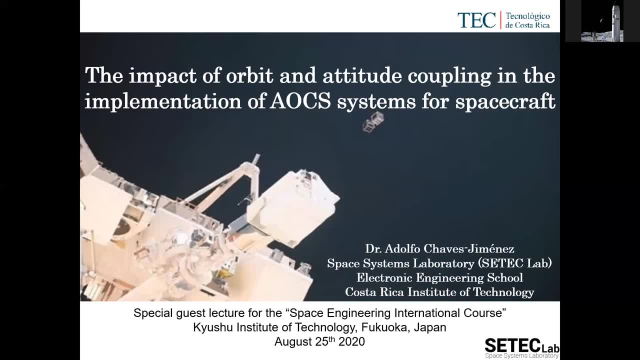 for satellites and estimation systems for satellites. usually, when you work in estimation and control, you think of orbital dynamics and you think of attitude dynamics as separate matters. Actually, you have Okay, Okay, So you have orbital dynamics experts and you have attitude dynamics experts. 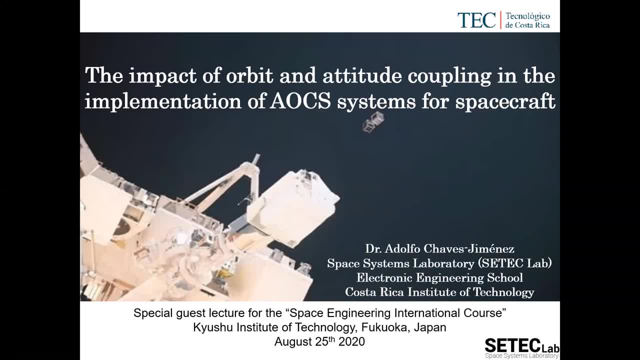 and they usually don't talk to each other. In my PhD, I have to learn from both and I have to become both of them. And why becoming both of them? Because for the future of the missions in space, it would be every time more important. 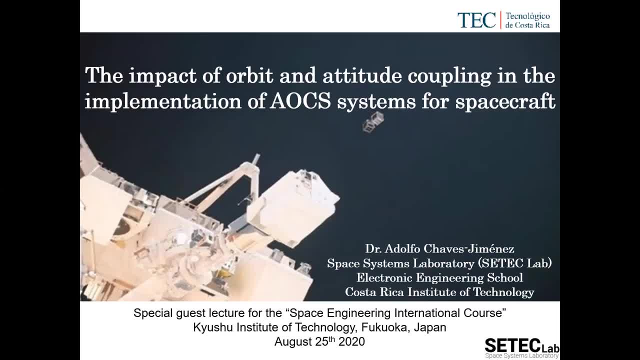 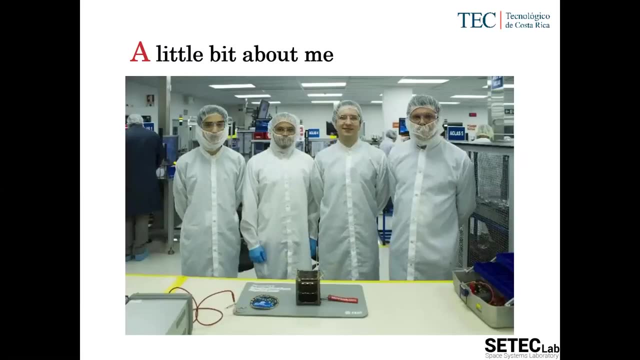 to take into account the coupling that exists between orbit and attitude dynamics In the implementation of the Attitude and Orbit Control and Estimation Systems or spacecraft. So first of all I'm going to talk a little bit about me. Already, George did an introduction. 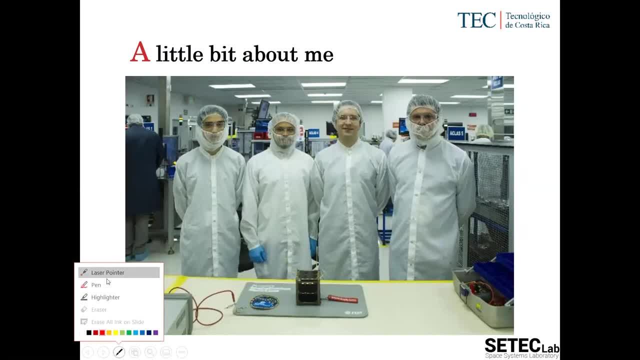 As George said, I was part of the project Irasu. This is the Irasu satellite. This was the first satellite of the country and actually the first satellite of Central America. This was assembled. This was done in our laboratory in Costa Rica. 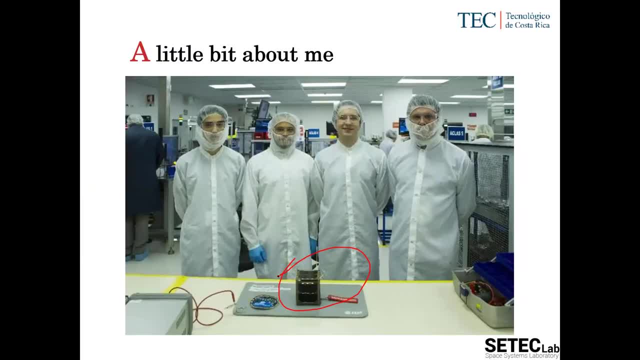 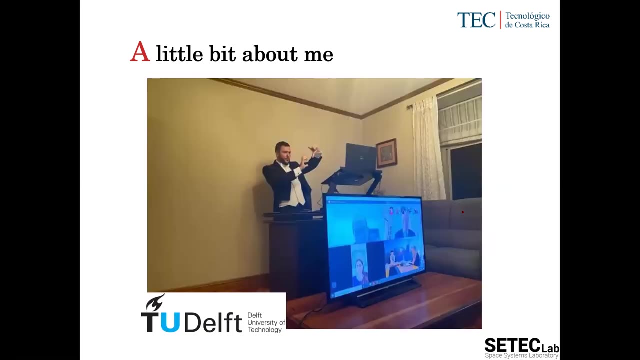 It was assembled in a company, because we don't have a clean room as you do, And later, after that, it was sent to QTech for testing. I'm the fat one, I'm this guy. So also, I just finished my PhD in COVID times. 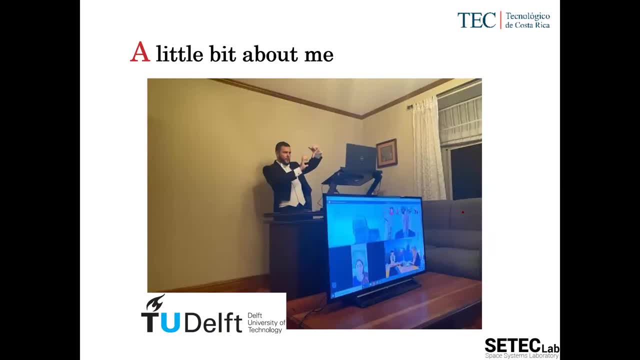 My PhD is in the field of aeronautics, So I have a PhD in aeronautics. This is a little bit in the subject that we're going to talk today. So this is how a defense looks for the Netherlands version of COVID defense. 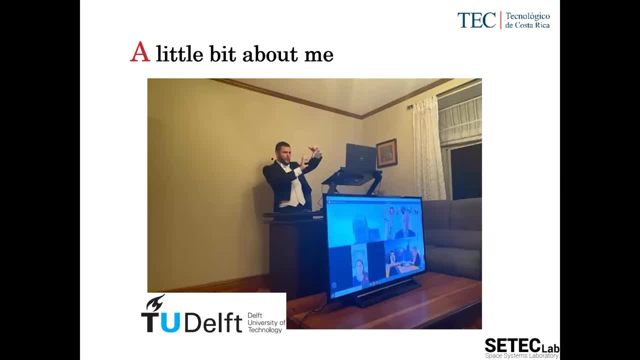 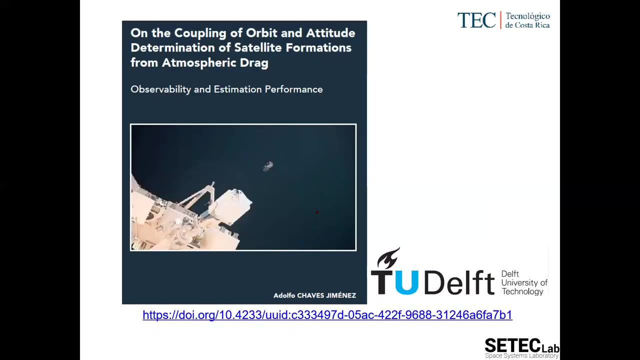 With me in the fancy suit- which I don't own, by the way, And you know, this screen is just connected for my family to see what was happening. So I graduated this year as a PhD at TU Delft And this was my thesis. 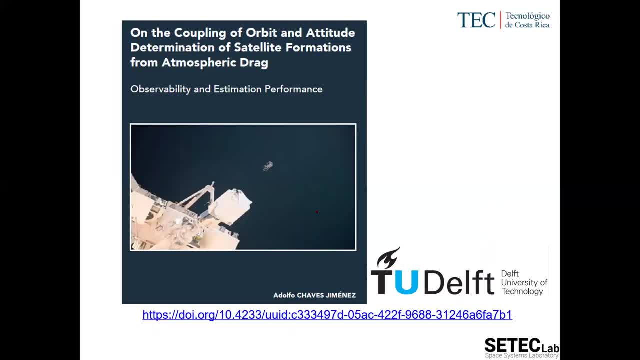 The thesis. the objective of the thesis was to answer the question how the consideration of Copley forbidden attitude determination influences the efficiency of the estimation of dynamics of spacecraft. This is the link. I'm going to send you the presentation And if any one of you is interested in reading the thesis, it's completely open at TU Delft. 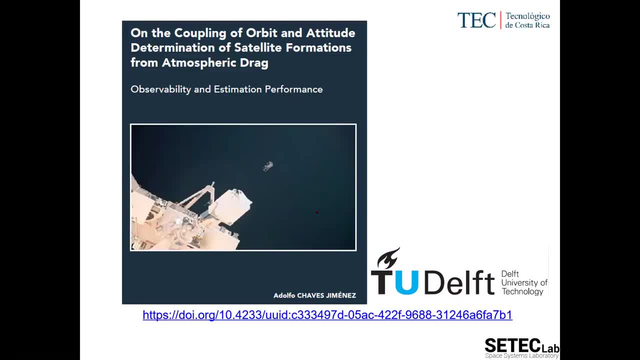 So if you're interested in reading the thesis, it's completely open at TU Delft, So it's material that you can read. You can ask me anything. So this research work was done at the Delft University of Technology in the Netherlands. 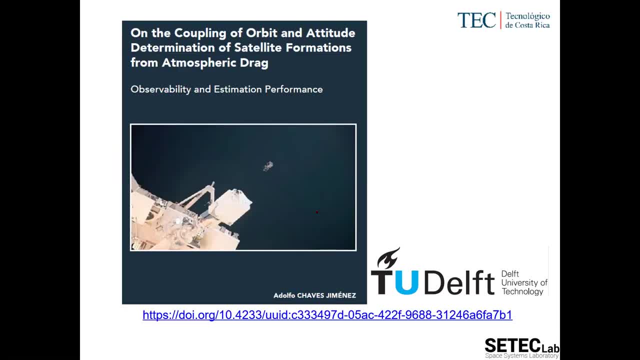 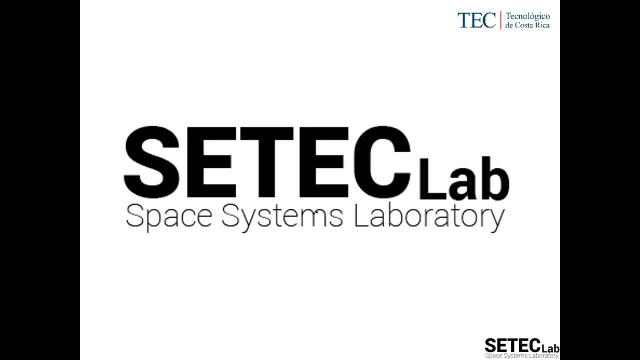 And now I work in Costa Rica, But most of this work was done there. Okay, So after talking about me, I want to talk a little bit- just an introduction- about our laboratory: space systems laboratory, The CETEC lab. This is the laboratory. 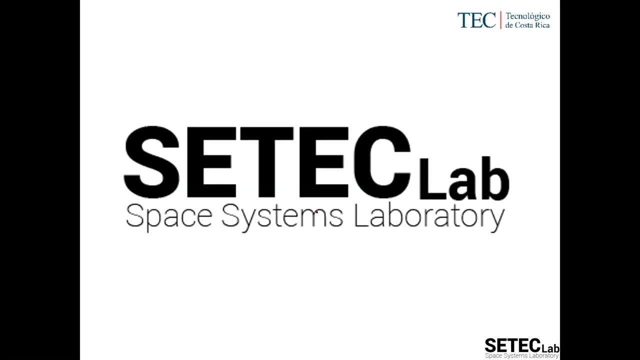 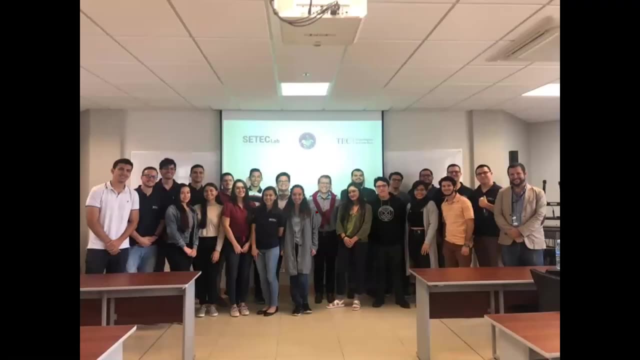 It's the first of its kind in Costa Rica and Central America. The laboratory was founded with the objective of using space engineering in Costa Rica, And it's constituted by students and lecturers in the Costa Rica Institute of Technology. This is a photo of last year, when we could, you know, be next to each other. 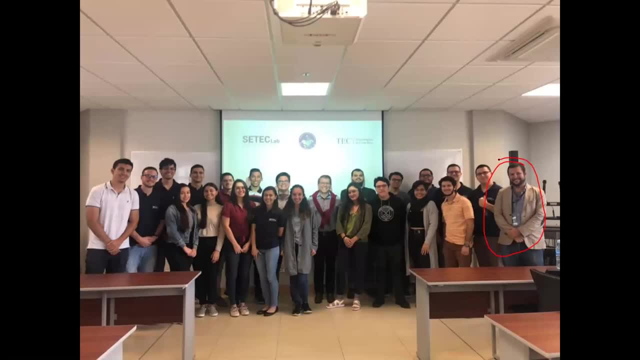 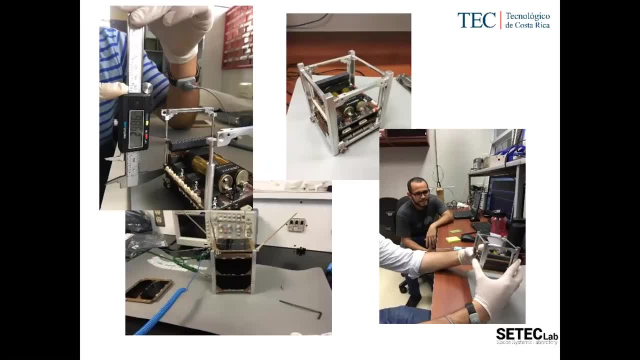 And the project that was the cause of our of us being born was the Ida-SUV project that I talked a little bit just before. The Ida-SUV project: this is the construction of Ida-SUV project in the space systems engineering laboratory. 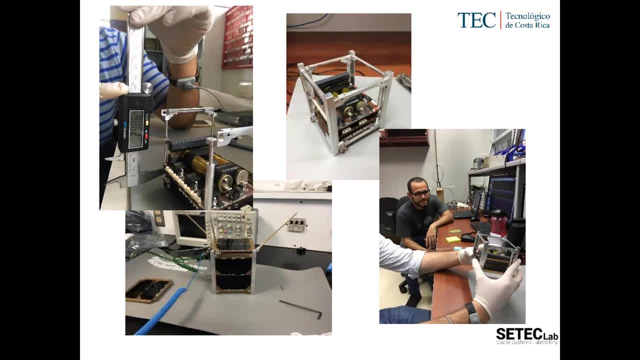 Somebody here is saying in the chat that you cannot see the share screen. Is everybody else okay? Because yeah, so it's a one person problem, I guess. Okay, Sure, Okay, Thank you very much. Thank you very much. 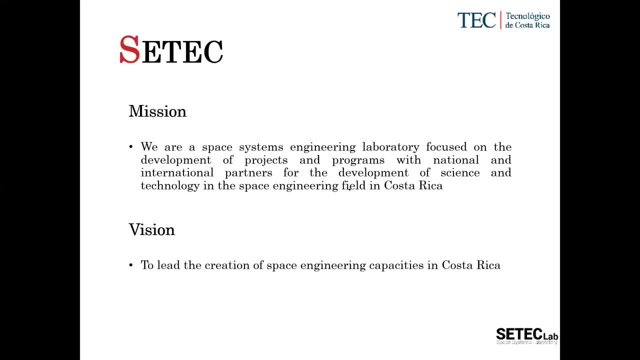 Okay, So our mission- I'm not going to talk too much about this because we need to get into our matter- We're a space systems engineering laboratory, the first in Costa Rica, the first in Central America, And our mission is to create a space system engineering laboratory. 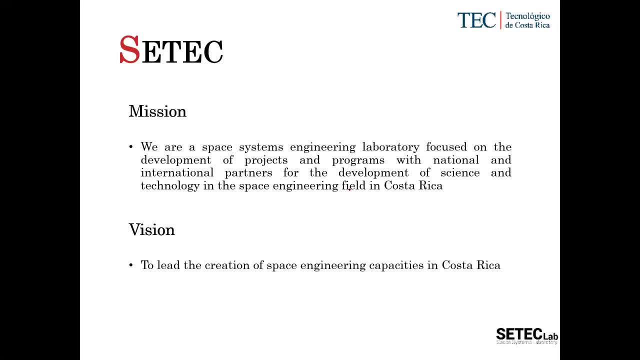 So our objective is using space engineering as a tool of development, as probably many of you who come from other countries to Japan to learn about space engineering have- the objective of using space engineering as a tool of development, A very powerful tool, by the way. 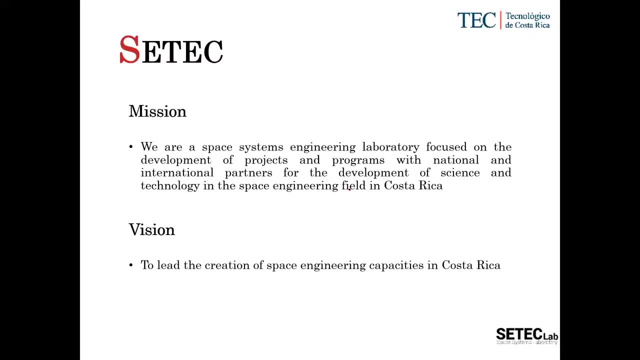 And our vision is to lead the creation of the space engineering capacities in Costa Rica. Currently we're working on a satellite project with the George Washington University, developing the attitude and control- the attitude control system of their satellite and the remote communication systems for their satellite, and also working 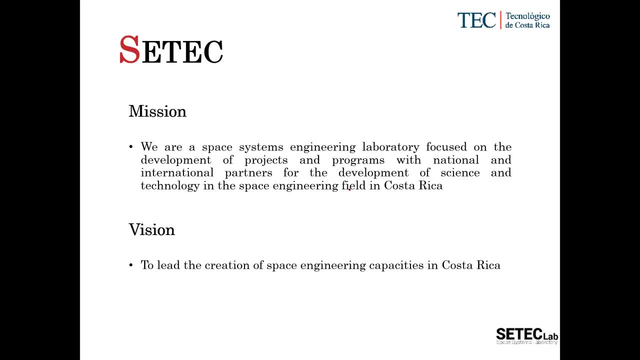 cooperation on the BIRDS project with you And the CETEC lab was also the lead technical lead for the proposal of the Costa Rica Space Agency, which is right now in Congress actually being discussed this week. So, okay, let's talk about spacecraft, post-dynamics, okay. 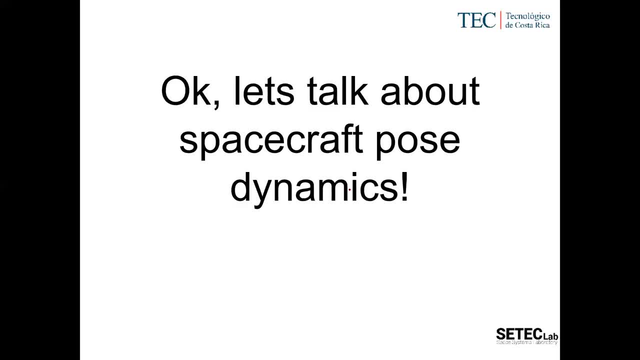 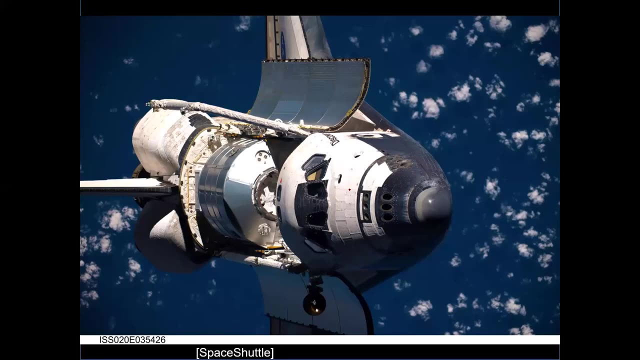 This subject. I have to say I really, really like it. I like dynamics, I like control. It was very, very interesting to learn about these kind of things. why? Because when you see this kind of spacecraft which doesn't go to space anymore, 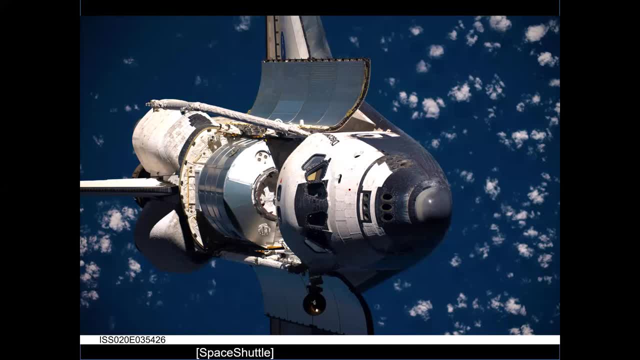 people used to say: you know, this looks like a plane because in the atmosphere you land on an airport, but this has no use in space. and the question is: is it really so? does it, does this have any use in space? day? the wings of the of the spacecraft. is it important? 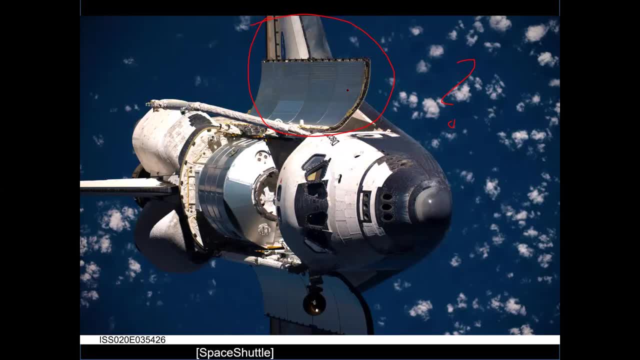 is it more important? actually, this is the question we were trying to answering and the question we're answering and the and the answer is yes. I want to some point, and the important thing, if you are a control engineer and is going to be more and more important in the future, is to know when is it going to be taken? 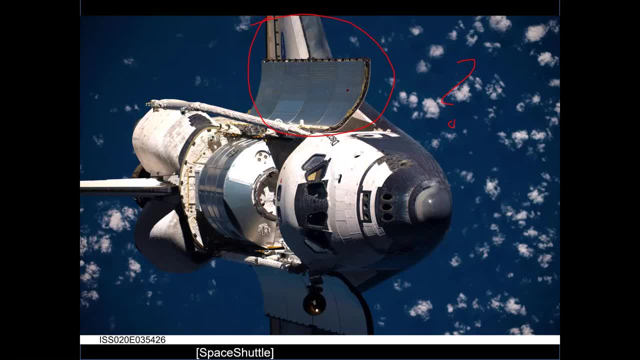 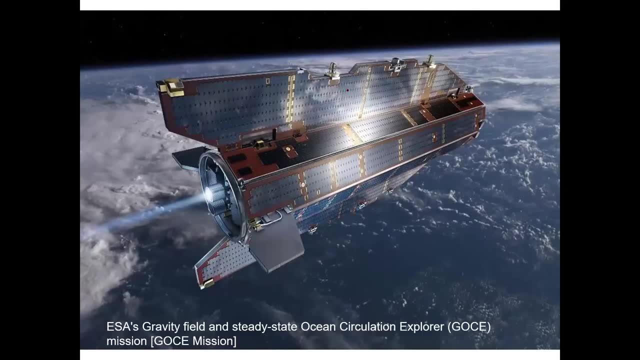 into account. is it important or not? we know many different cases when this is important. one of these cases was, I have to say, one of my favorite satellites, because it looks like Batman satellite. honestly, this is so cool. it's so really awesome. this is there. a goes. 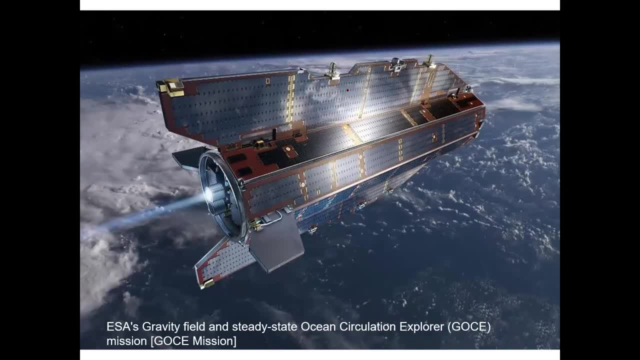 experiment from ESA and the go see the goes experiment from ESA has a particularity: that he had to be really, really, really close to land while still being in space. I mean, I'm not going to talk about the mission itself, I'm going to end in the OP. 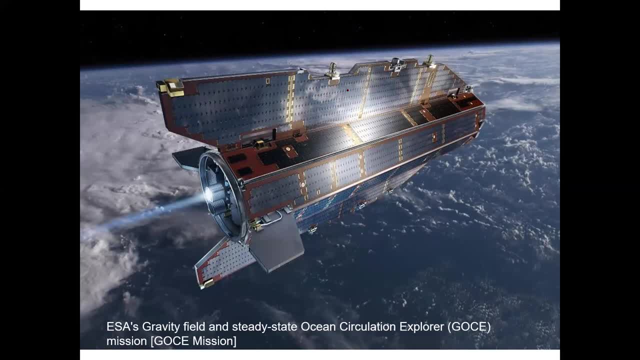 going to see it only from the control engineering point of view. So you need the satellite that is close to space, but you need the mission not to last- I don't know- six months, three months or something like that. Then this satellite was designed with aerodynamic considerations. 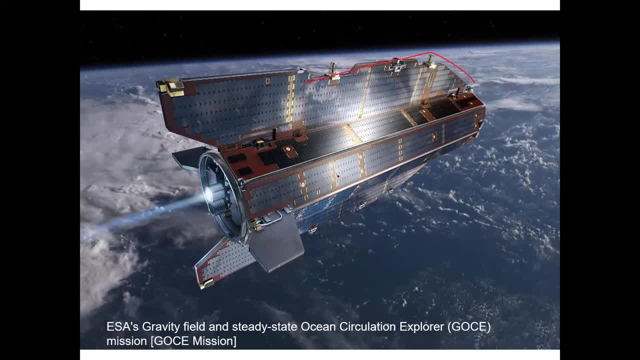 As you see, this profile is some sort of aerodynamic. This has these fins, It has this kind of thruster and things like this, because it was working approximately at 260 kilometers above the Earth's surface, And for any one of you who is already in the 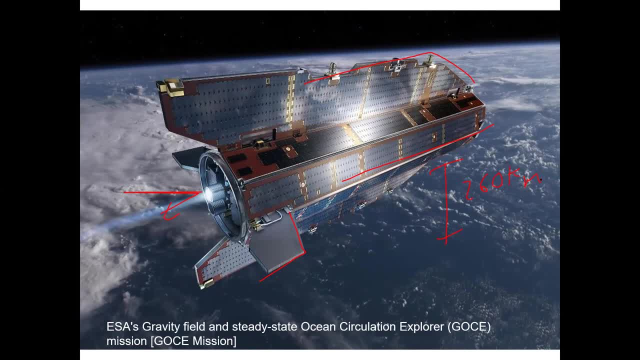 astrodynamics course or already has been in the astrodynamics course. you know that 260 kilometers is very, very, very low And probably missions on this, on this altitude, will take, if not control, somehow less than six months. But you need this kind of. 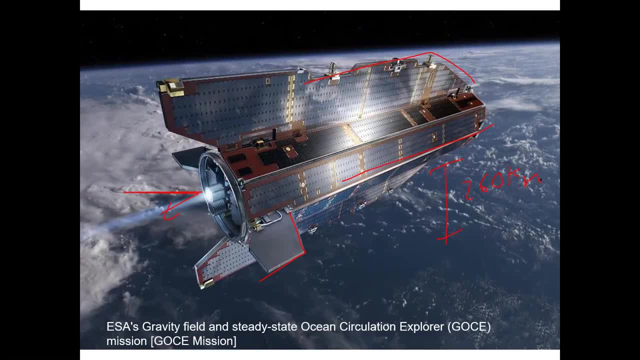 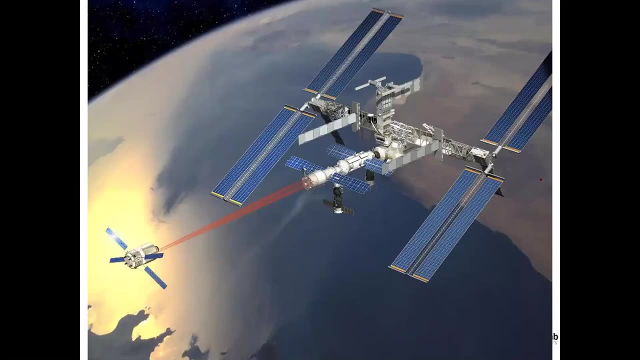 satellites to last not six months but years, maybe two, four years. So this satellite already proves that this consideration is important, the consideration of this perturbation Now, usually classically in a spacecraft, relative dynamics, one of the typical considerations, and this is the typical example. 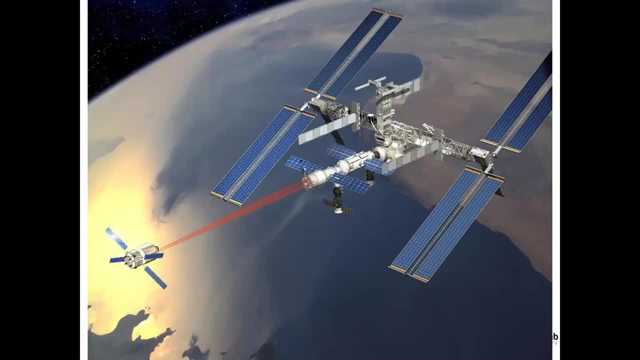 which any aerospace student and professional would think about, which is the close encounter between a spacecraft and International Space Station, or a spacecraft and another spacecraft, like the reparation of the Hubble telescope or this kind of missions, In this kind of missions. 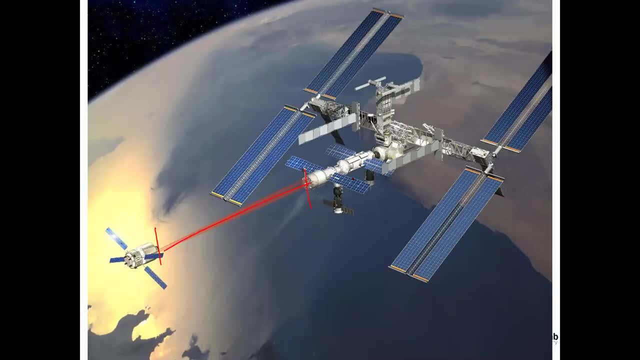 actually there are some equations, and I was. when I was preparing this. I was about to get the equations but I didn't get them. They're called the close-away Whitshire equations. Sorry, sorry, it looks awful, Let me erase that. Okay, let's go again. It's the close-away. 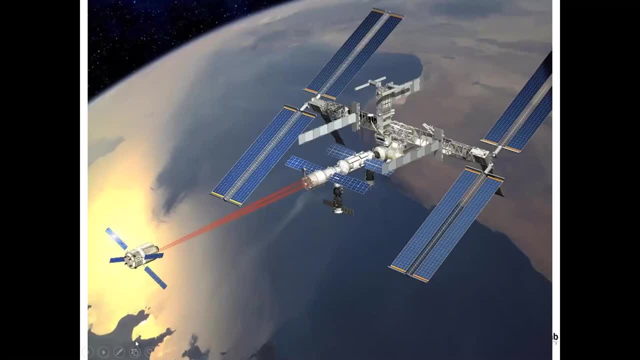 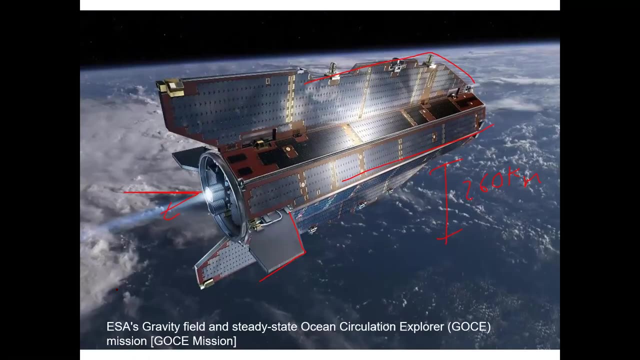 Adolfo, can you go back to the previous slide? Yes, So it's only 260 kilometers. Now, when it's 160 kilometers above the Earth, how can it possibly stay in orbit? Well, there are different things. The effective area of this spacecraft is very, very low in. 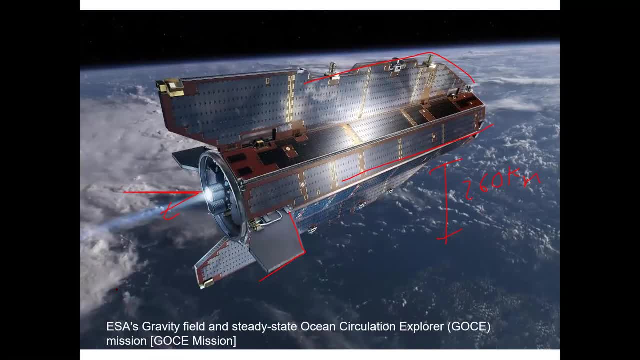 relation to its weight, in relation to its size. Actually, the Eon thruster was keeping it in orbit. with the continuous operation of this thruster And the, it uses the aerodynamic force and torque to actually lift a little bit. i don't know the details about the control. it could. 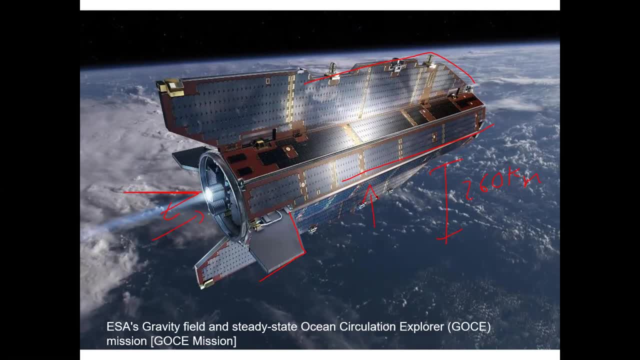 be a complete conference itself. but, yeah, it uses all these these, uh, these interesting steps and actually, uh, this is one of the things that i want to come at the very end, because i think this is possible to be done in a cubesat. there are a few proposals in that sense, but i think it would be a 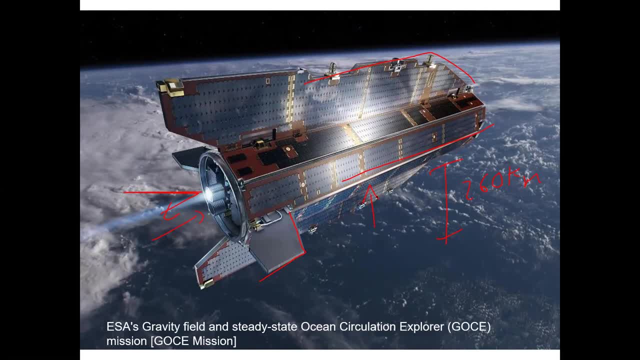 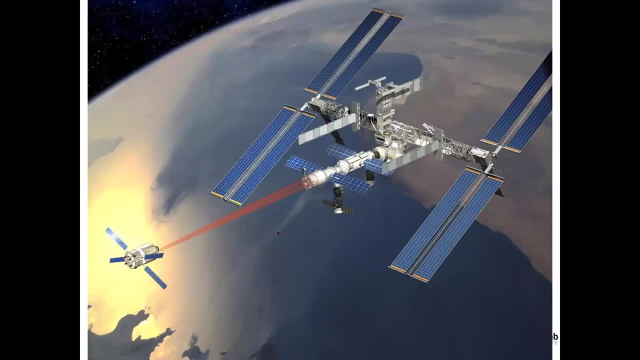 very, very interesting research in the future. and what fuel is it burning? i don't know. honestly, i i don't remember. sorry, okay, thank you okay. um, yeah, so, as i was saying, since the 60s, uh, 60s, 70s, there have been some equations and relative dynamics that are called the cw equations. 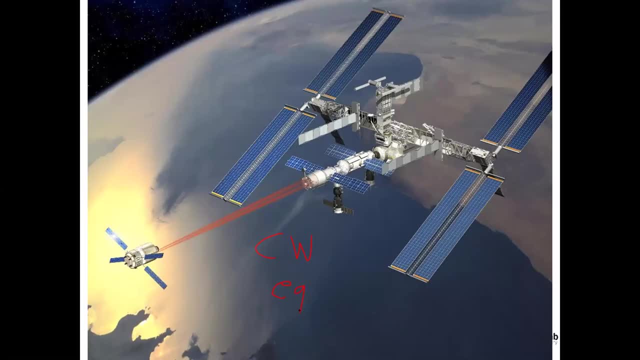 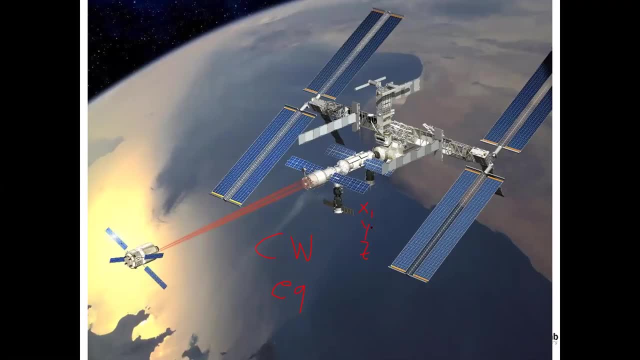 x, y set. say one, one one and x two, y two and set two. and then you say, well, relative dynamics, is x, relative um this, this i'm going to say, this is x1 um this one like this, like a vector, and this is x2 like a vector. and then you say relative dynamics. 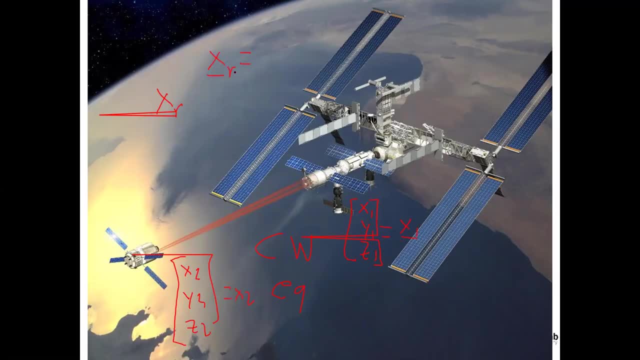 as a vector, of course, is x2 minus x1 and this uh dynamics, the variation of this uh relative dynamics, meaning that the partial derivative of x are sorry, sorry, like in this, with respect to time, where, um, there is uh this, these equations that i'm telling you about, and they are linearized version of equations, they are 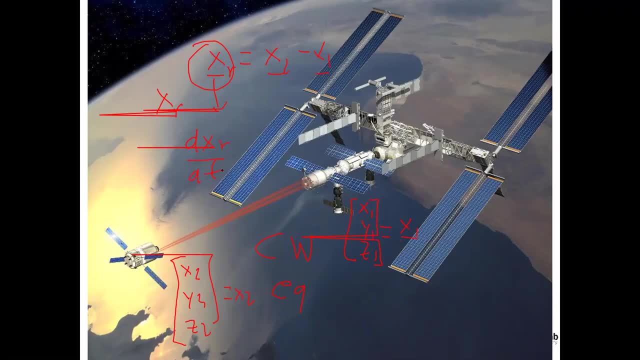 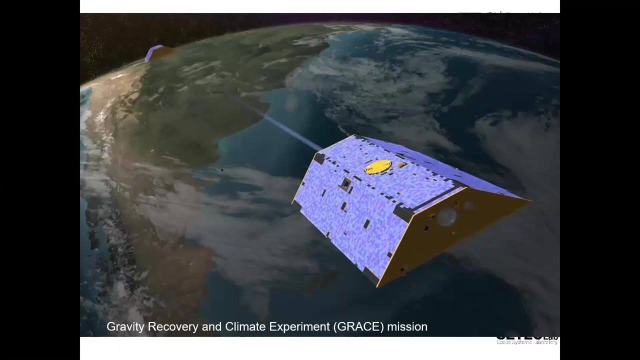 only valid when you're very close to your target, when you are in circular orbit, and it doesn't consider any sort of perturbation and it's only about orbital. but this has changed a little bit more because now we're working in formation flying configuration. but this has changed a little bit more because now we are working in formation flying configuration. 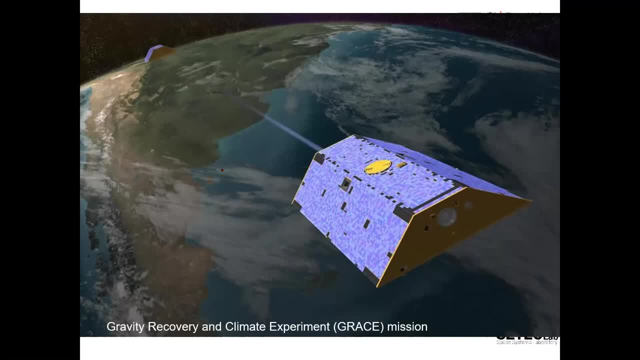 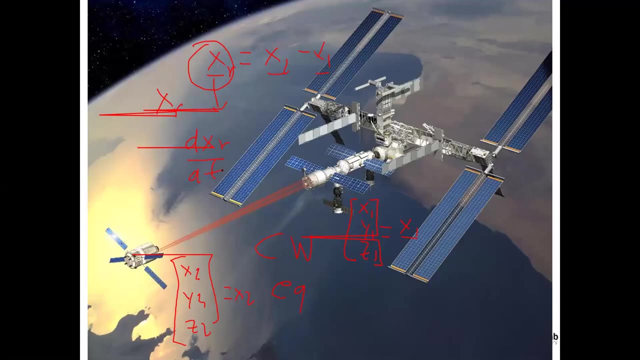 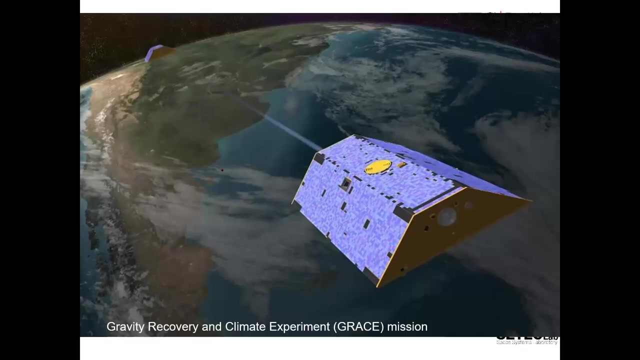 that work together, that have to need very, very precise estimation and control objectives, and there are not as close as this kind of things. this, this, this configuration could be, you know, valid for one kilometer or less, but we're talking now about constellations of satellites that could have separation of. 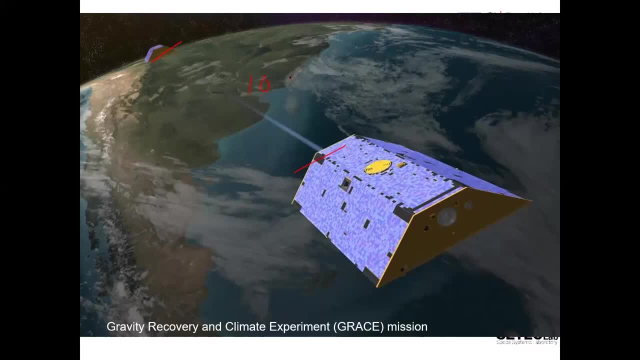 hundred hundred kilometers, four hundred kilometers or things like that. here these equations are no longer valid and here the consideration of coupling and the consideration of perturbations could be the difference between having the position that you need and not having the position that you need. so this is. 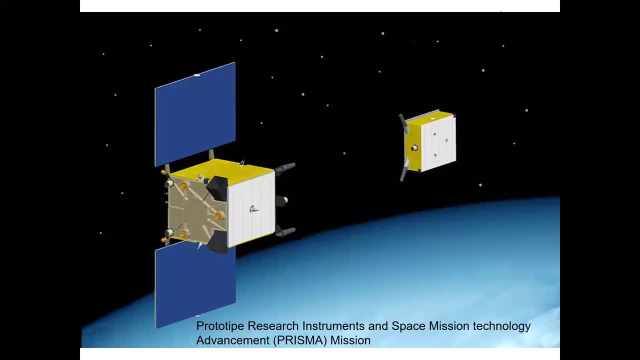 another example of this kind of missions. the prisoner mission was proposed in order to test formation flying for spacecraft, and what you get here is that you get very precise GPS, very precise connections and data from sensors, from all the sensors that you're working on this satellite, but there is a limit to these sensors. I 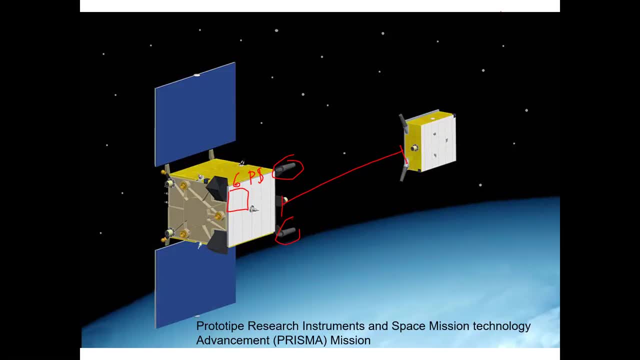 mean, if you want more precision- usually every engineer, especially us, that I'm an electronic engineer- by by formation, you just get more instruments right. where's the band? what's the advantage of the model of dynamics that you have? well, the advantage is that, with the same hard work, exactly the same hard work, you 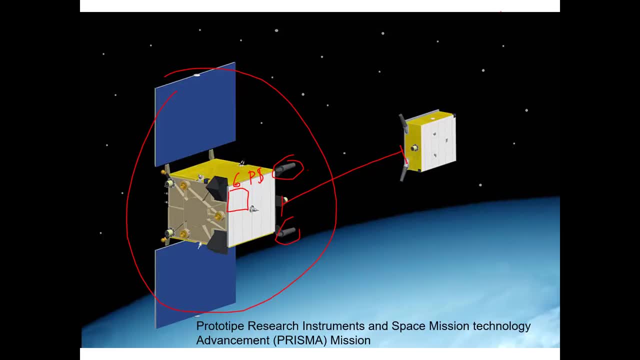 could get more precise estimation results. so imagine that just by using better models for estimation and control, you get better, better results without spending anything on hard work. usually- and this is this is something that is really funny- aerospace engineers are very conservative. I mean conservative level, having microcontrollers from the 80s in the 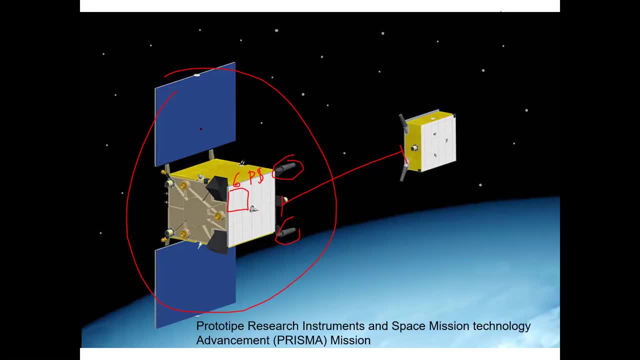 space shuttle in 2011. what? and this has been an approach that has been useful, because we're talking about safety, we're talking about PLRs of nine and this kind of things, but we're not taking advantage of the Moore law, we're not taking advantage of the fact. 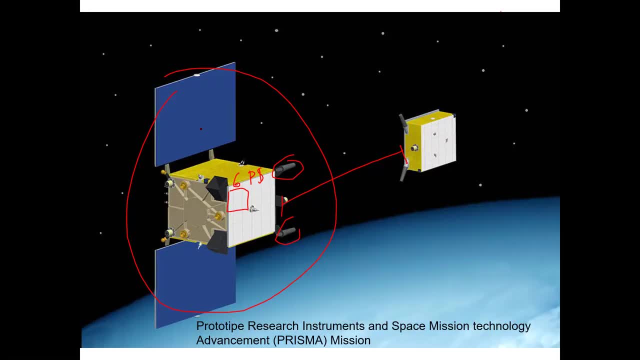 that the computer power of systems is doubling every two years and actually the use of CubeSats has allowed this to happen and that's why we're talking about the nuestros kind of advancement to be done. we can use CubeSats to take advantage of the. 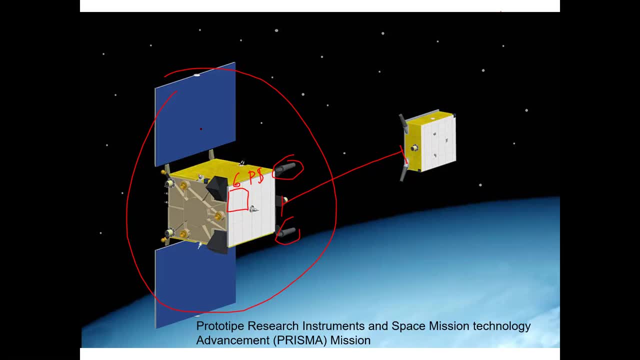 computer power of the current micro controller microprocessors and actually have advanced dynamic models in other places. for this advanced dynamic models were not used, were not used before. I mean for decades. in the area of amplitude and orbital dynamics, the efforts of many scientists were have been focused on simplifying models in order for they to work on the microcontrollers. 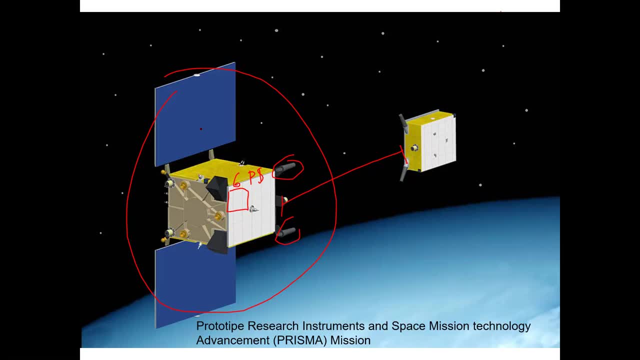 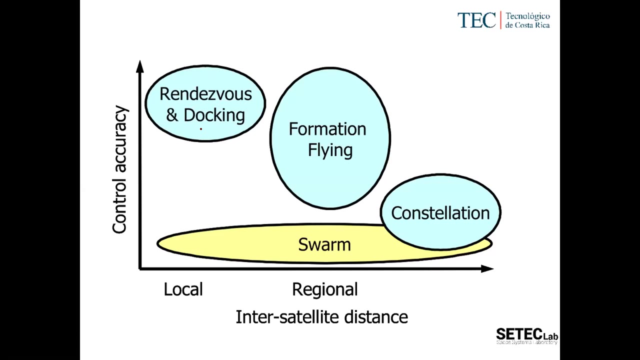 But I believe honestly that this, this is no longer a requirement And actually the best models possible could allow us to use the same hardware, no more masks, and have better results. So, in that sense, what I can tell you is that probably you all know that this is a tendency. 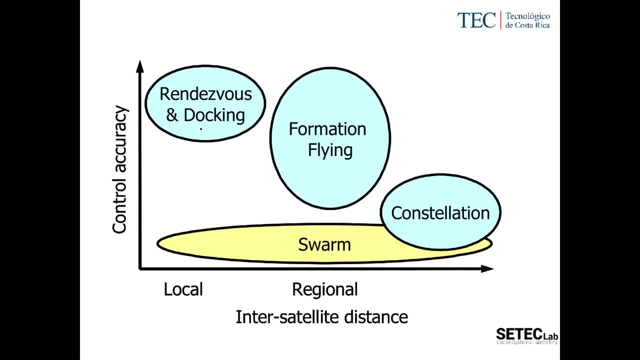 going forward and forward. Not one single satellite, but many satellites working together to accomplish a mission. Different kind of satellites are known as constellations, if the satellites are not necessarily working together, but they're just, you know, like one and each other. 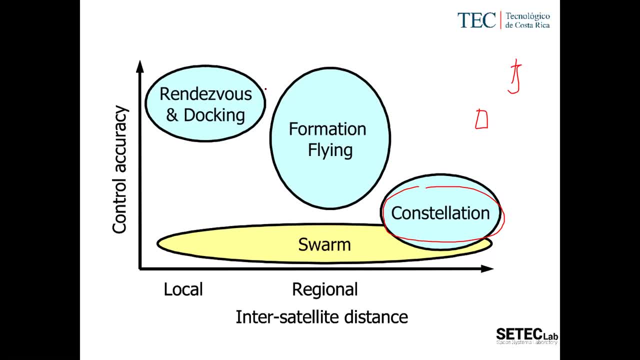 And formation flying requires more control accuracy, because the distance between one satellite and the other could be a requirement for the mission itself. Here in constellations, you don't need much control accuracy, which is this part, because really it doesn't matter what's the distance in these things? 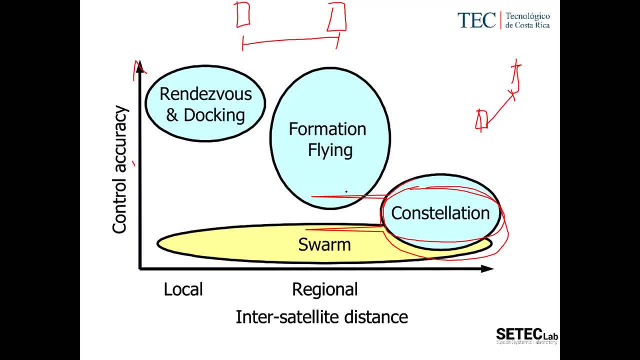 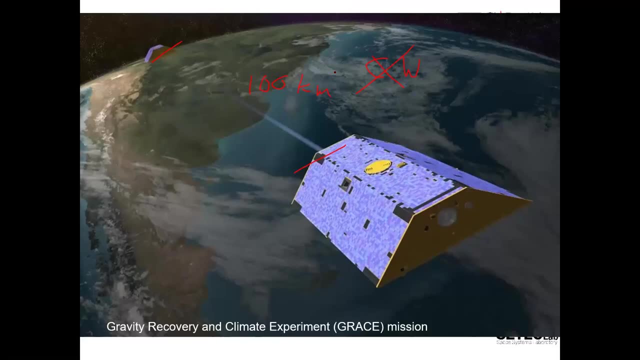 In formation flying. you might sorry about that. in formation flying you might have low requirements, but you might have very, very high requirements. Actually, I, I think I remember for GRACE that these requirements for estimation were in the matter of millimeters. 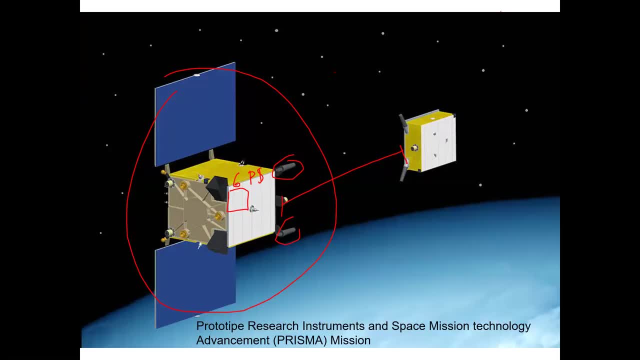 For example, the Star-Link constellation currently being built by SpaceX, currently being launched by SpaceX. These are satellites that communicate with each other using lasers. So we're talking about satellites that need millimeter precision and we need- we need all we can get on these kind of devices. So 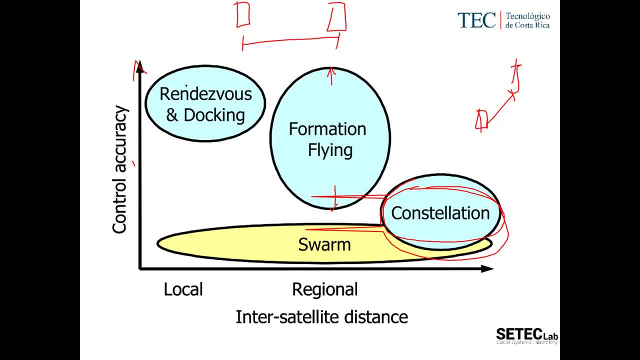 of course, in the Muandoki we'll always need control accuracy, but the difference is that this is very local In formation flying. we're talking about satellites with separations that could be in the matters of hundreds of thousands of kilometers. 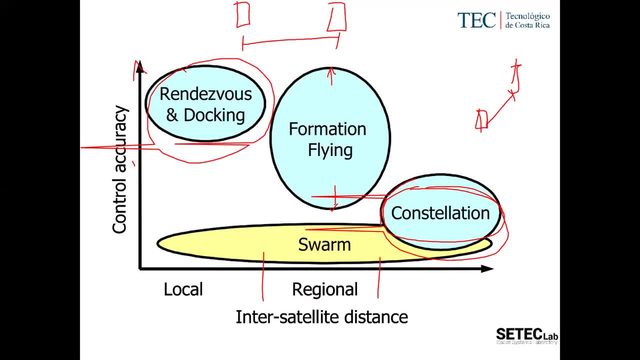 By the way, George is, it is usually you make the questions at the end, or you prefer to make the questions at any time. Whatever you prefer, I don't mind. Sorry, I had the mute on. Let's have all the questions at the end. 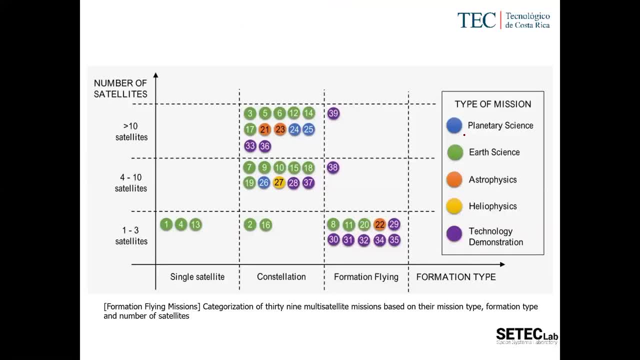 Okay, let's do that. Then. this is important. This is: this is the all these missions that I'm showing here, that these graphics are on my thesis. this is taken from away. these are all small spacecraft missions. I'm not talking about larger spacecraft. I'm talking about CubeSats, just as the ones that you're doing there in CubeTech. 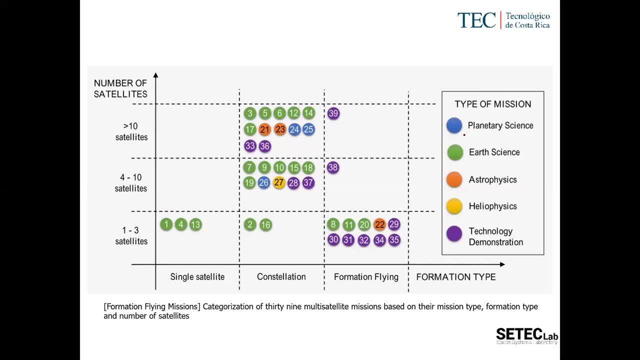 All these missions are requiring more than one satellite to be accomplished, and this is this is an image from 2015.. I mean, we're in 2020, probably this is three times more or so. I mean we're in 2020, probably this is three times more or so. 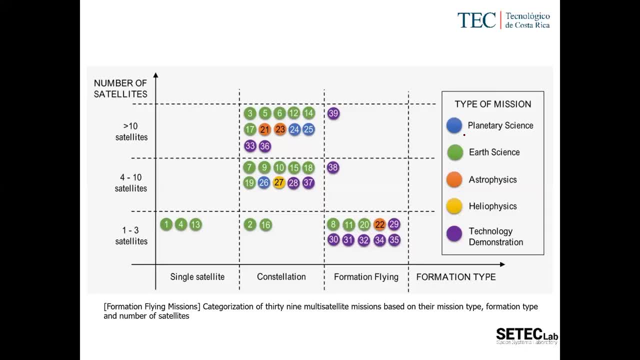 I mean, we're in 2020, probably this is three times more or so- And we're talking about a lot of missions, not only on constellations, but on formation flying. so we need this kind of better models for the relative dynamics. 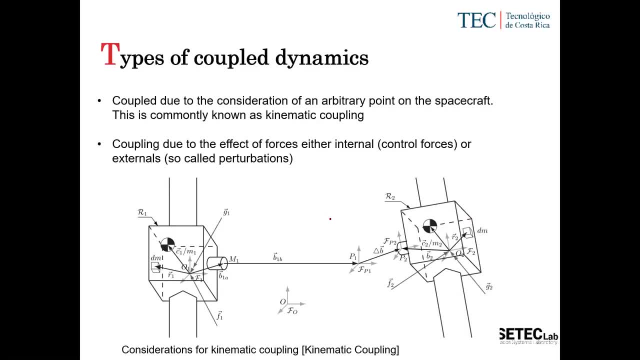 Okay then, I already talked about relative dynamics and the importance of relative dynamics in the present and future. Actually, most you know, a lot of innovative missions are formation flying. Then what I need to show you is that the consideration of coupled dynamics is important. 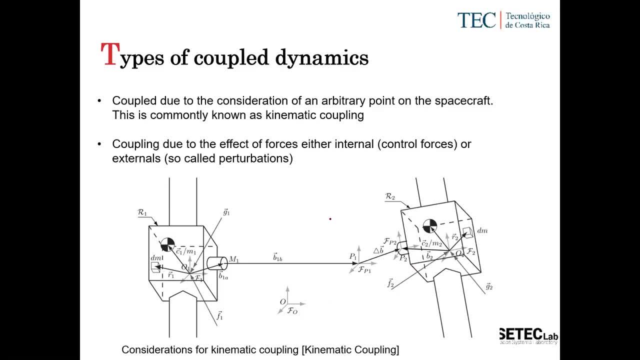 First I'm going to define what I'm talking about with coupled dynamics. There are two kinds of coupled dynamics considerations. The first kind is the one that some others know as kinematic coupling. Kinematic coupling is based on the fact that if you have the center of mass of the satellite, 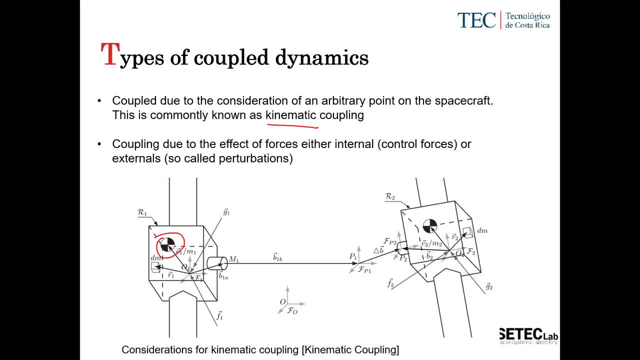 you usually describe the dynamics of the satellite using the center of mass. But if you don't use the center of mass but you use any other part of the satellite- any other part it doesn't matter- as a way to describe the attitude and orbital dynamics. 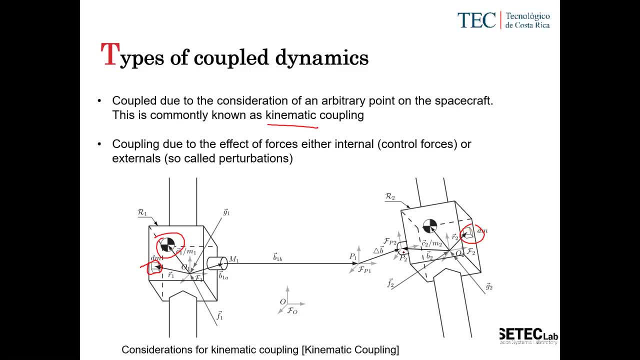 especially the relative attitude and orbital dynamics. then you will have couple dynamics. Why would you do that? Well, sometimes we don't have our camera exactly in the center of mass and we want to know the dynamics not only of the satellite but actually of these two cameras, because maybe this is not a camera, maybe this 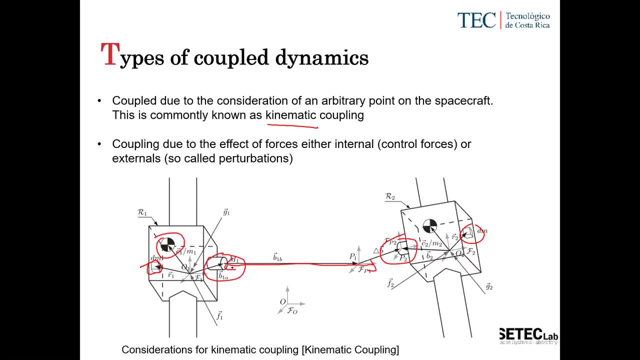 is the laser, and we need to know directly how these two parts are moving in order to have the better control and the better estimation at the end. This is known as kinetic coupling and it's not going to be the discussion of this talk When we talk about dynamic coupling. 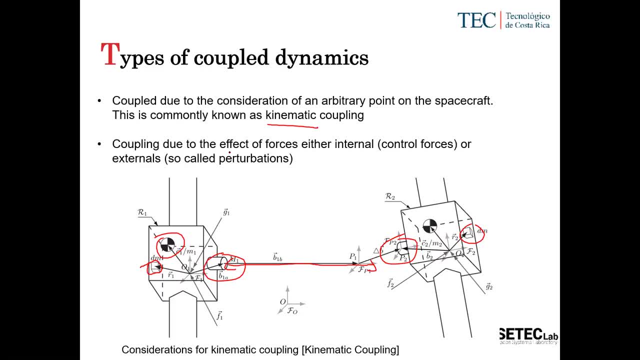 we're talking about the coupling that is due to the effects of force, either internal, meaning control forces, or external, the so-called perturbations. I say so-called perturbations because atmospheric drag might be used for control and is being used for control, and then if you're using it for control, you wouldn't call it. 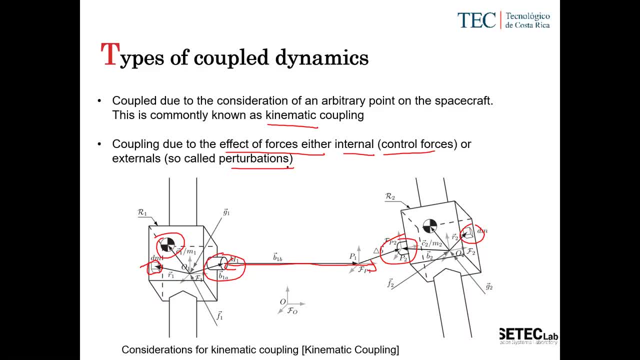 perturbation right. In the case of control forces, it means typically- and this is very normal- that you might have a control system that is not located in the center of mass and then the reaction of this control system not only moves, not only modifies the orbital dynamics of this. 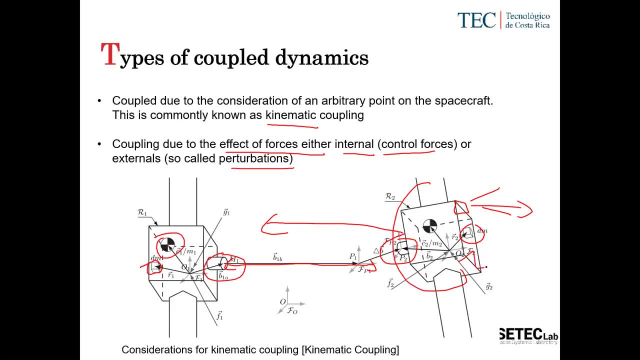 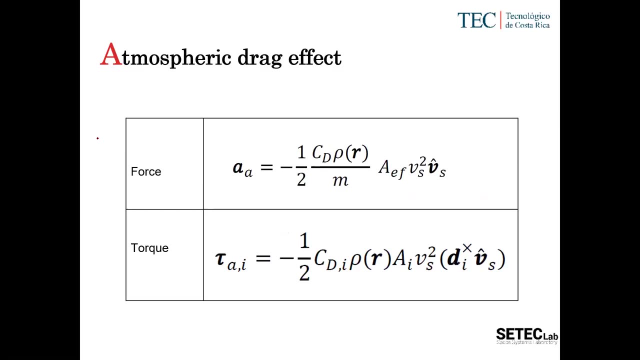 spacecraft, but also of the attitude dynamics of this spacecraft. That is, both, and we're going to talk in this lecture about dynamic coupling. Okay, then let's get to the mathematical matters a little bit. Most of the talk is going to relate to atmospheric drag effect. This atmospheric drag effect 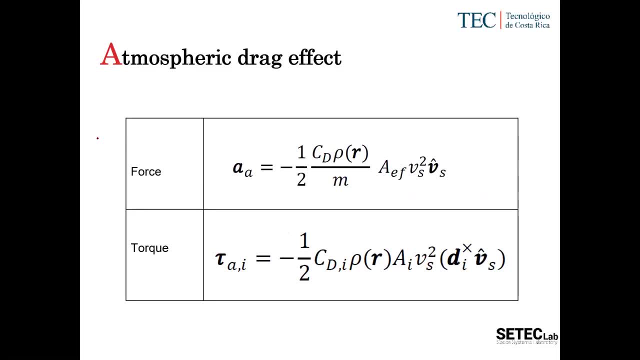 is usually very strong in a lower orbit. Here I'm talking about the atmospheric drag acceleration. As you see, the mass is here. If it was the force, then you would have the mass here, but it's not. Then here, the atmospheric drag force depends on the coefficient of drag. This is a constant. 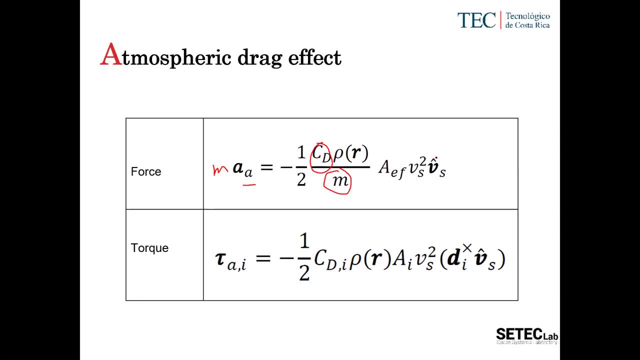 for different materials on the velocity of the spacecraft with respect to the atmosphere, And this is really important. The velocity of the spacecraft with respect to the atmosphere is not the velocity of the spacecraft itself, because you know, the atmosphere also moves. Then if a certain spacecraft is moving at a certain velocity, 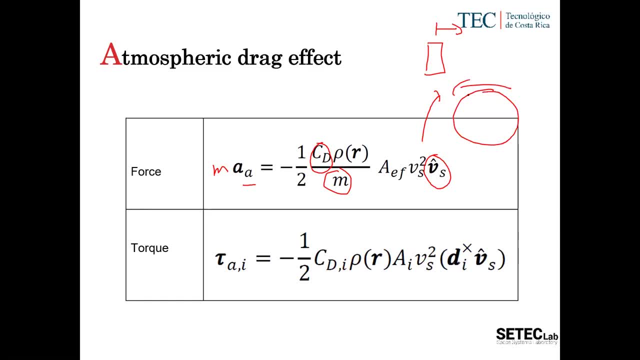 then the Earth is rotating in this way, then the atmosphere has a velocity with this kind of vector. But if you're moving in the other way, then the atmosphere has another velocity, Then this Vs will change, because this Vs is the velocity of the spacecraft minus the velocity of the 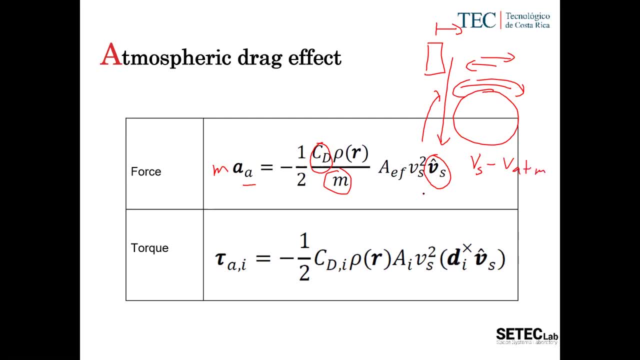 atmosphere. Okay, and this is important, Density: this is the density, and the density depends on the, on the position of the spacecraft. Here R is the position of the spacecraft, It's a vector, And this A is the effective area of the spacecraft. And here is where we 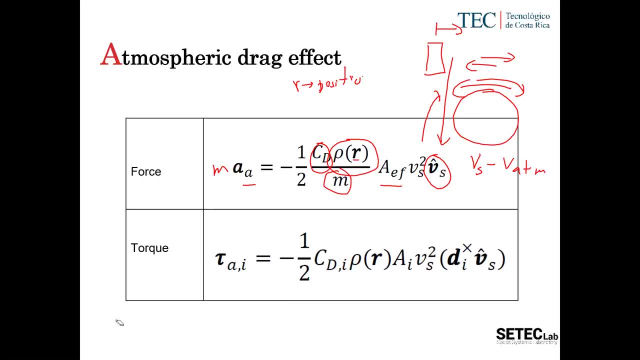 start with the fun part. Typically, the effective area of the spacecraft is considered to be. typically, this effective area is considered constant, But actually what my thesis was working about is that this effective area is not constant. The only satellite where this effective area is constant is 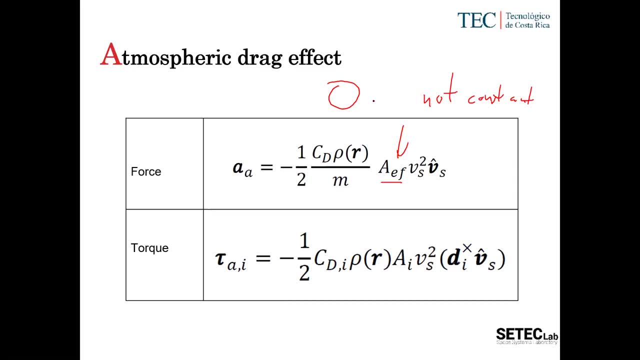 a circular satellite. If you don't have a circular satellite, then this effective area is not necessarily constant and could affect the amount of force. There is also the torque. Usually we don't consider the torque, But you see, the torque is an effect We have. this torque is in one side of the satellite Because 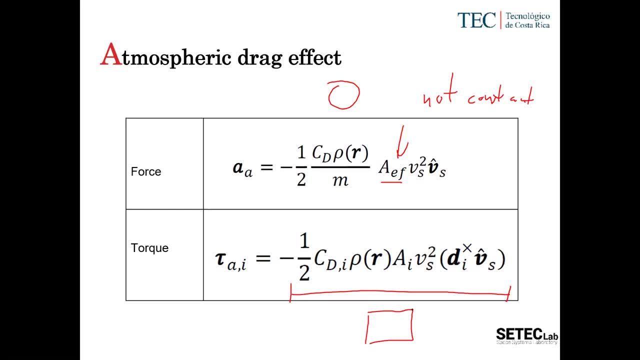 if we have a satellite with different sides, then there is a torque being applied here, another torque here and another torque here. So this equation is for one side. This is the coefficient of drag, This is the density of the atmosphere And, as you see, this density of the atmosphere, 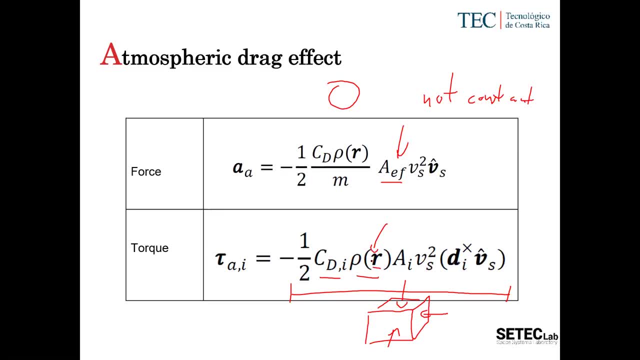 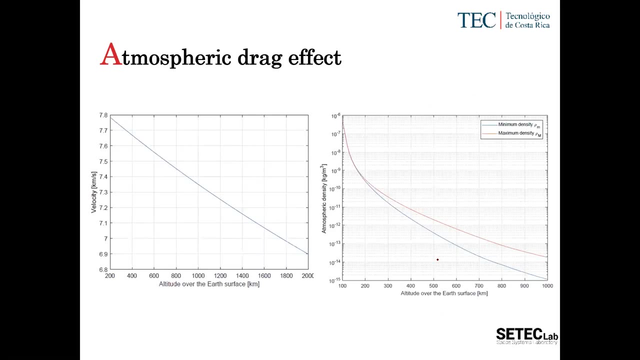 depends on the position. Already something in the attitude realm that depends on the position, This effective area, this is the velocity of the spacecraft, And this is the vector that we'll see soon. Then, what is important, before we talk about coupling itself? 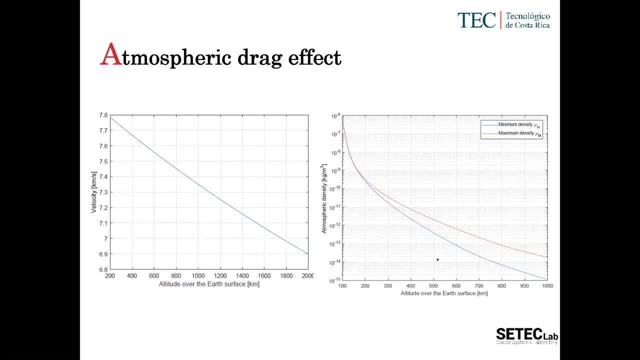 The atmospheric drag effect, as you saw, depends on the velocity of the spacecraft and the velocity on the atmosphere. So the amount of in low orbit, the velocity of the spacecraft ranks from 7.8 kilometers per second to 6.8, 6.9 kilometers per second, depending on the 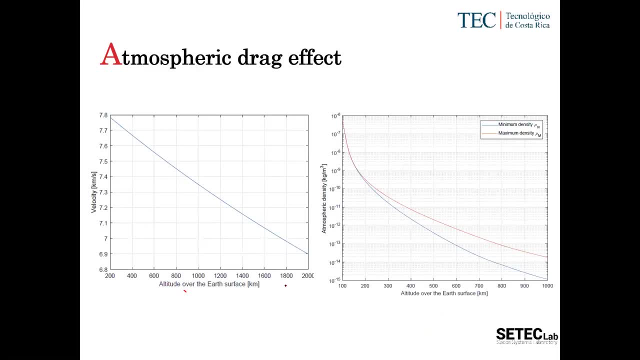 altitude over the air surface. This is for circular orbits And, sorry about that, this became a little crazy and I live completely in the city. Okay, I hope it's not too much noise Later. the other fact that we have here is the. 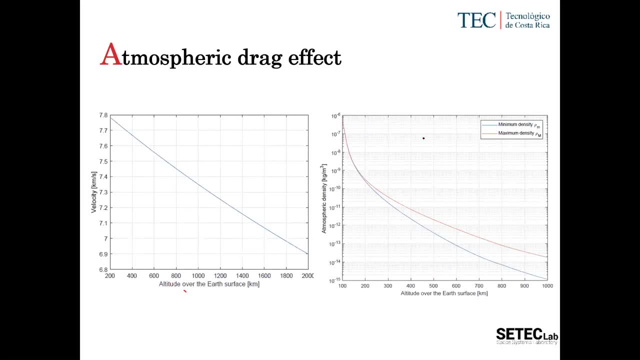 atmospheric density. This atmospheric density, it has a minimum. it has a maximum but ranks from 10 to the power of minus 6 to 10 to the power of the minus 14, for 700, 800 kilometers. Pretty much, basically. from here on, this consideration is no longer necessary. 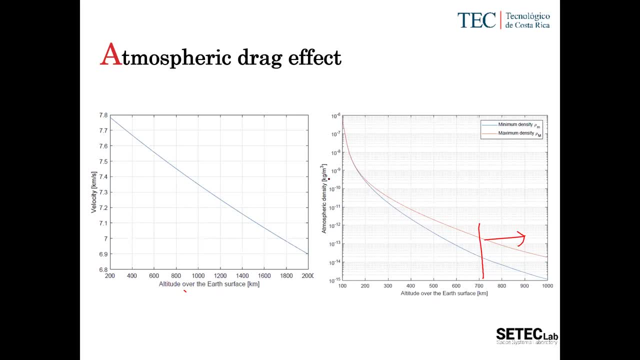 Adolfo. maybe we should stop a second for a moment, Adolfo. maybe we should stop a second for a moment, Adolfo. maybe we should stop a second for a moment. Does anyone have a question right now? Okay, if not continue. 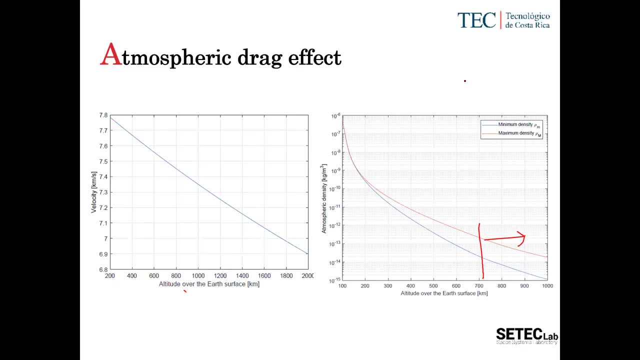 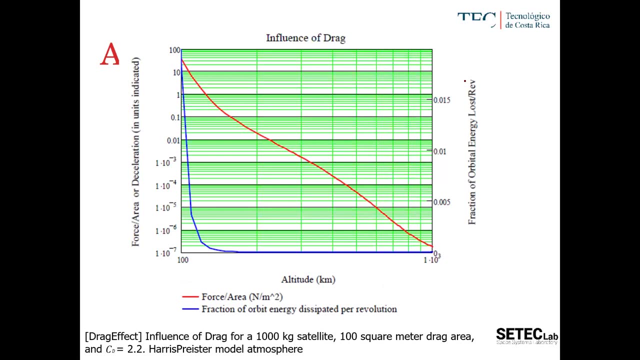 Okay, okay, I think I'll get to the part that will get all the questions. So I realize I'm taking more time than I expected. So here is an important fact: We lose one percent of the orbital energy due to drag when we are around 200 kilometers altitude. 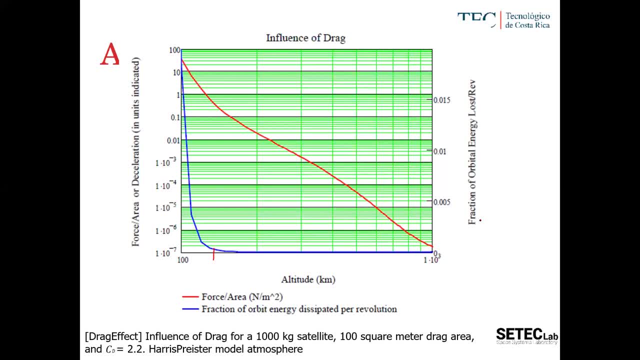 200, 300 kilometers, So this fraction of orbital energy lost per orbit. we're losing this kind of energy And of course if this is a constant loss then it doesn't matter. But really the loss of this energy in the orbital dynamics depends on the 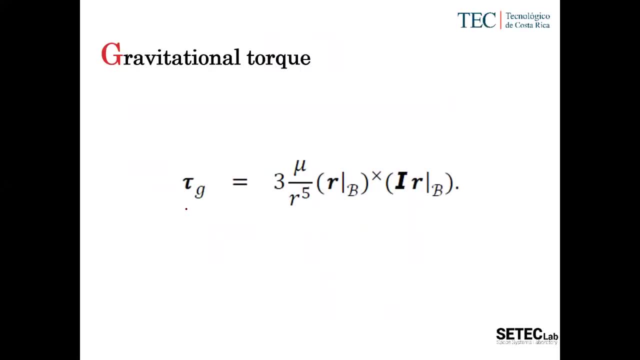 attitude of the system itself. So there are other sources of perturbations, like the gravitational torque that depends on the position of the spacecraft and depends on its inertia, But I'm just illustrating it here. It could be also analyzed, but this is not the case. 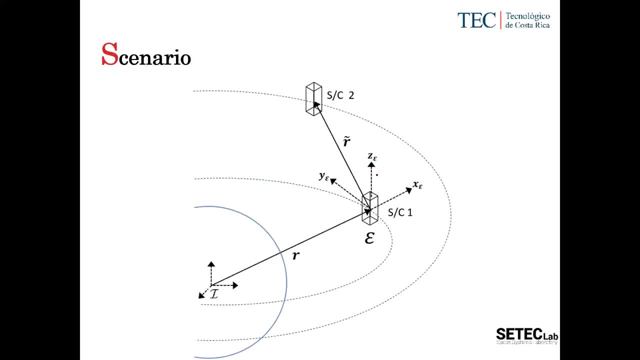 So, in order for us to check in my thesis, what was the effect? we started with two spacecraft. These two spacecraft, actually, this is the model of the systems, but the two spacecraft will be in 300 kilometers at the altitude, circular orbit. 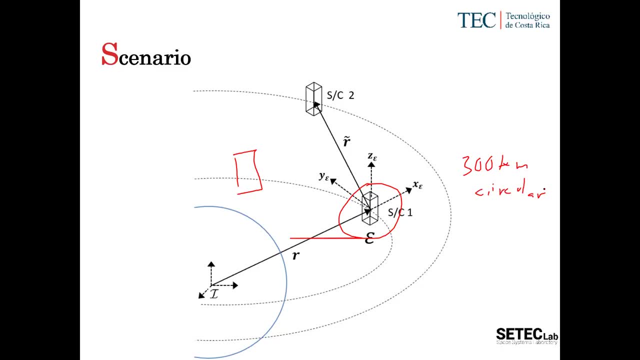 This circular orbit was selected, and this is equatorial. Equatorial orbit was selected in order for us not to take into account the stratosphere. If we take into account the stratosphere, we only take in to account atmosphere drag. then we don't have to relate to the obasto of Earth. So this is a very experimental. 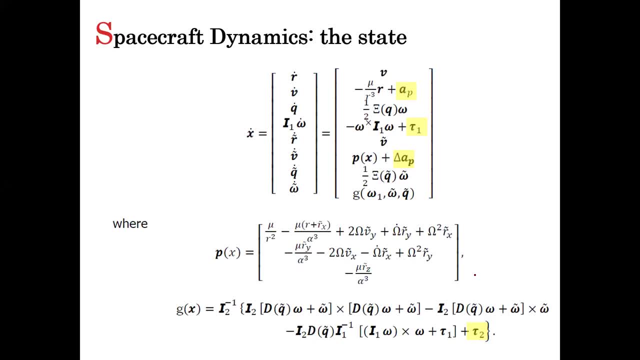 scenario And in this we get all the dynamics of the spacecraft. This is my dynamic model. This dynamic model has 20 states and I'm going to explain this very quickly. This is the position of a spacecraft in equatorial orbit. 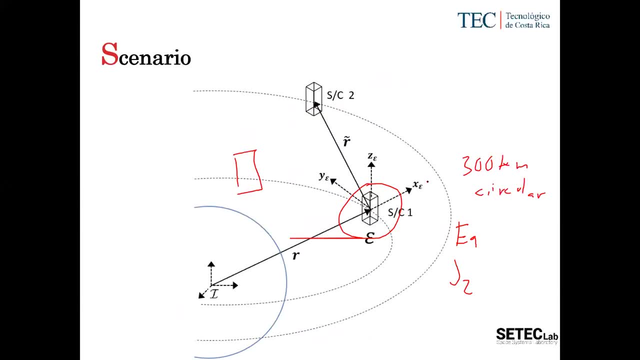 One spacecraft is considered a chief. This is the chief And this is the deputy. Okay, So the first spacecraft which is the chief. we have the absolute dynamics of this spacecraft. It's known, Okay, We know the orbital dynamics and the attitude dynamics. 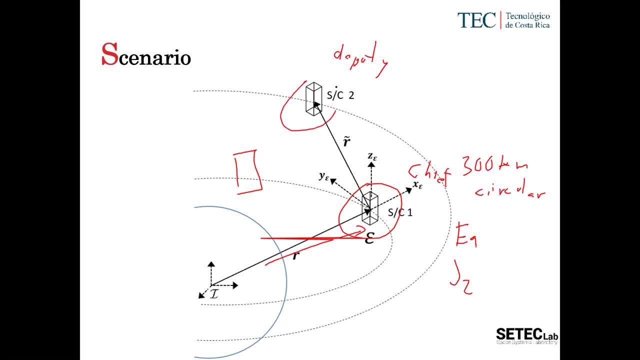 This second spacecraft is considered uncooperative. It doesn't have any sensors, It could be debris even, And we only know the relative position of the second spacecraft with respect to the first spacecraft. So this is the scenario we work on to test our theory. 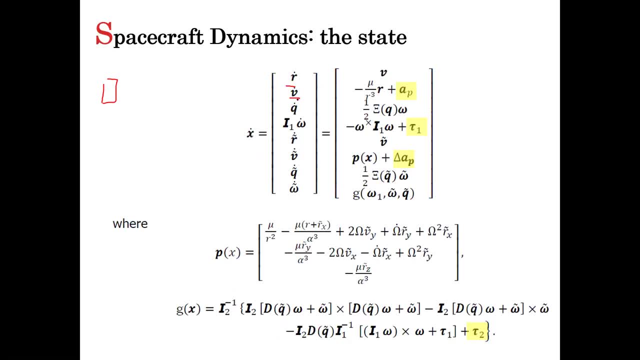 And then we have the position and velocity of the spacecraft. This is the attitude of the first spacecraft and this is the rotation rate of the first spacecraft And then the second spacecraft. we have relative position, relative velocity, relative attitude and relative rotation rate. 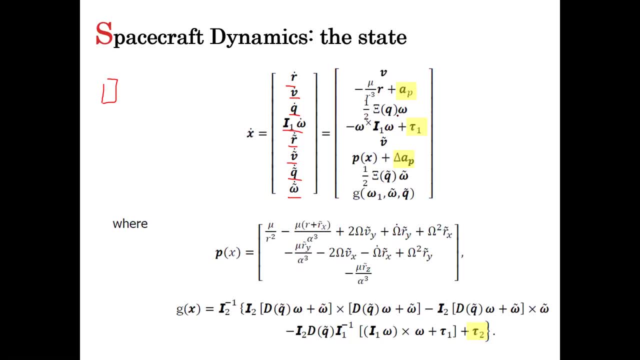 This is a complete mathematical model that is completely described on my thesis and probably most of these equations, especially the absolute attitude dynamics. you know them very well if you already were in an in an astrodynamics course. What is important? here I'm using quaternions for orbital dynamics. 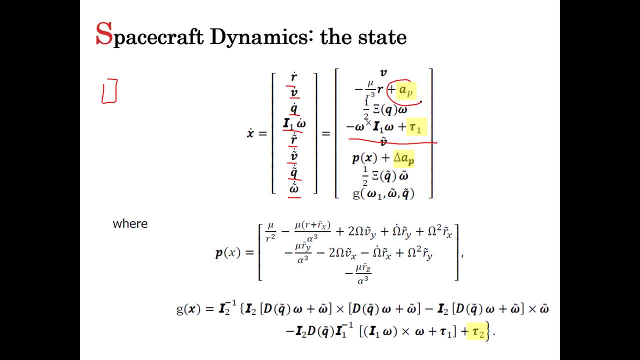 But the most important part is these kind of forces. This is the atmospheric drag force, gravitational force, torques and relative forces that I'm marking here. These are the source of coupling, Why? Because the effective areas of the spacecraft, the atmospheric drag, depends on the effective area for absolute and relative dynamics. 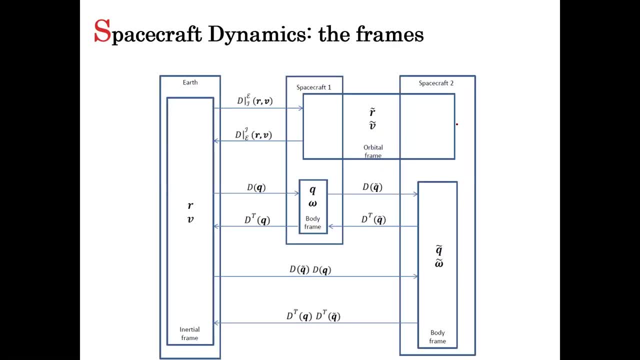 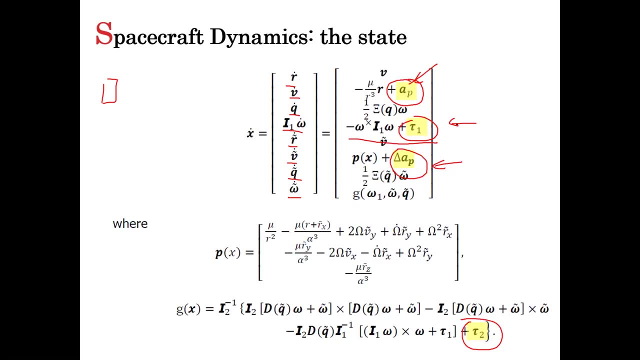 And the torque depends on the position of the spacecraft, And this is only an illustration. This, from the mathematical point of view, was a little bit difficult to manage because usually orbital dynamics are described for absolute dynamics in inertia frames. for relative dynamics they are described in orbital frames and usually attitude dynamics are described in body frames. 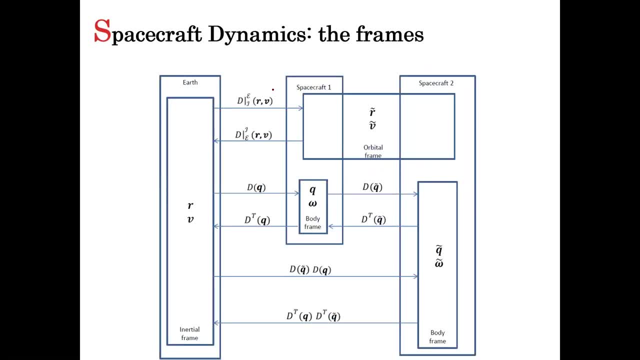 So these are all the frames that I use for this kind of research. We have the inertia frames for position and velocity of the first spacecraft, orbital frames for position and velocity of the second spacecraft, body frame of the first spacecraft for attitude and body frame of the second spacecraft for relative attitude. 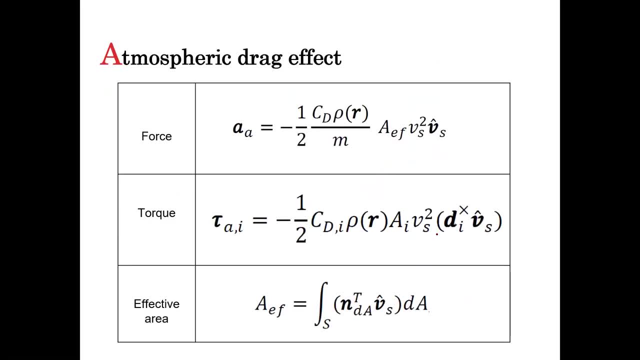 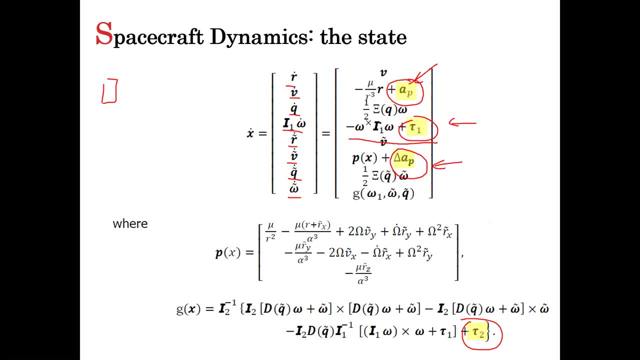 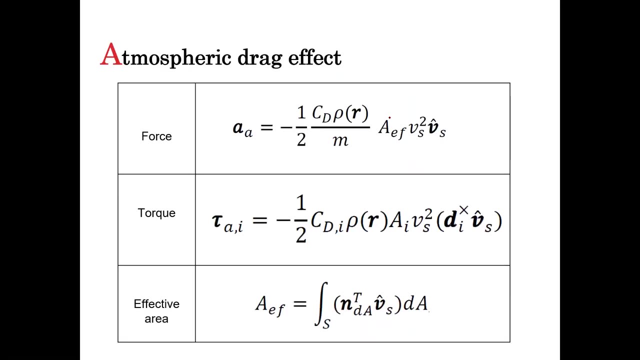 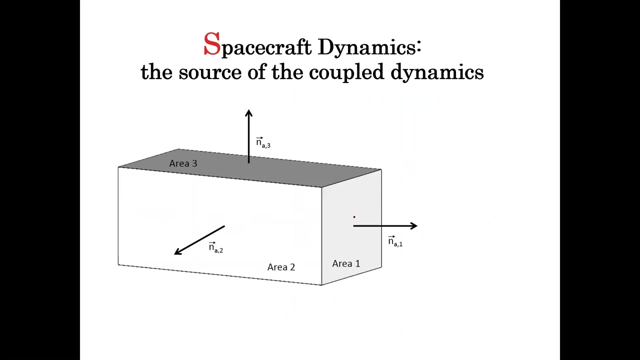 These all frames were used for this model and the atmospheric drag effect is described here as a coupling effect. So these yellow parts are the coupling effect. okay, This is what relates orbit and attitude dynamics And this is how it relates. Here we have the force depends on the effective area of the spacecraft and we have the torque depends on the effective area of the spacecraft and the effective area of the spacecraft. it's an integral, it's a surface integral and this surface integral, it depends on what the effect of the atmosphere is in every one of each area of the spacecraft. 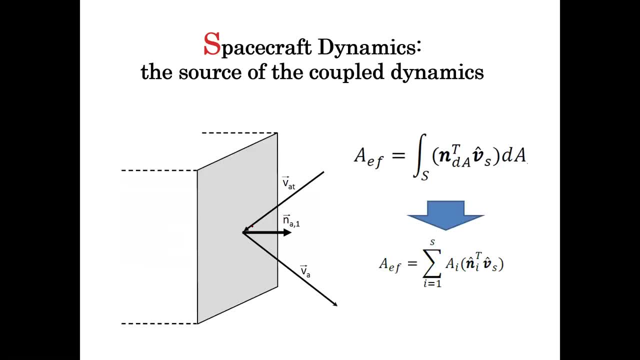 So how do I do that? I described the spacecraft as a series of areas. Then the effective area of the spacecraft is the area itself. you know areas could be described as vectors. So this n vector is the normal vector to the area, which has the magnitude of the area itself. 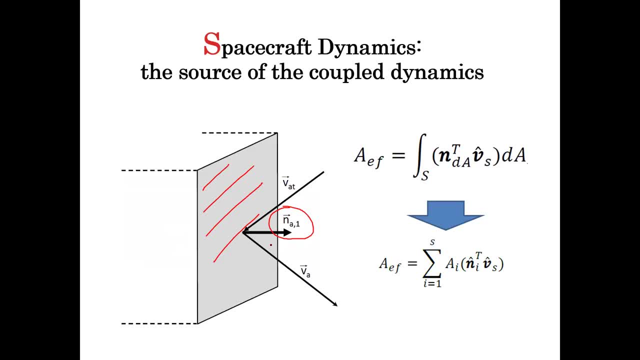 It has the direction. It has the direction out of the area itself. So we have the velocity of the atmosphere and we have the velocity of the area, And then the effective area of the spacecraft is the dot product between this vector and the vector, that is, the subtraction between VA and VAT. 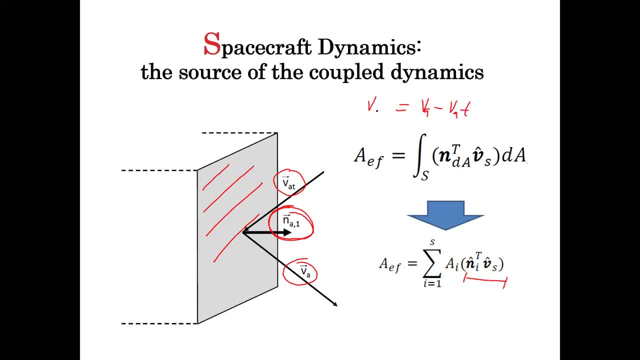 This is VS. So, in each one of the areas we make, we define the normal vector to the velocity of the surface with respect to the atmosphere, and we do this for every single area of the surface of the spacecraft In order, for every single time, we determine the effective area of the spacecraft. 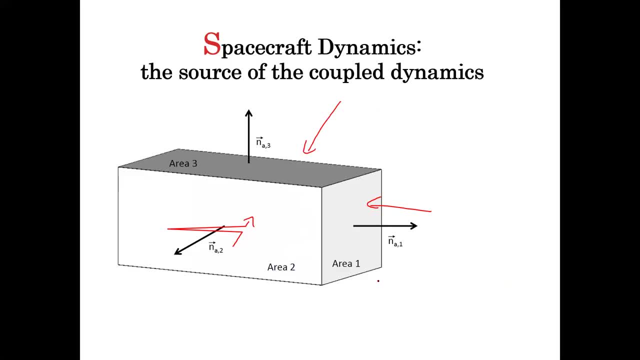 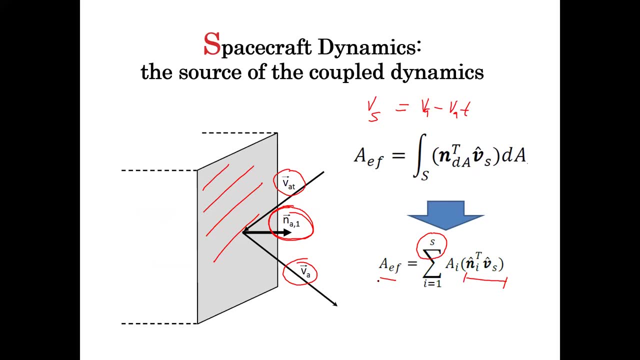 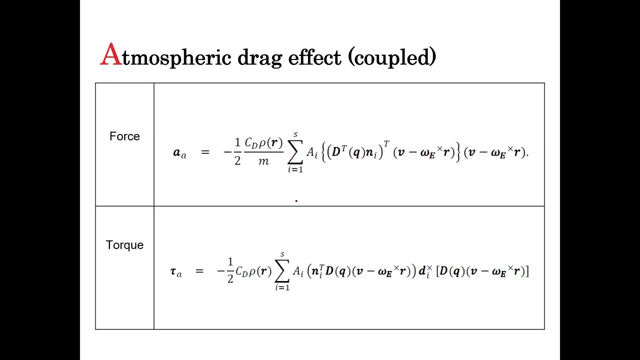 To know what is the effect of the atmospheric drag force and torque- And I'm only talking about the absolute dynamics of the spacecraft. This is only absolute dynamics. This is the model of the force and the torque, of the absolute, of these absolute dynamics of the spacecraft coupled 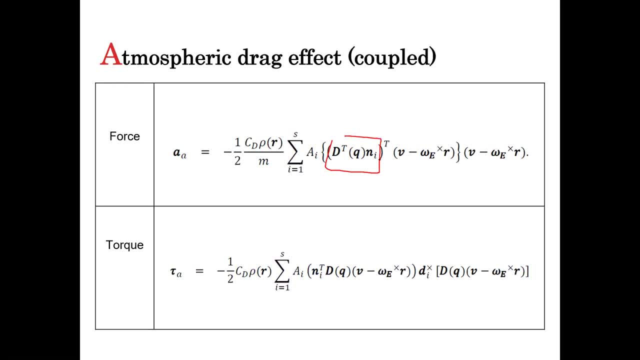 This. this is described because this n vector is described in the body frame. We have to rotate it to get it to the inertia frame. Adolfo, Adolfo, Yes, Right now do you have a question? Hello, I do. 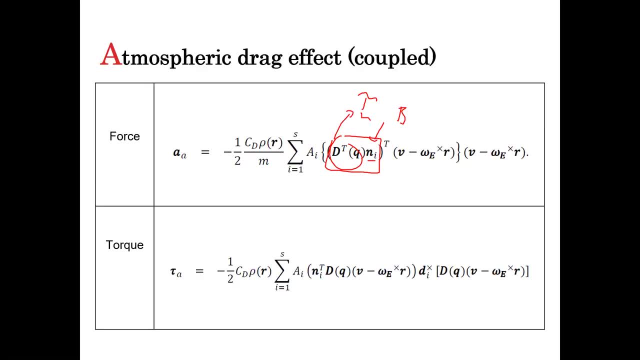 Hello, Professor Maeda and Adolfo. Yes, First of all, thank you for letting me participate in this lecture, And my question relates to the calculation of the of the resulting vectors, due to the fact that the atmosphere velocity- I think it's not constant, right? 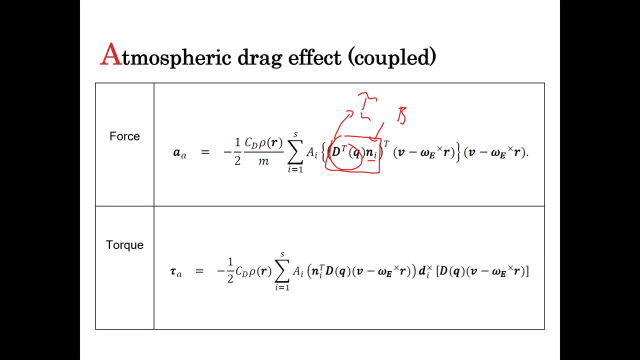 It changes a lot depending on position and the angle of the orbit the spacecraft is in that moment. So how do you model it to be able to compute every, every other part of the vector when you use it to calculate? I think that's a lovely question. 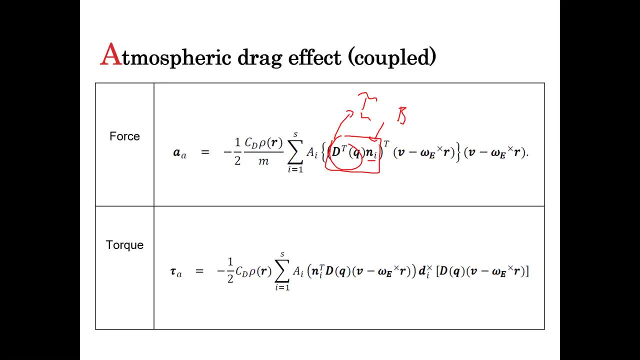 Actually it's a very, very good question, The short. I have a short and long answer. The short answer is that we assume in our models that the atmosphere is co-rotating with Earth. So the atmosphere is, the Earth rotates and the atmosphere co-rotates with Earth. 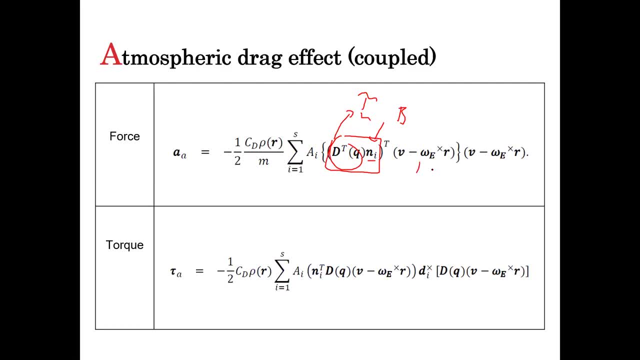 Actually, here in the model, this is the velocity of the atmosphere And this is the velocity of rotation of the Earth And this is the radius. So this is, this is the velocity of the atmosphere. This is a description on the atmosphere co-rotating with Earth. 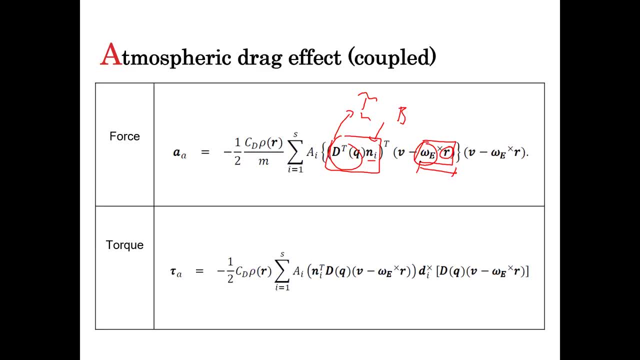 Of course, this model is not perfect. That I give you. But it's better than not taking it into account at all. So it's still not perfect- It would be impossible for it to be perfect because it's not deterministic- But it's way better, way better than not taking it into account. 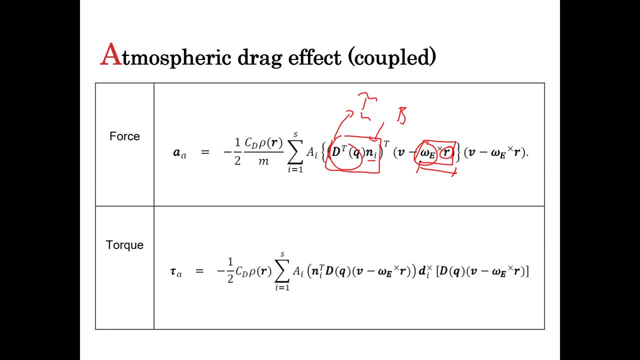 And the better we are, the better our estimation is. I don't know if that answers your question. Yes, it answers it very, very good. Thank you Because? yes, because I was wondering, because you have to have a compromise right. 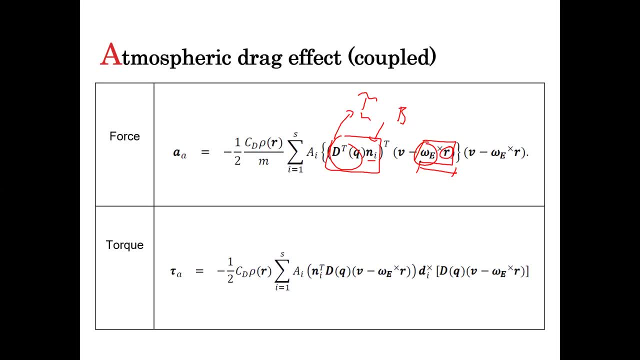 Between the calculation and the computational power to generate it. So I think it's a really good approach. Thank you for answering. Actually, it gets me to another part. I really think we could estimate density itself, And I think one of the future results of this kind of research is actually 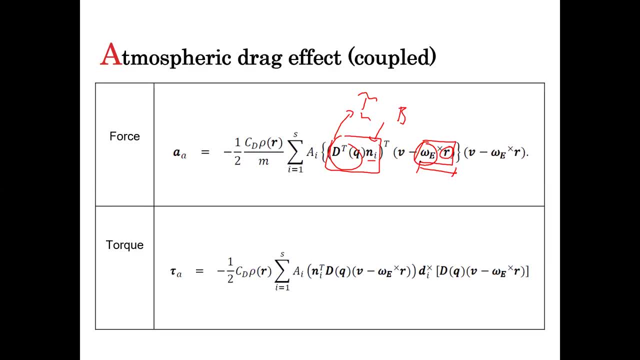 is a satellite that doesn't assume that you know the density itself, but actually calculates it. It's part of the estimation itself. We don't do it, but I think it should be feasible. All right, Very, very good question, Thank you. 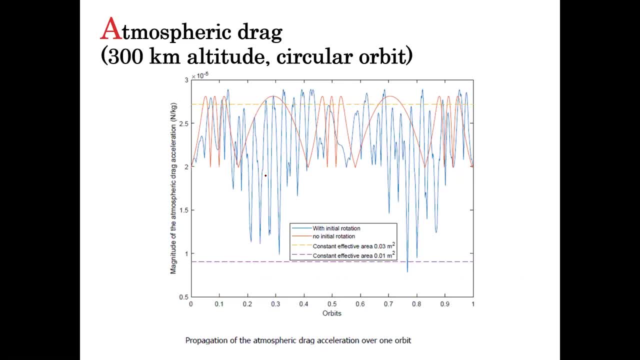 This is first, one of the first results that I wanted to show you. So you might think: why would you do all these complications? Is it really necessary? I mean, why don't we just say: well, you know, we have an effective area. 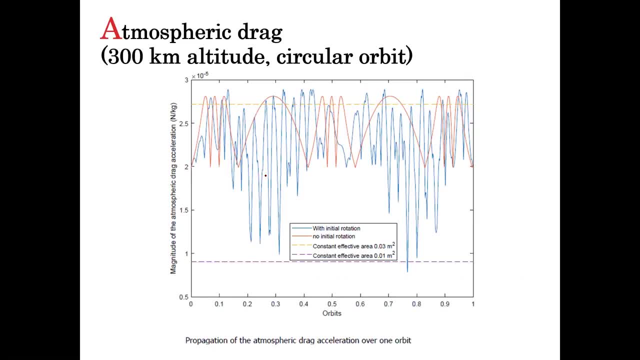 and this is the effective area. we calculate it and this is more or less okay. But in these graphics I show you what are the magnitude of atmospheric acceleration if we have an inertial rotation on the star. So if we have an inertial rotation on the spacecraft which is the blue, 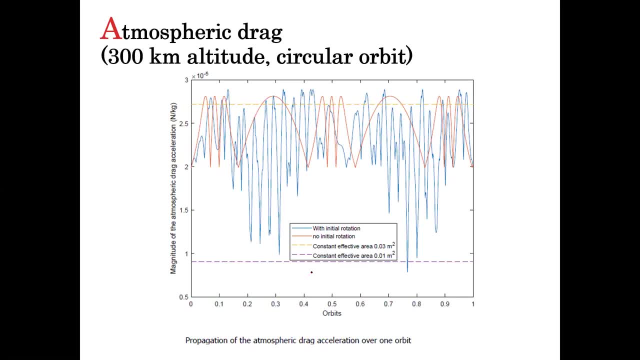 what would be the magnitude of atmospheric drag acceleration if we don't have an initial rotation? Okay, So what I want you to see is that any way the spacecraft, if it doesn't have control, it will rotate. But there are a lot of differences between this graphic in orange. 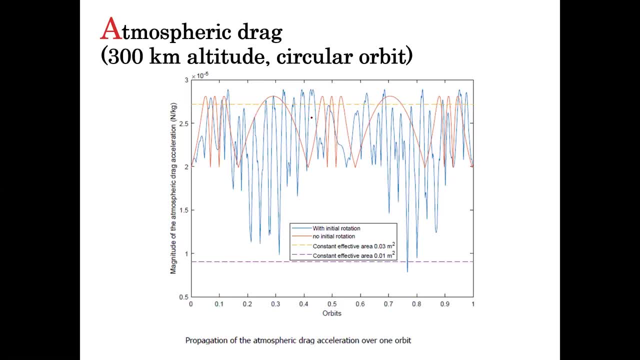 and this graphic in blue, This yellow graphic, is what will happen. I'm taking this into account. I'm using CubeSat, three-unit CubeSat. So this is 30 by 10 by 10.. So this is 30 centimeters, and this is 10, and this is 10.. 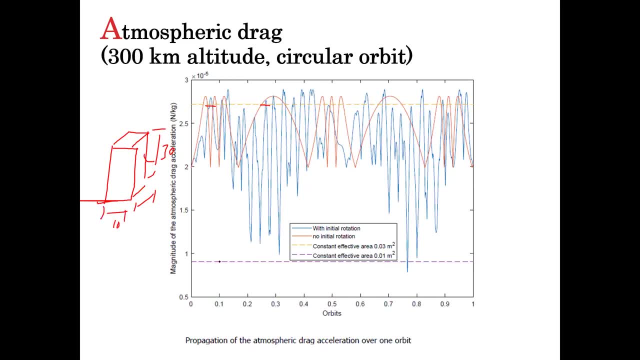 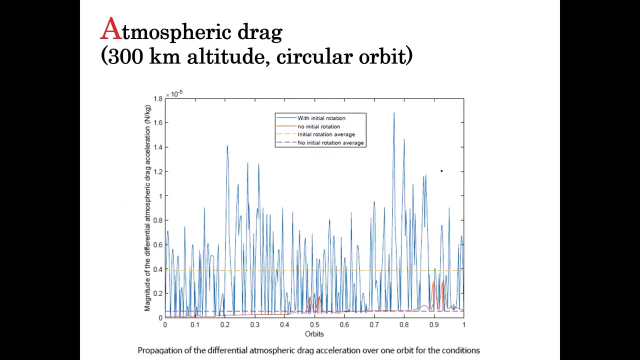 Okay, Then this would be the magnitude of the effective area if we take into account this area as the effective area. This is the magnitude of the effective area if we take into account this area, the long area, And these are all the dynamics differences if we're rotating or not rotating. 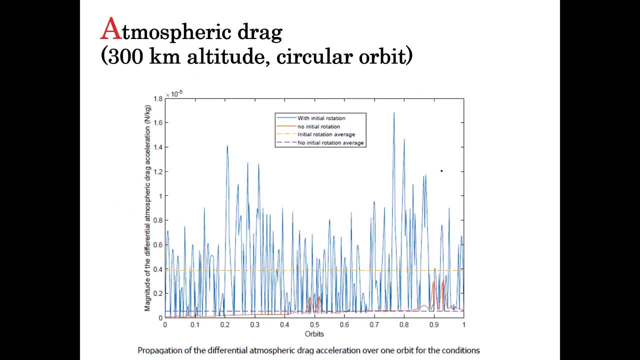 And this is important- The propagation of the atmospheric drag acceleration for one orbit is only one orbit. So if we have an initial rotation, this is the case of blue, and we don't have an initial rotation, this is the case of orange. 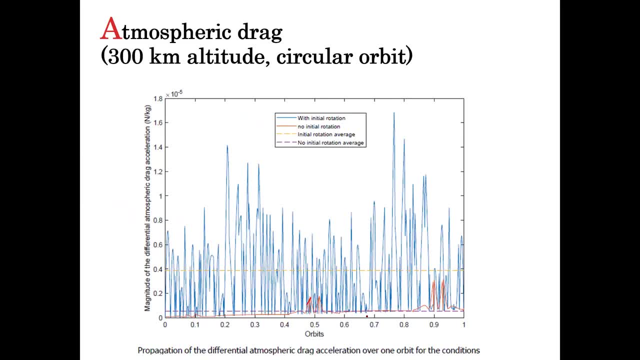 And the average of each one of them. we're talking about the exact same spacecraft. We're talking about the exact same spacecraft, but in one of the cases we are rotating and in one of the other cases we are not rotating. 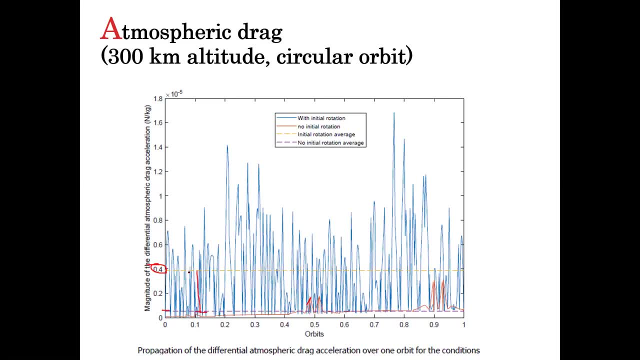 The average changes a lot due to the dynamic effect of the spacecraft itself, And this is a difference in force that we're not taking into our models of estimation, And this is important for this kind of cases. We're talking about the 300 kilometers altitude with circular orbit. 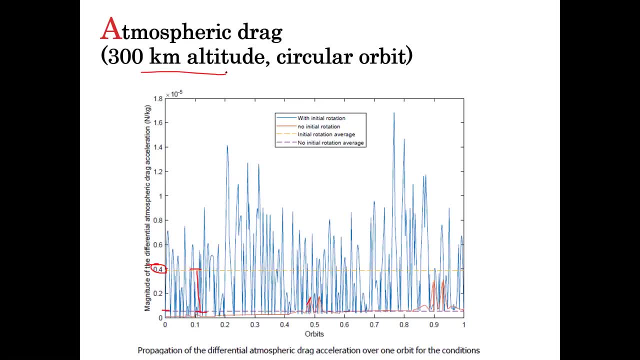 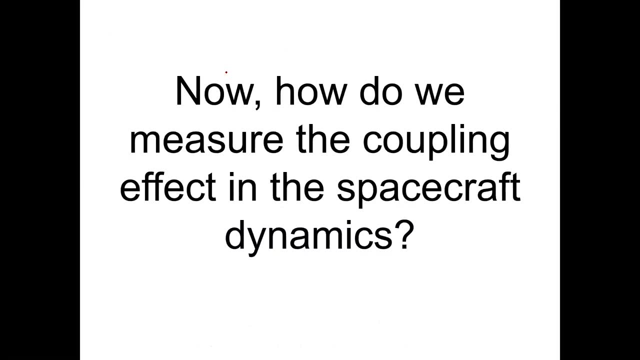 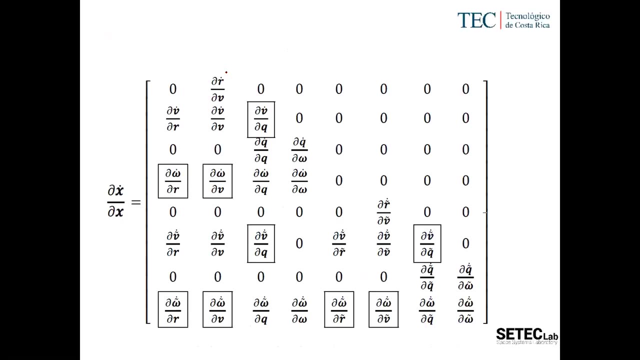 And yeah, okay, fine, We get this. It is important, It is a force, It could influence, estimation and control. But how do we measure the coupling effect? What we did in our research was that we get the gradient of the state itself. 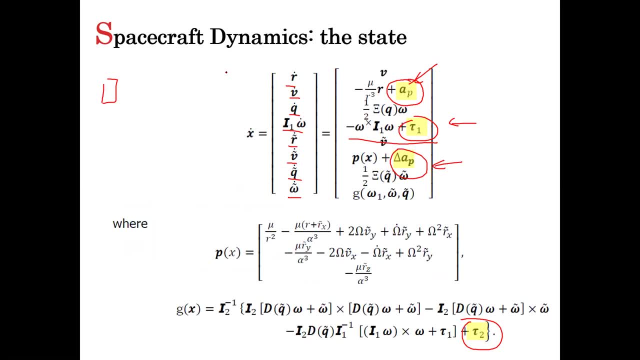 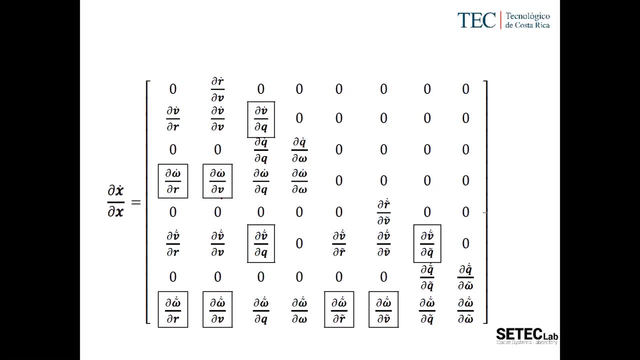 which is: this is the state, this is the complete state. So we get the partial derivatives of each one of the states with respect to itself. So, for example, all this is the partial derivative of the position with respect to velocity, partial velocity with respect to velocity, etc. etc. 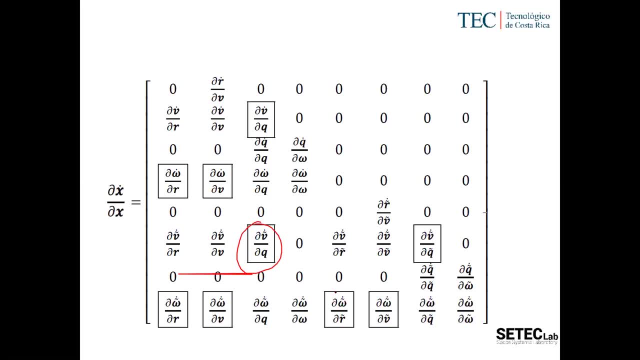 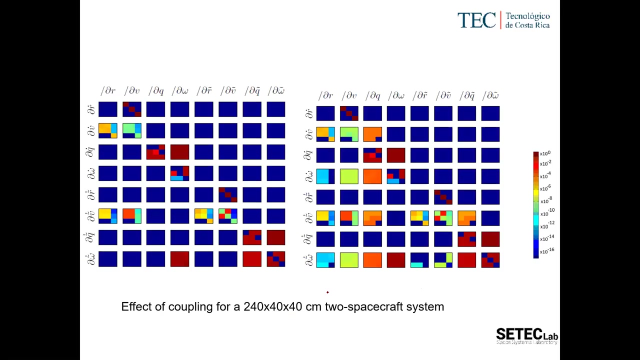 All these that are in a square are related to coupling. For example, this is the variation of the rotation rate of the relative spacecraft with respect to position, things like that. So all of them are related to coupling. And then I created this kind of radiography, these heat maps. 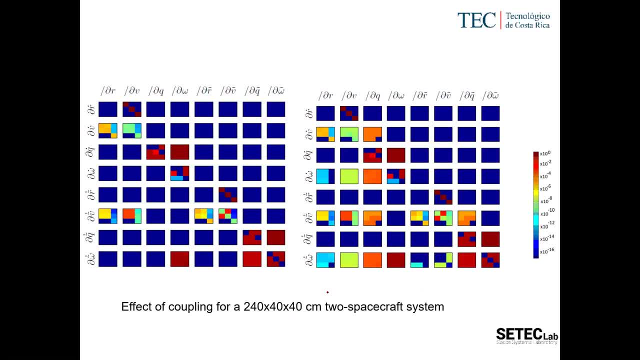 where we see what happens with these partial derivatives, when we take into account coupling and when we don't take into account coupling. When we don't take into account coupling, of course they don't exist. They are zero. But in these places we have these elements. 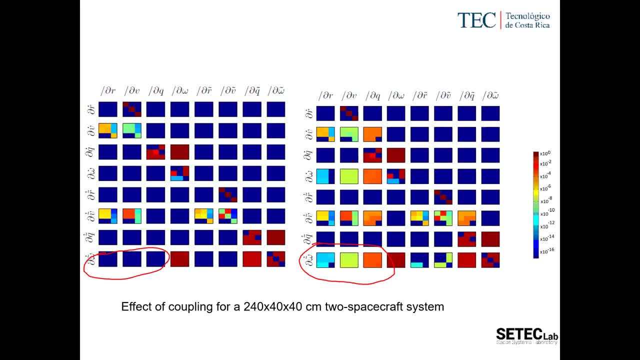 And these elements are related to coupling. These elements here are related to coupling, These elements here are related to coupling And many other elements here are related to coupling. What is important, What is interesting about this? Well, the gradient itself is a measurement of observability. 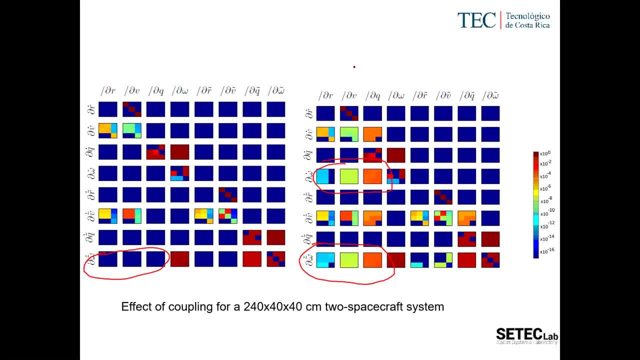 For any one of you- I guess everybody who has taken a control systems course you know observability is how much can we read the states of a system? And these elements add observability to the system itself, And this is the important part. 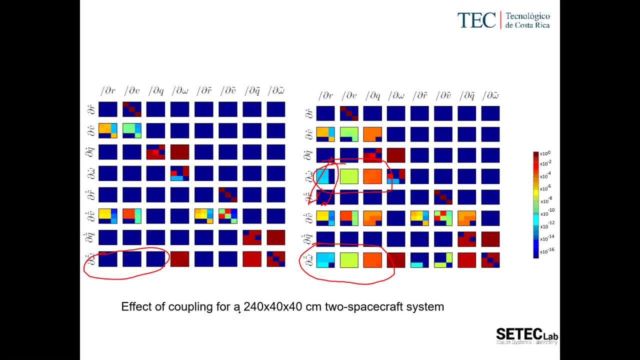 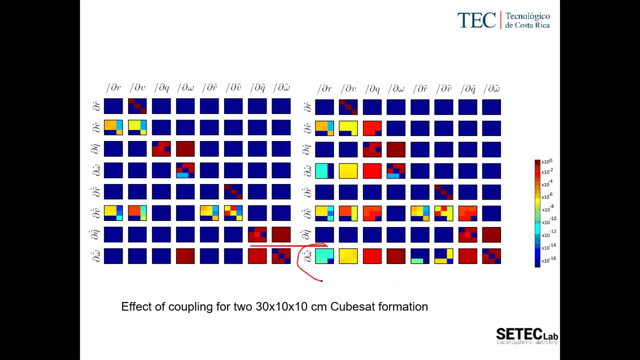 So this is the coupling for a 240 by 40 by 40 centimeters spacecraft to a spacecraft system And you will say, yeah, okay, this spacecraft is large enough. Well, this is the case for CubeSats. In CubeSats, we still get these elements, these coupling elements. 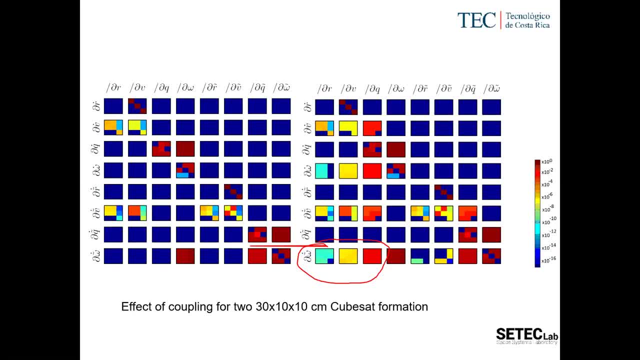 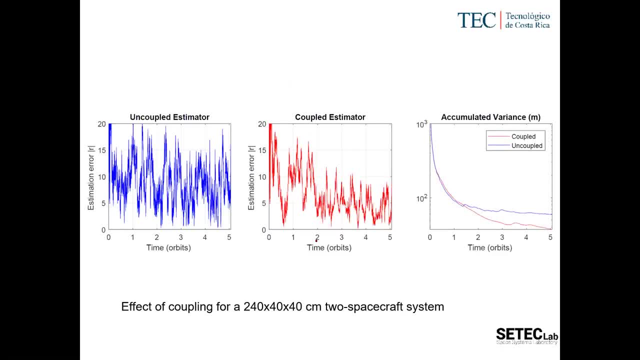 And this is a radiography of the coupling elements. And you might say, okay, fine, it exists. Of course it exists, But how is this important? Well, in my second research, we created a Kalman filter, one that didn't take into account the coupling. 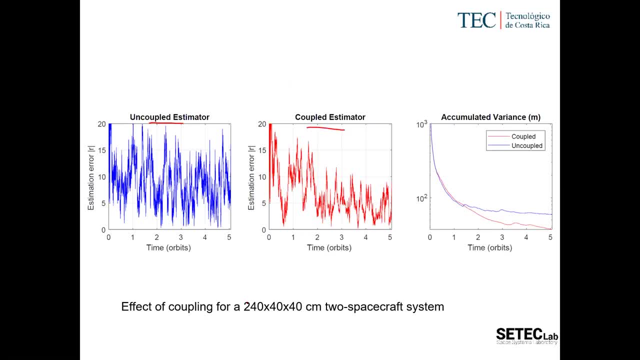 and one that took into account coupling. This is for the largest spacecraft, or five orbits, And this is the estimation error in meters. This is the average of, of course, is the absolute value of r. I'm talking about the one spacecraft and the second spacecraft. 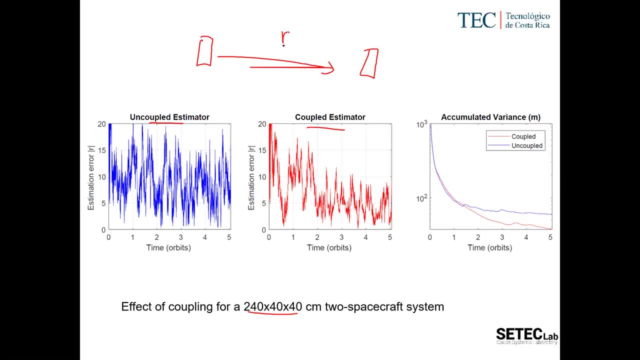 And the relative position of these two spacecraft is known as r, like this, And what we get here is the absolute value of this part. So, as you might see, this coupled estimator had better stability and it has an accumulated variance very low with respect to the uncoupled estimator. 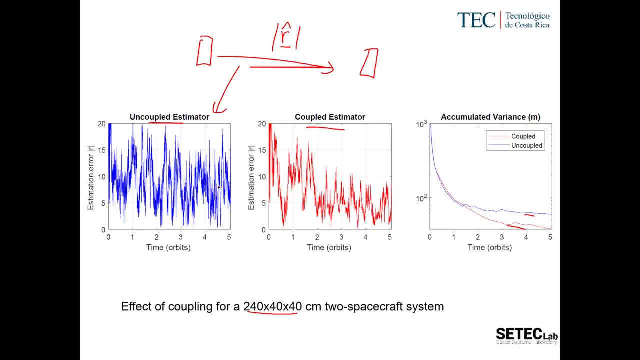 The funny part about the uncoupled estimator is that we actually try using- not using- the dynamic model couple, but we- and this actually took me weeks- we tried to synchronize this uncoupled estimator to be the best possible uncoupled estimator. 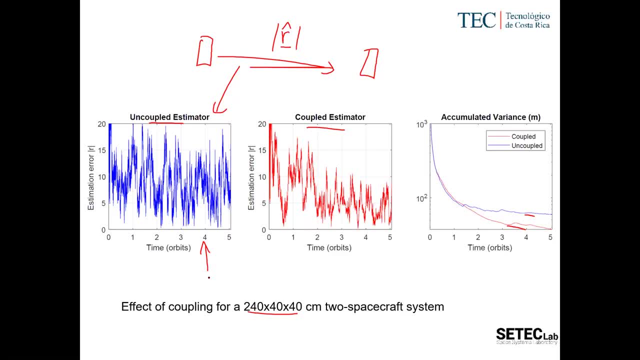 This is described on my thesis But, yeah, we took the work to actually have the best uncoupled estimator possible, trying to noise model itself, And this is the case for a larger spacecraft And this is the case for CubeSats. 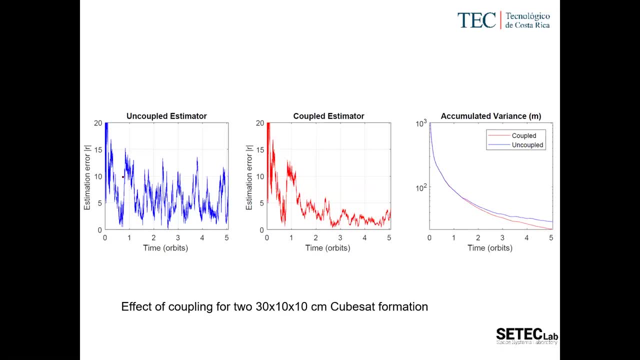 As you might see, the uncoupled estimator had this between 15 and 5 estimator error, but the estimation error for this spacecraft is way lower. We're talking about CubeSats. I mean, what am I saying here? I'm saying that with the same hardware. 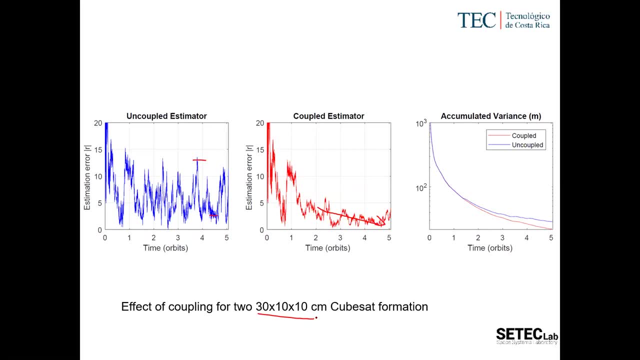 with absolute, absolutely the same hardware for relative dynamics. you can improve the estimation results for CubeSats with only improving your dynamic model, And these are the results that we published in the second journal paper. This is the variance of the error depending on the area itself. 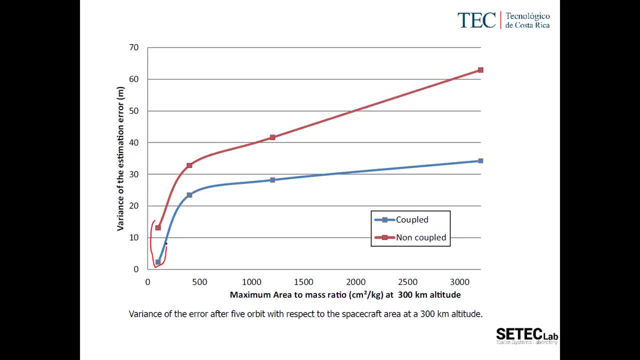 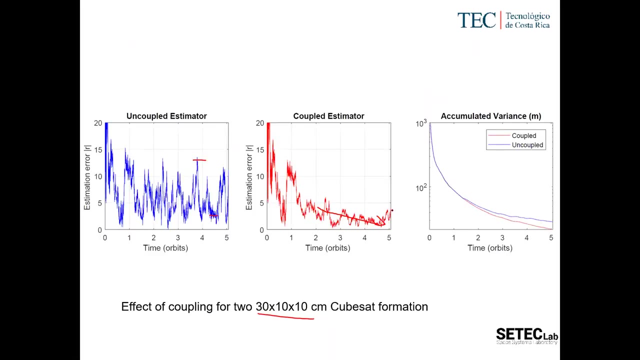 So for small areas we get the couple to be better than the uncoupled, But for larger areas, of course, this result is even larger. This is the variance of the error. I mean this error. this is the variance of the error. 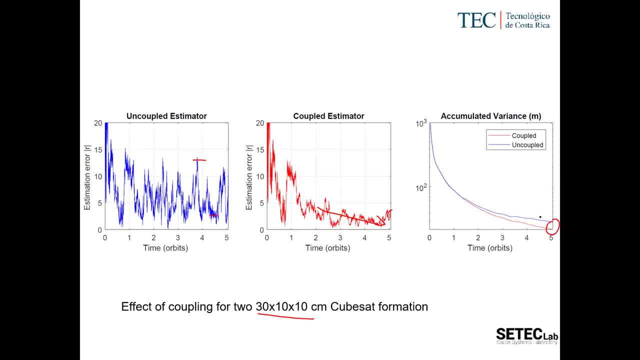 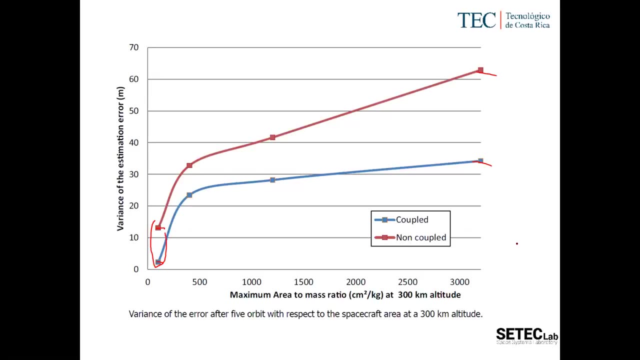 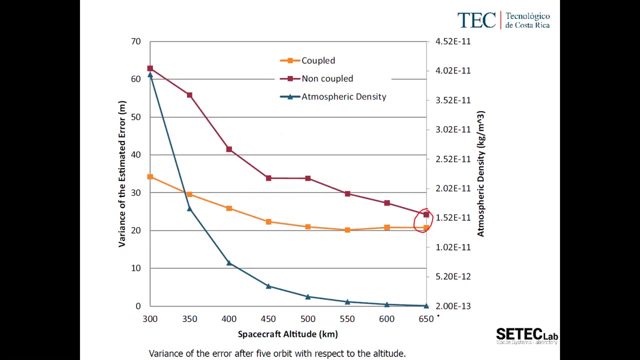 So after five orbits we have a variance of the couple and the uncoupled And this value here we tested for different spacecraft altitudes And we see that after 650 kilometers about the Earth's surface this is almost the same. 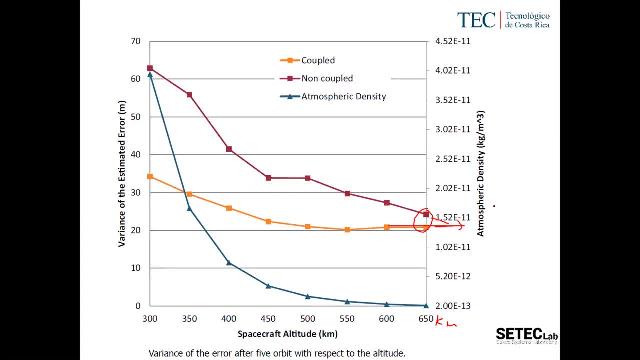 So our conclusion is that for the scenario that we selected, after 700 kilometers about the Earth's surface, this doesn't give us much of a good result. But for, say, 300, 400 kilometers, the couple estimator is way better than the uncoupled estimator. 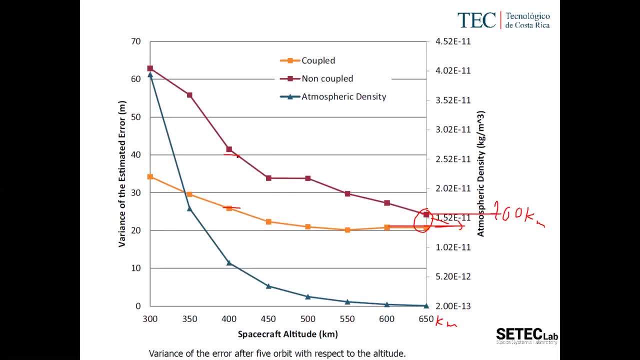 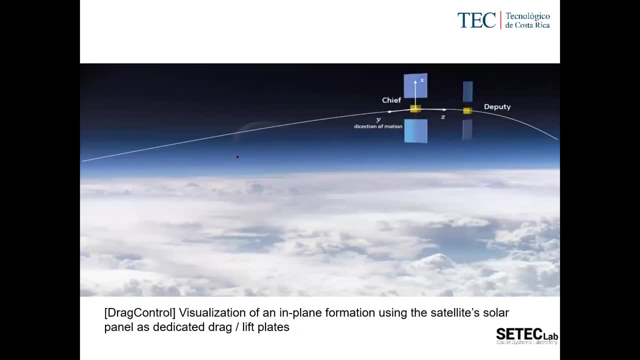 And this is about estimation. I talk about estimation a lot, But of course, many of you might be interested in coupled control. I can tell you what's happening with coupled control. There are many experiments already and this was started by the University of Toronto in 2014,. 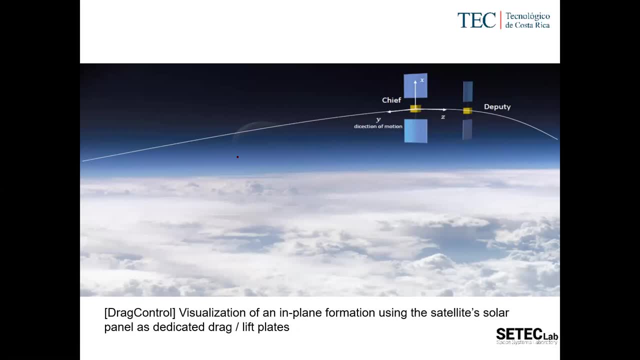 where they change the effective area of the spacecraft by moving the solar panels to control the distance between a chief and a deputy. But they work in kind of a 1-0 kind of configuration where we have, say, for example, one solar panel like this and one solar panel like this. 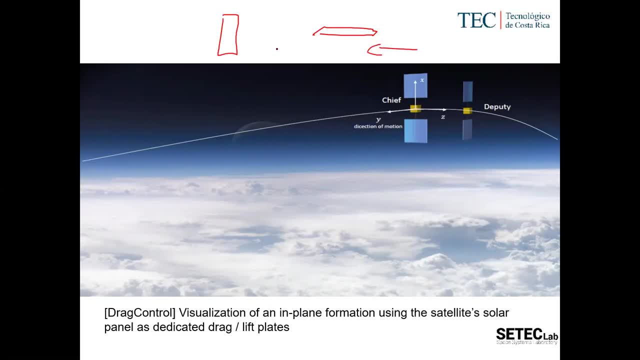 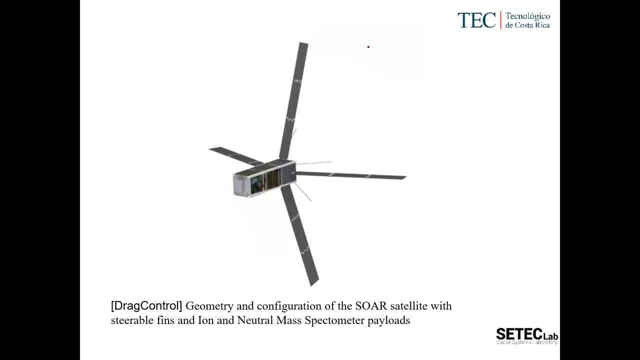 if the velocity is like this, Because one has to chase the other one, or one has to be farther away or closer away, And this is a use of coupling dynamics for control purposes, And this I found actually one of these days that I was doing. 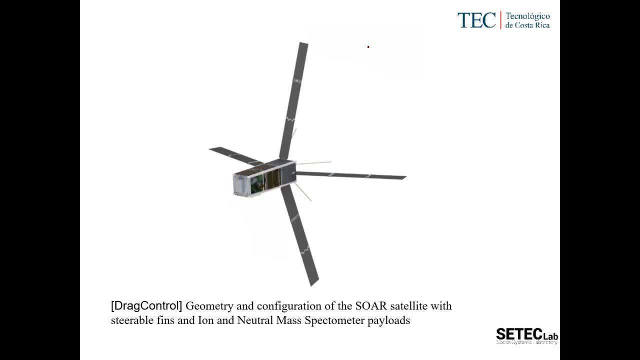 I mean, I presented this thesis this year, but of course this is a hot, hot topic And I was researching- and this is a proposal by the University of Manchester- of a CubeSat that is designed to actually take into account this coupling effect. 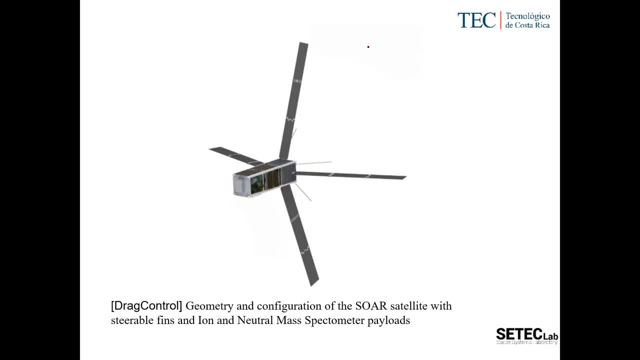 And it is designed a little bit dynamically. I would say This is not launched, This is from a paper in 2020, this year, But, as you see, we have a very big opportunity in showing control and estimation systems with CubeSats. 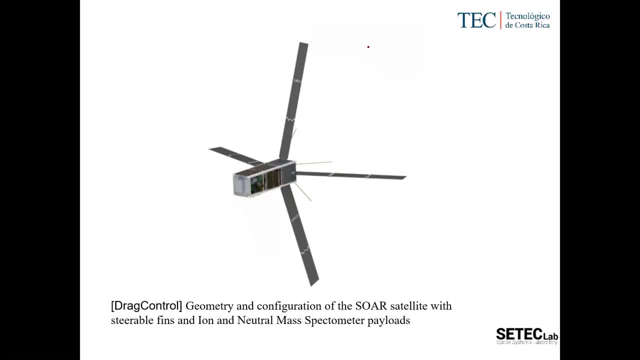 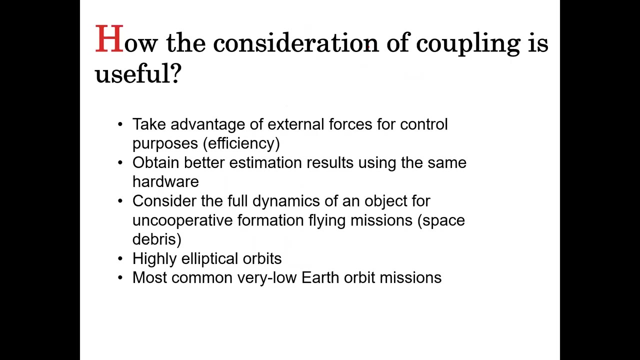 because they're relatively inexpensive And we can do very, very advanced. we can use very advanced dynamic systems and control to actually prove new concepts with the spacecraft dynamics. So how is the consideration of coupling useful? First, take advantage of external forces for control purposes. 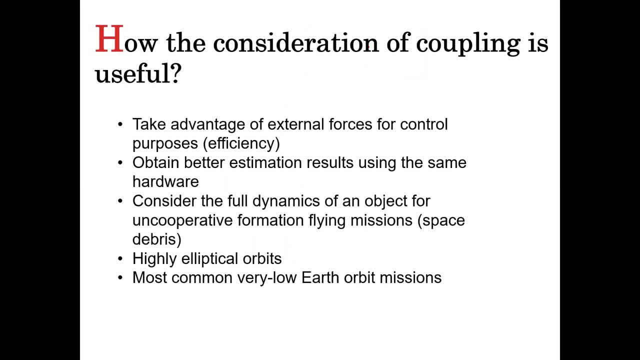 efficiency, I mean you are not using your own energy. Obtain better estimation results using the same hardware that I've repeated for. Consider the full dynamics of an object for uncomparative formation- flying missions, for example, caching space debris. I didn't take into account this in my scenario. 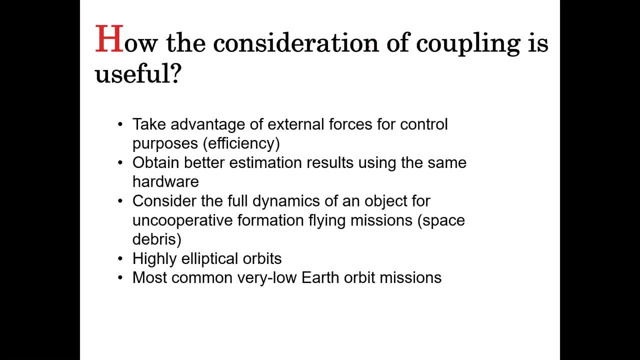 but this could be taken into account for highly elliptical orbits Or say, for example, to make more common very low Earth orbit missions. I mean we're talking that usually Earth orbit missions, like very low Earth orbit missions, like the first one that I showed you. 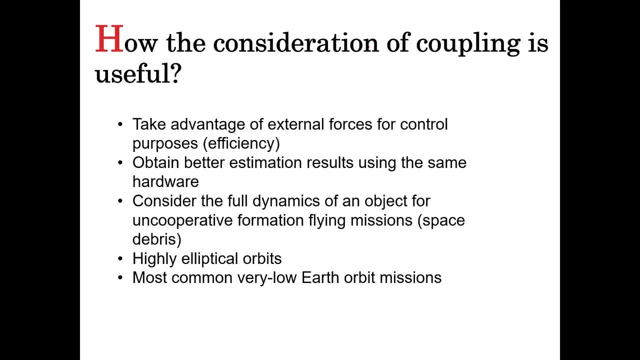 they're not very common because they take very, very few time. But imagine that we could launch a satellite from the International Space Station and instead of taking us two years, we can prolong this mission to double because of our mechanical design. This would be very interesting. 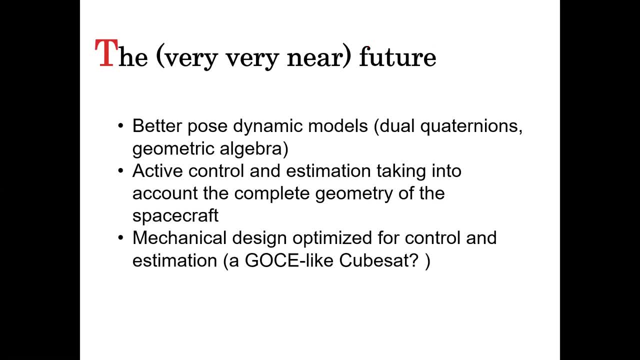 In the very, very, very near future we can take into account better post-dynamic models. I've been working with dual-continuous and geometric algebra. There are mathematical models where the orbit and the altitude dynamics are in a single entity, So the mathematics itself are more simple. 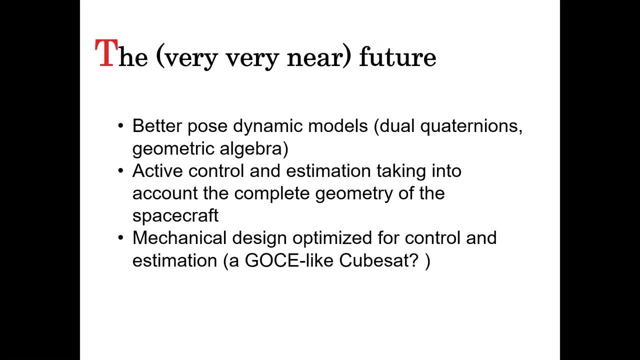 You have to learn them, but they're more simple: Active control and estimation, taking into account the complete geometry of a spacecraft, meaning spacecraft design, to take into advantage this coupling And mechanical design optimization for control and estimation. Say, for example, a goose-like cubesat. 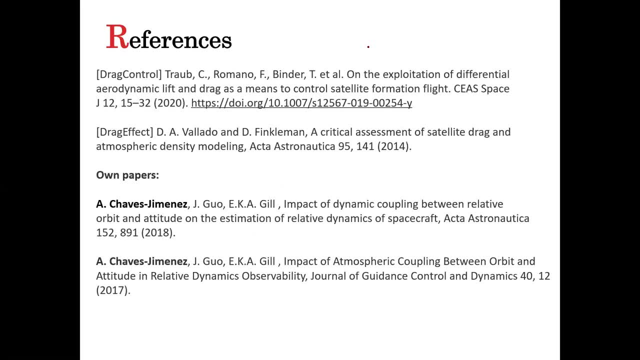 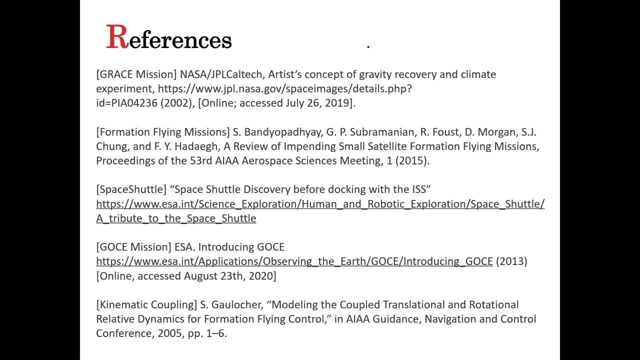 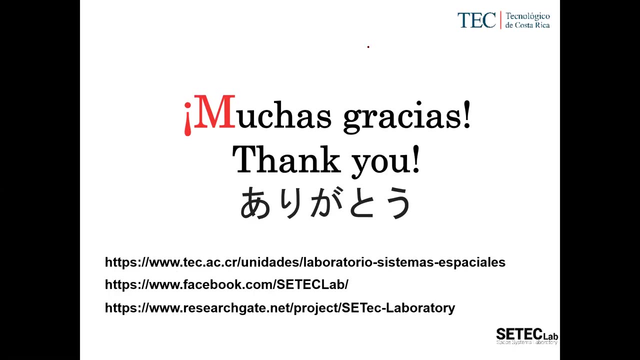 And this is my talk. These are all the references that I use, including my own papers, And I hope you like the talk as much as I like to create it. And again, it's an honor to be here And I'm very open to any questions. 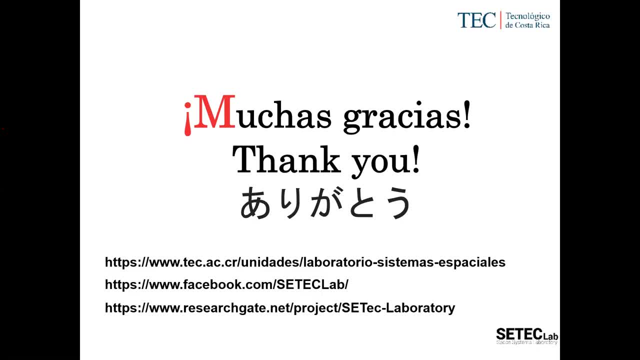 If you might have. Okay, Thank you, Adolfo, Let's go with the questions. Anyone, Timothy, I thought you had questions. Thank you, Professor Maeda. Well, my question is maybe not from what has been presented. 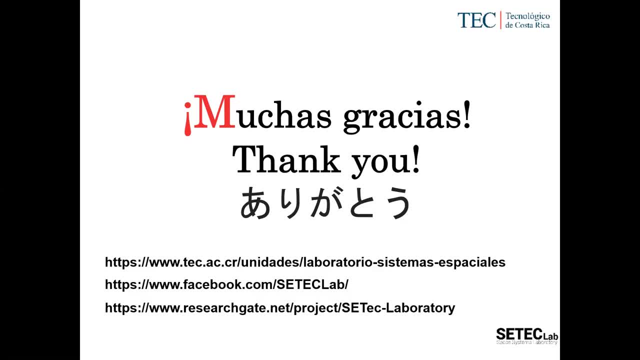 But yeah, my question was what can be the best option- let's say for a satellite mission or for getting water quality- let's say for the water body That I want to take an image when the satellite is passing through- And what can be the best method? 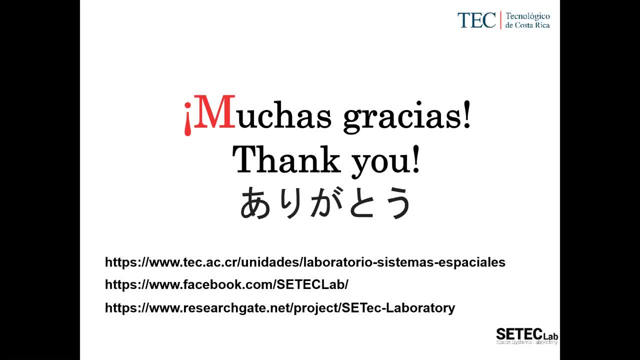 Let's say we've got the passive and we've got the active method using a 1U cubesat. Well, it really depends on the position of the mission itself. It really depends, If you want to, to point the satellite to the place where you're taking the image. 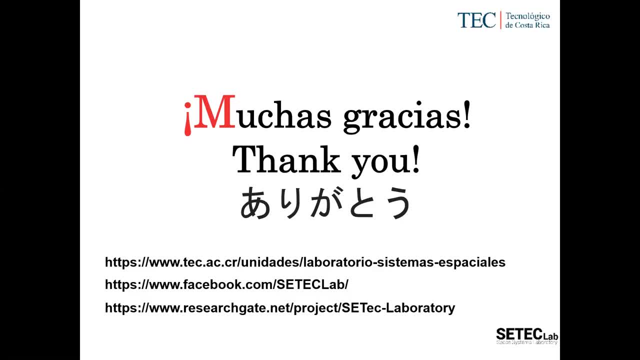 or if you are just trying to get the satellite always to point to Nadir, then if it's always pointing to Nadir and then you take images all the time, like Planet does- I think Planet Labs does this- then probably if you're able to do it in a passive way, 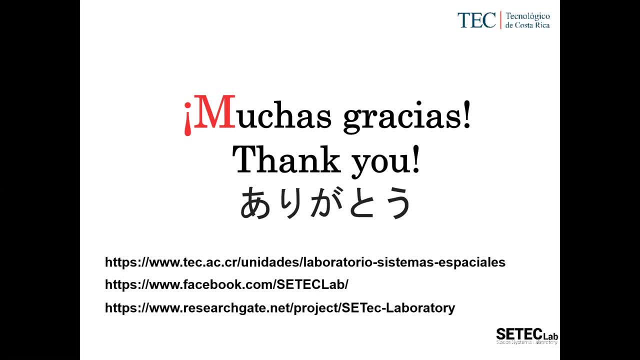 it would be way better for your power consumption. But if you really need precision, you'll definitely use probably rotation wheels, which are very expensive from the point of view of mass. They're very expensive from the point of view of power. But if you need them, only say less than 5%, less than 1% of the time that you're in orbit. 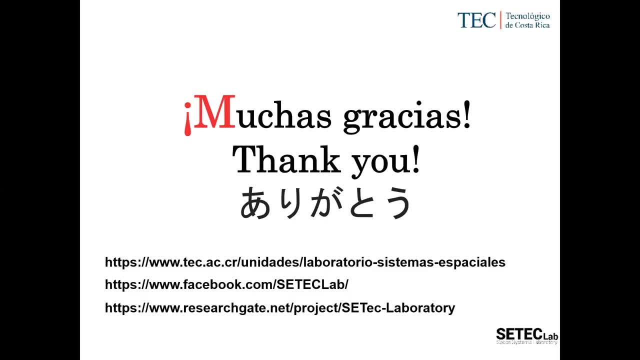 then it might be worth it, But it really depends on your mission. We're actually doing this for the GW satellite, The GW satellite in George Washington University, And their experiment is that they're testing their own propulsion system. So we're not using rotation wheels. 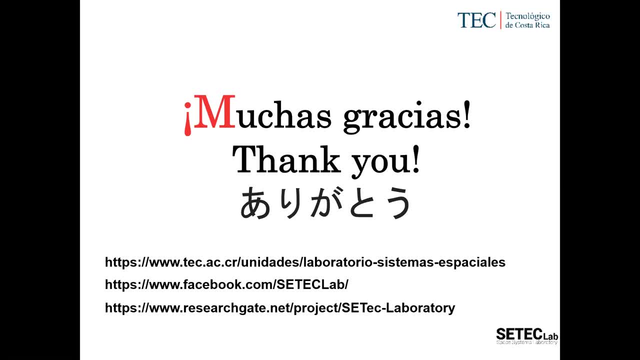 which will make it very difficult, But that's actually the experiment itself. Typically, rotation wheels are the ones to select, But it really depends. So, Timothy, recently Guatemala launched the first satellite. It had a very good camera And I think it was something for water quality measurements. 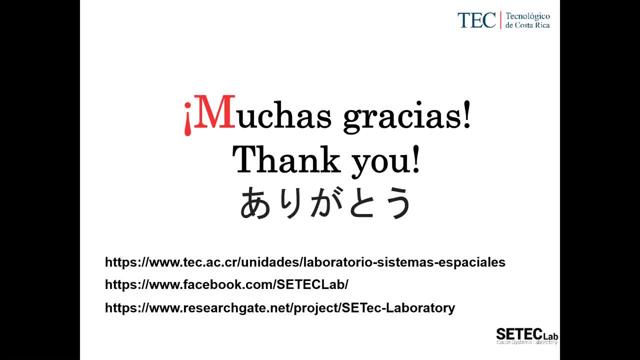 And so that camera had to be pointed at their lake. So, Adolfo, do you know what they did for attitude control? They don't. They have a passive system of attitude control, using the magnetic coils that they have Only to stabilize the system. 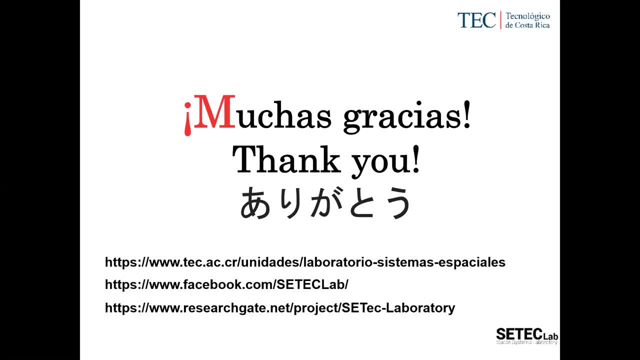 And what they do is they take photos and they use the ones that are okay Because the system they use they wanted to test the payload, But they are not required to have a proper photo every single time that you pass by Guatemala. With only a few photos, they could get the whole mission to be a success. 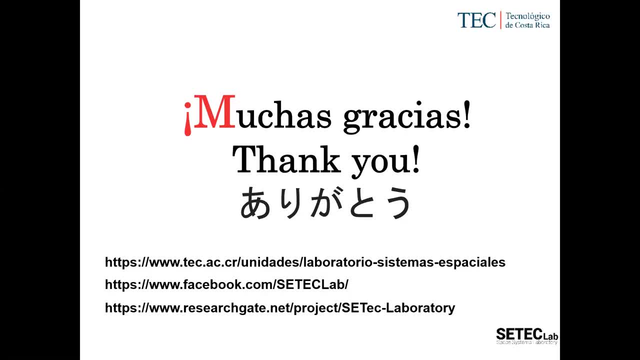 So they don't have a. As far as I understand, they don't have an active control system. So, Timothy, for good control people use reaction wheels, But in a 1U CubeSat it's not done too often for the reason Dr Adolfo said. They're power hungry. right, They're power hungry, They're mass hungry. I mean, they're not even that expensive, But they are. I honestly don't remember if 1U CubeSats already have reaction wheels. I guess they do. 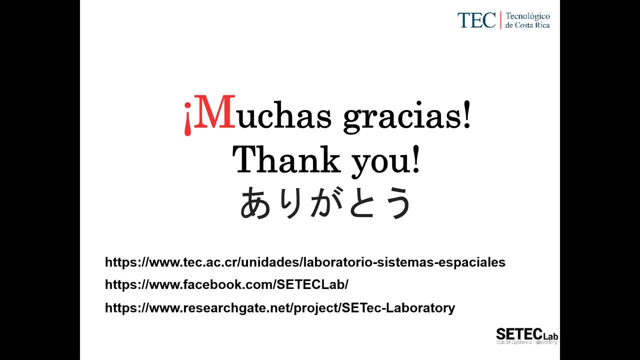 Because typically 3U CubeSats are the ones with the reaction wheels. We had one at Teodef. I also work in a project at Teodef. We had reaction wheels, But it was a 3U CubeSat. It's a very good question. 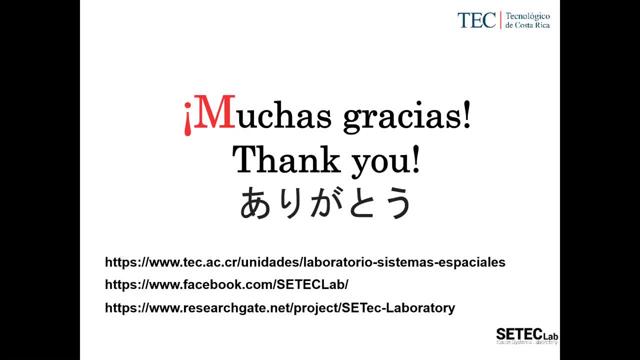 Honestly. Honestly, I don't know. I would guess it has been used. I would even guess that maybe you have used them in 1U CubeSats, But I don't know. Have you actually, George? Oh no, 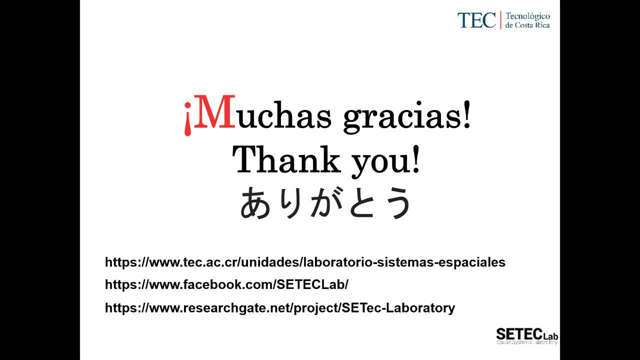 Professor Cho says they're too heavy and too power hungry. Oh yeah, They are. They are Absolutely, I agree, Because the 1U doesn't have enough surface area for collecting. Yeah, Yeah, Yeah, Yeah, Yeah. 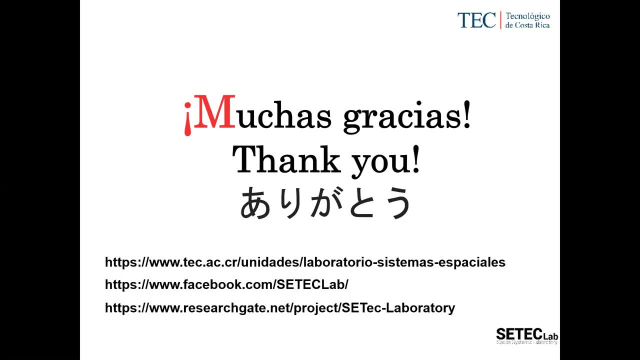 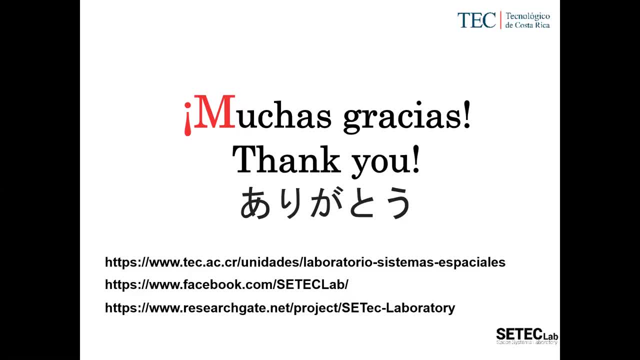 Then you might use less energy to actually stabilize the satellite, because the passive system itself does stabilize it, But this hasn't been done too often. This might be done, I believe it might be gone. it might be wrong, and this is something i want. i is one of my future research, uh approaches actually. 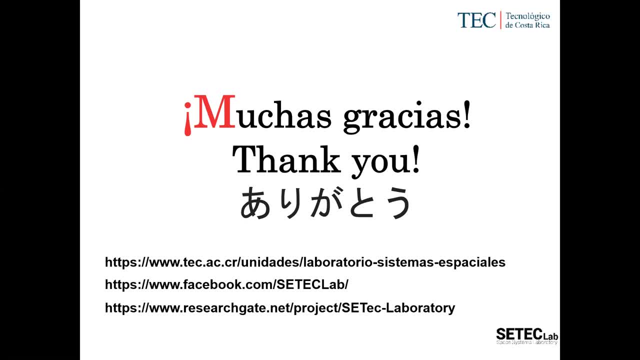 anyway, timothy asked that question because, uh, birds five is in the design phase and and they're trying to figure out, um, how the satellite should work. i would say, for sure that you, you need to use the magnetic, the magnetic systems for for control, because they're inexpensive, they don't. 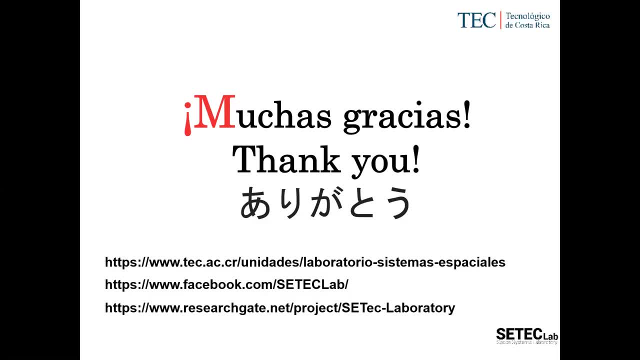 use a propulsion system and they can stabilize the satellite in a good enough way. i don't know if that's good enough for um for to point to nadir, because if you want to point to nadir you need a three, three axis control and the magnetic system. thus it only gives you two axes. 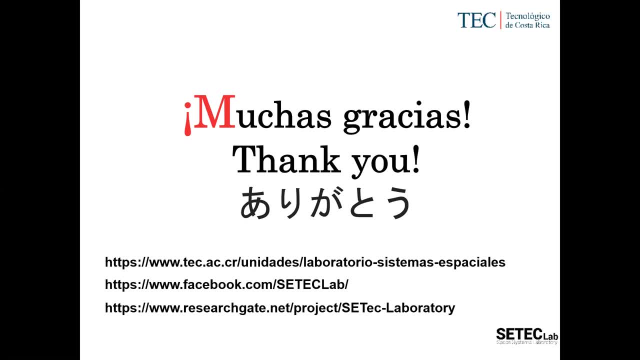 so yeah, yeah, in general, the bird's philosophy is just to stop the tumbling. point pointing is too difficult, but but at least stop the tumbling. yeah, yeah, yeah, yeah, for sure, the tumbling with the, with the magnetic system, should be enough right now. do you have a question? I do, it's. 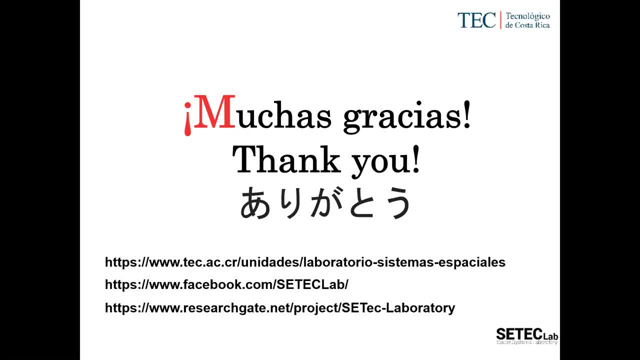 regarding that low earth altitude spacecraft are really. I really need it for a lot of communications systems and there is a really good interested in reducing the altitude to work with a lot of spacecraft due to speed information from the speed of the information. so I was wondering: why do you? 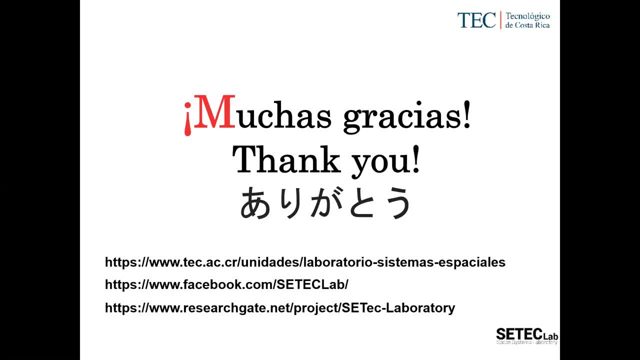 think that. take coupling dynamics. it's taking advantage basically of one thing that was considered, as you mentioned, perturbation, but that now can be an asset to, to come to aid and control. so why do you think it? it is a topic that is most that it's hot today and not before when, for example, with Starlink. 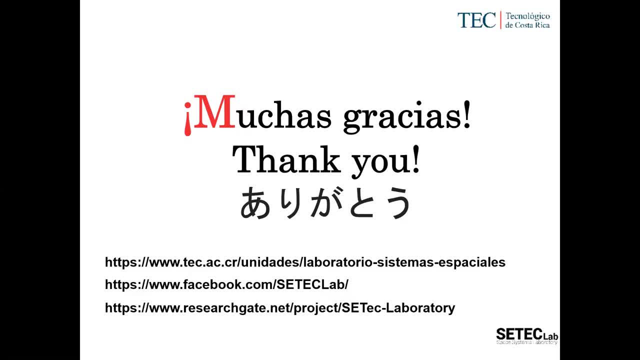 we're having a satellite constellations, for which which its selling point it's uh internet speed. so I find it difficult to to consider that it hasn't been uh considered before. right, it has been, it has been, but it's it's hasn't it hasn't. 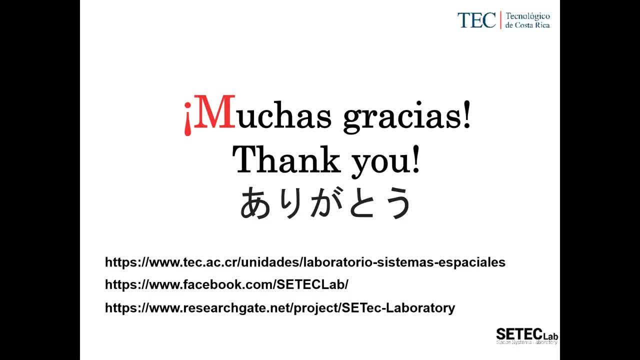 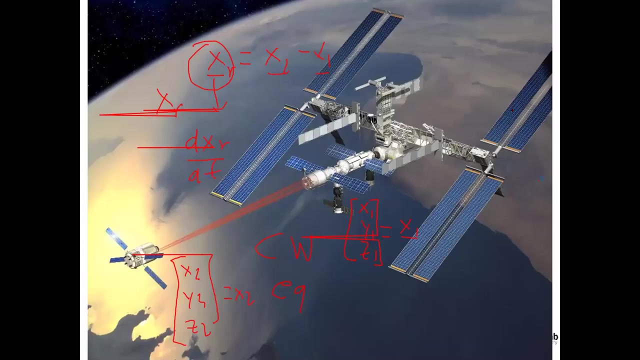 been considered before because, um, constellations are very new hot topic. it has been always a topic. now I have topic why? because, as I said before, um, usually the relative Dynamics that were important for for our research were this kind of relative Dynamics, and this kind of relative Dynamics we. 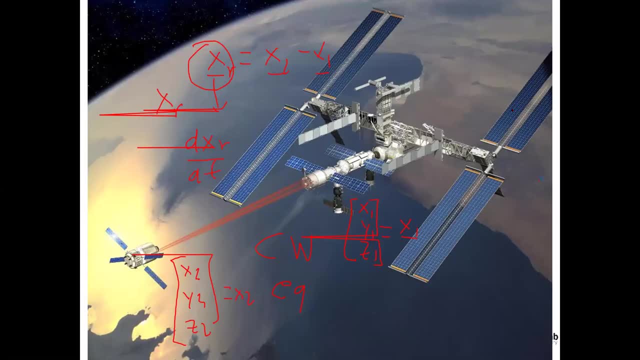 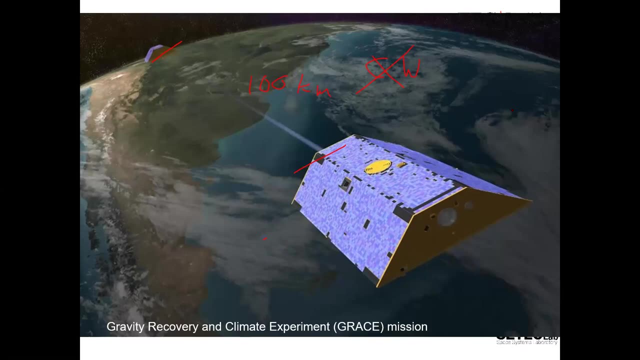 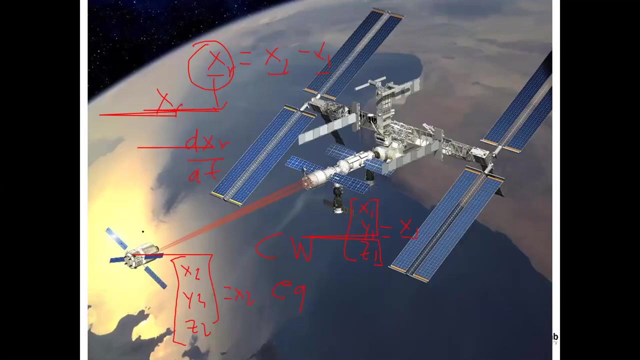 had good enough instruments, we had good enough information for us to do this, but when we want to do this, we're talking about something completely different. we're talking about a different Beast. I mean the correction that you can have on system: and this is a TV from, from Europe. this is, this is automatic. uh, it has enough sensors in order. 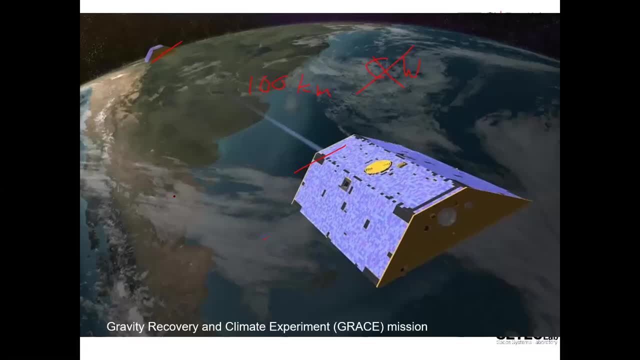 to for it to connect. but when we have to point a laser 100 kilometers apart on two spacecraft that are very small, we can use all the help we can get right um. why is it not used? um? one of the reasons is because the tendency among uh aerospace engineers is to simplify the dynamic models. 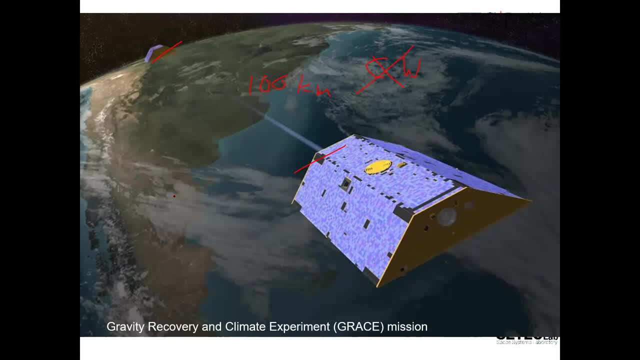 usually the uh. the use of more advanced dynamic models comes from the realm of mathematics, not necessarily space engineering. so, um, why not using them? it's a very good question. the answer is usually that you try to simplify using. because you have a microcontroller that is not that capable, because you buy GPS or you buy 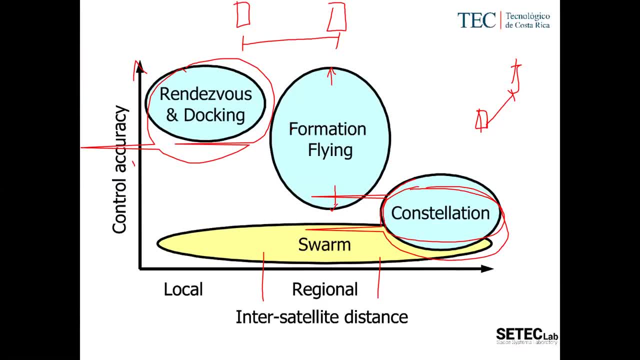 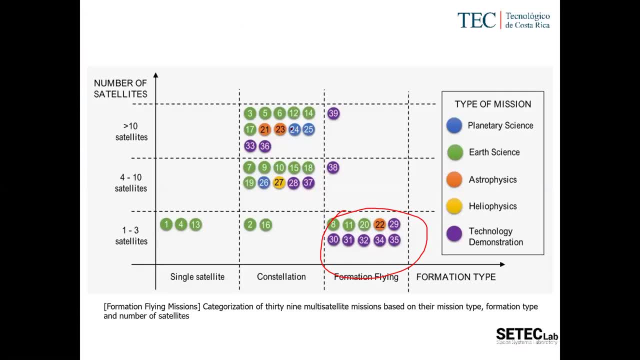 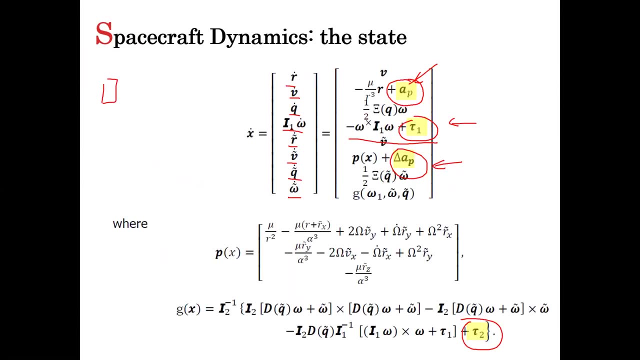 other systems to make it more precise, but you don't take into account the mathematics. um, I don't know. honestly, it really beats me that it hasn't been taken into account. I think the mathematics are a little bit dense, honestly. I show you only the small uh equations. there are quite a lot of more equations and I think the reasons are are first: 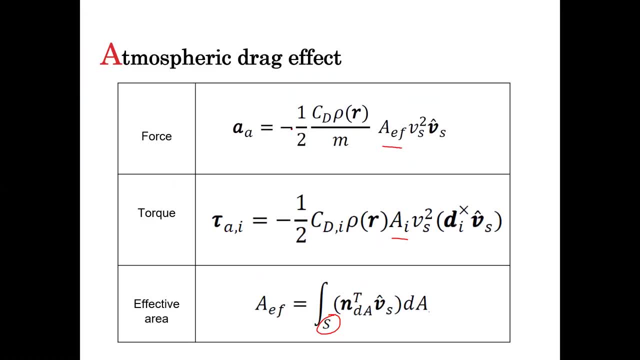 it hasn't been necessary, but now, because of the missions we're working about- talking about, say, for example, Starlink- it has to communicate between two laser, I mean between two satellites with laser. this, this level of precision. now we need millimeter level of precision before we. 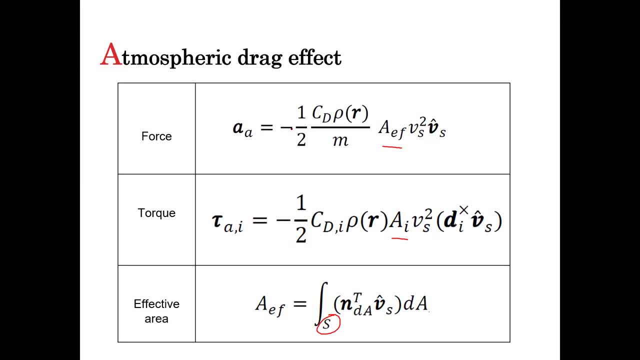 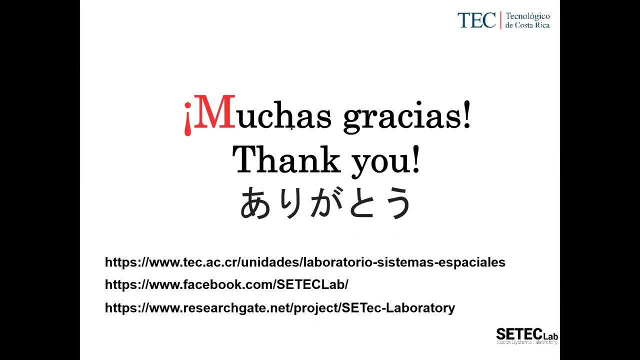 needed meter level of precision. so this is one requirement. so we need to store as much as possible- will be the computer capacity. Now, the computer capacity allow us to have more and more complex models and I believe we are soon to be to the point with that. we 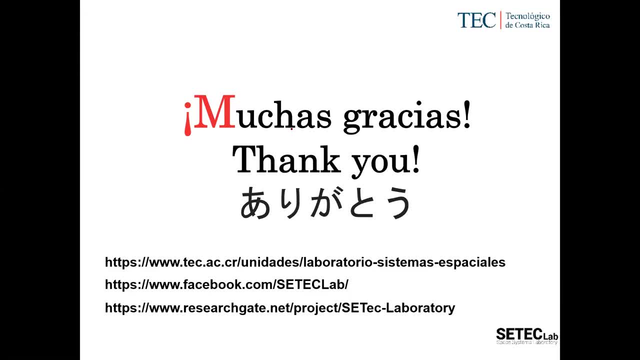 don't need to simplify our models. I don't know if that answers your question. It does. I think, as a summary, it could be the fact that we have now more computational power in a more dense, in a denser mass, because we can have 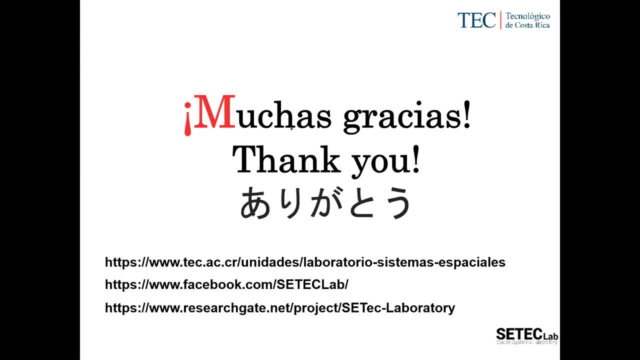 computers that can do thousands of calculations in a thousand of the space that we could do before. So yeah, I am guessing it has to do with what you said before of the Moore law, right? Yes, that's one, and the second one is that we 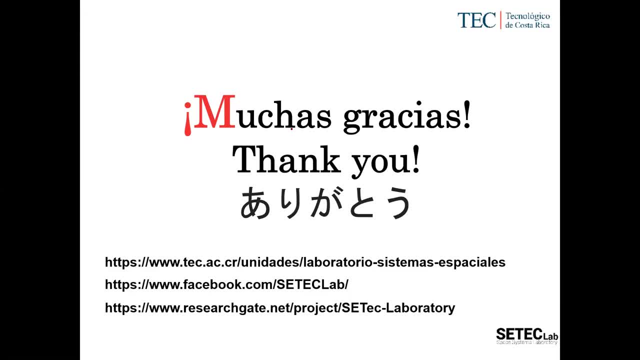 need it now and they don't need it before. Go ahead, That answers my question. thank you very much, Elov. No, thank you. Okay, let's have more questions, please. I have a question. Yes, Dr Jiménez, I would like to know if, in a further perspective, can we imagine? 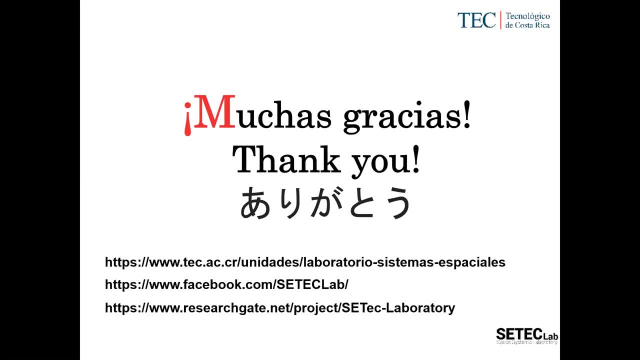 let's say coupling or having a coupling of more than two spacecrafts, like having maybe one spacecraft, Yeah, one chief and two deputies or more, or one deputy with two chiefs, I don't know if it's, if it's possible and or interesting. yes, both. yeah, the model that. 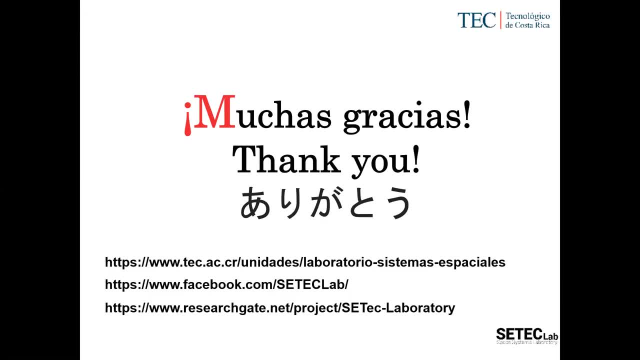 I use on my thesis can be expanded to any amount of spacecraft that you want, and it would be interesting because the most dynamics you have, the most sources of of errors you might get. so the better your model, the better you will get, and the most the most spacecraft, the more accumulated error. and if you use an 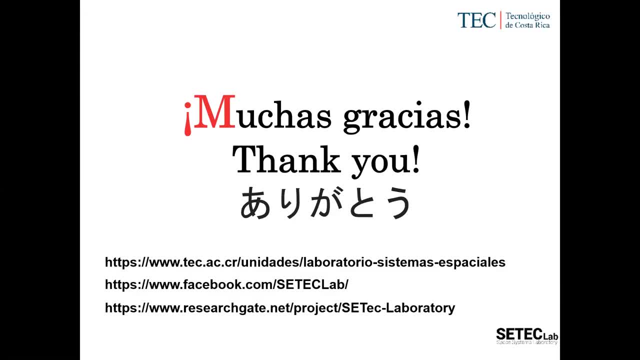 estimate, better estimation model, then there's less later error and they can work better. honestly, it will really surprise me if constellations like the Starlink of SpaceX will not use this kind of model. but but- and this is a very, very, very large but- if you under, if I understand. correctly, Starlink is about 650 kilometers. it's about 700 kilometers and and you might have a reason why in what we are talking about today on the perturbations, the perturbations may make more difficult the lemon of control that they need. So I guess that's the probably answer why Starlink. 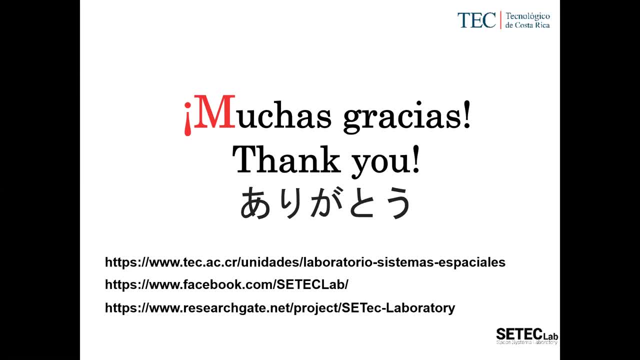 is higher in orbit, But taking into account this could allow us to actually using passive control and spending less and less in control and getting better estimation systems and using the satellites in lower orbits. It could be used even for the orbit in the spacecraft itself. I see, Yeah, I don't know if that answers your question. Yeah, 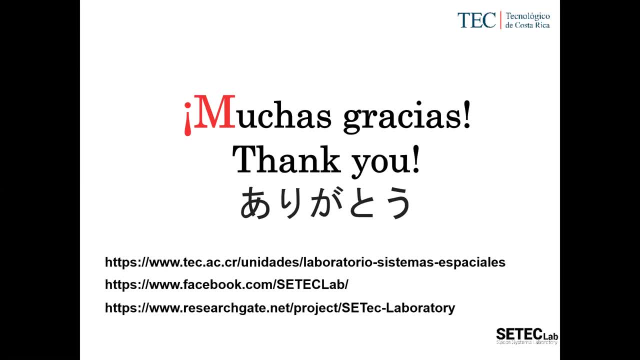 definitely, Definitely Okay. thank you, Thank you very much. All right, Okay, who's next? Hello, Dr Adolfo. Yes, Thank you very much for your presentation. My question is about your model. Yes, Thank you very much for your presentation. My question is about your model. 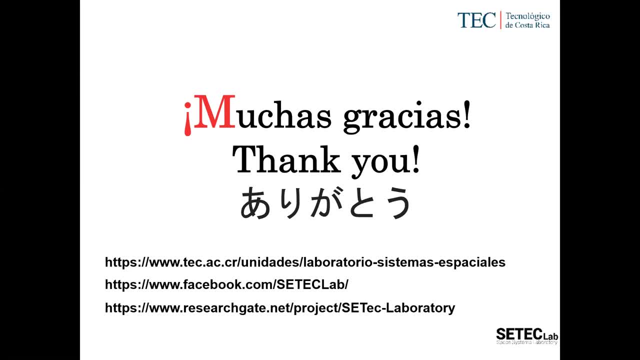 For the coupling effect. I see that you concentrated mostly on the atmospheric drag effect, right, Yes, Which is basically the external source of errors on the satellite. You also talked about the level of accuracies for different mission scenarios, And we both know that. 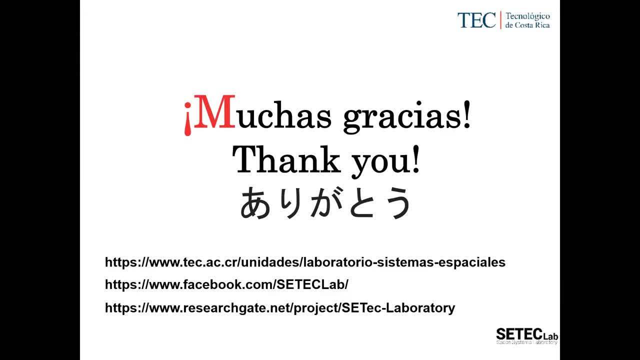 the higher the mission requirement, then actually you have more requirements on the point accuracy, For example, you talked about the Starlink LASAR communication platforms- Yes, I believe. by the way, I'm actually. my PhD is actually considering optical communications and how we can help the pointing between a spacecraft at the ground station or inter-satellite scenarios as well. 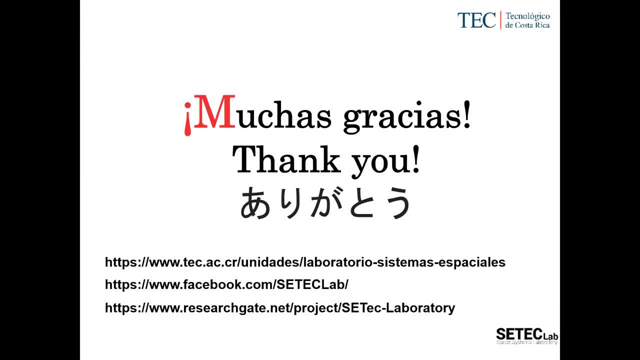 Yes, My question is about your model. Have you considered internal inter-satellite scenarios as well? Yes, My question is about your model. Have you considered internal inter-satellite scenarios as well? Yes, My question is about your model. Have you considered internal? 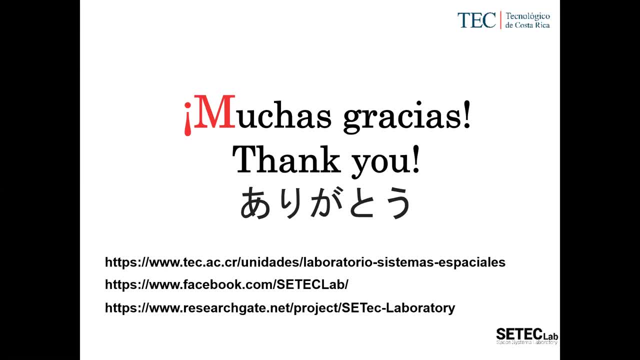 effect as well. For example, reaction wheels are like the holy grail for pointing when it comes to inter-satellite LASAR pointing and LASAR communications and all that. But then you still have a lot of problems with reactions in itself because there are a lot of imbalances. 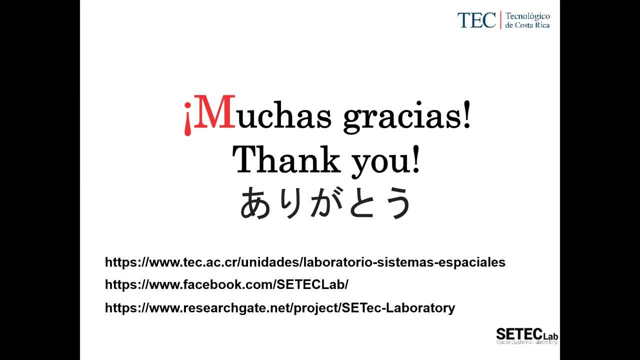 that are being experienced in reaction wheels, And this can pose a lot of effect on the kind of models that you develop. So the question simply is: did you consider internal effects Aside from the external disturbances, like the atmosphere? very dry, Very good question. The answer, the short answer, is no, We didn't consider the internal effects. 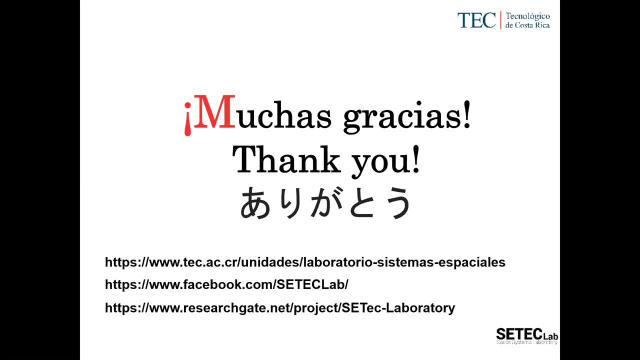 And there's a reason for that. The internal effects. you know them And this is important, Because internal effects I mean if you're working on your reaction wheel, you know how much force you intend to use on your reaction wheel, So you can use the. 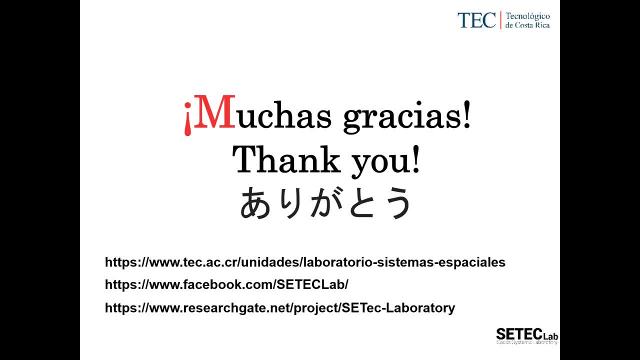 the dynamic model doesn't have this level of not knowing what happens with the dynamics in the case of internal dynamics, because internal dynamics are in your control, But with the reaction wheels, which is the case that you mentioned, there is a lot of problems. 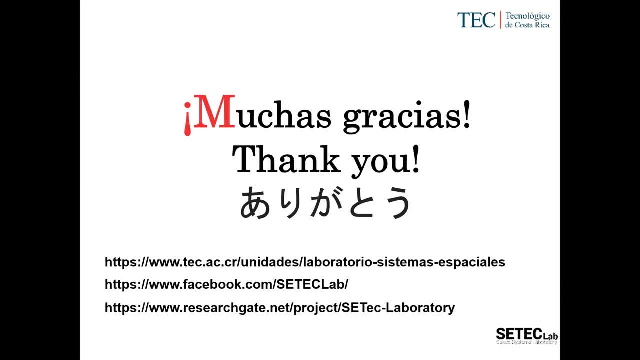 with the, with the- what's the name of this? with this part that is, you know, going away and away and away from the possible phenomena reaction on a much slow speed. benefit, That's isso, Tomé. But with the reaction wheels, which is the case that you mentioned, there is a lot of problems with the. what's the name of this? With this part that is, you know, going away and away and away from the possible phenomena reaction while there's motion on the radar. And, uhont gentleman, you might master example of how dynamic the actual momentum is in the actual body. But yes, everyone knows it's this stuff. 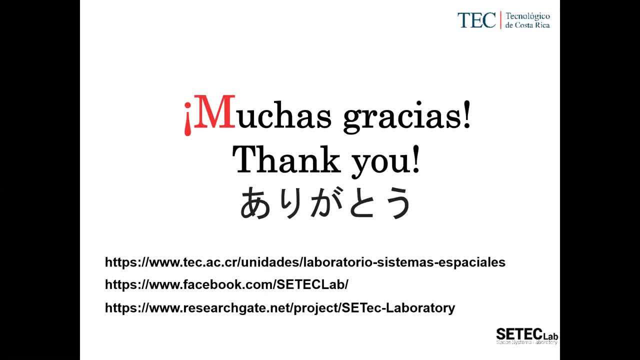 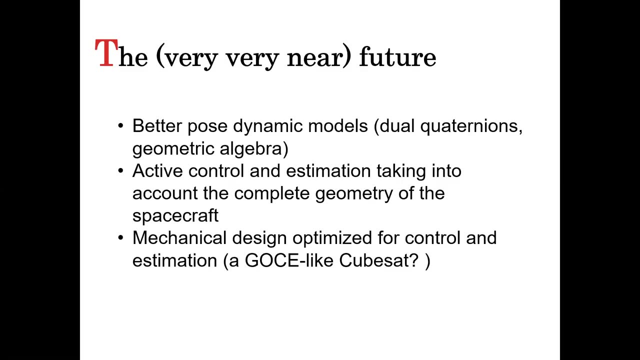 from the possible force that you want to have, And this is also the source of estimation. Could it be taken into account? Yes, actually I talked about geometric algebra and dual quaternions. And why I talk about this? because sometimes, when you do attitude control, 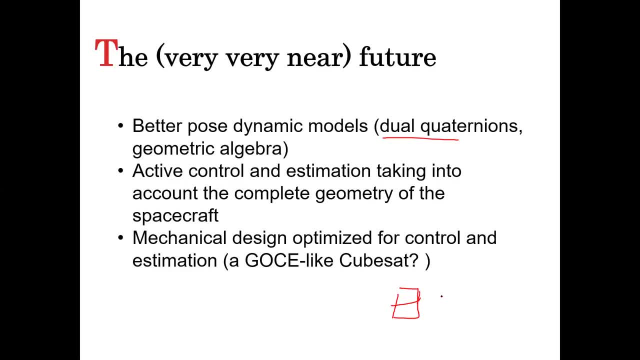 you don't take into account how the orbital dynamics of the spacecraft is going to be modified, or vice versa. For example, if you have a propulsion system here, this is really bad. Okay, If you have a propulsion system here and you turn it on. 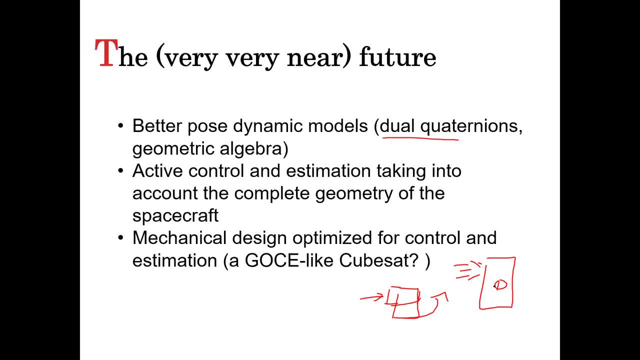 then this is not going to be in the center of mass of the spacecraft And this is going to move the spacecraft forward, but it's also going to move it in some way, And usually what we do is that we compensate this effect by using the reaction wheels at some point. 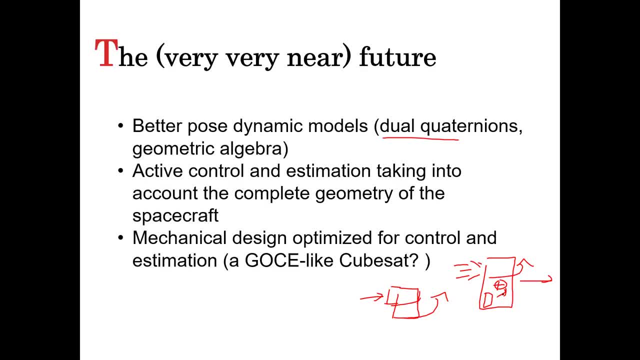 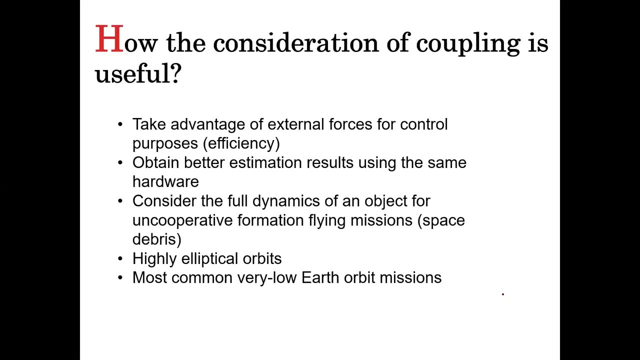 or things like that. So we don't take into account this couple dynamics, And this is actually important. If you use the control, if you design the control taking into account the couple dynamics, you could be more efficient from the energy point of view. 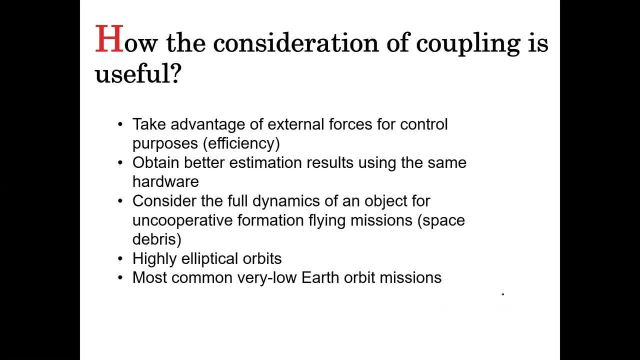 And this is actually something that we want to test in George Washington CubeSat project- that we use control methodologies, control algorithms that take this into account, because we're going to use post dynamics- I don't know if you know the term, but we talk about post dynamics when we talk about orbit. 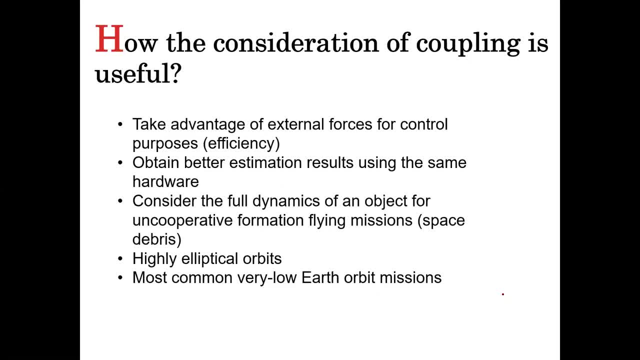 and attitude at the same time. So, when we talk about post dynamics, taking this into account together could allow us to focus more on the optimization of the energy usage, And this could be very interesting, And this is not as common as it should be. 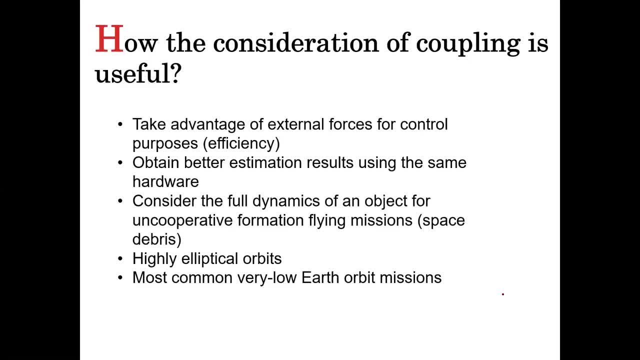 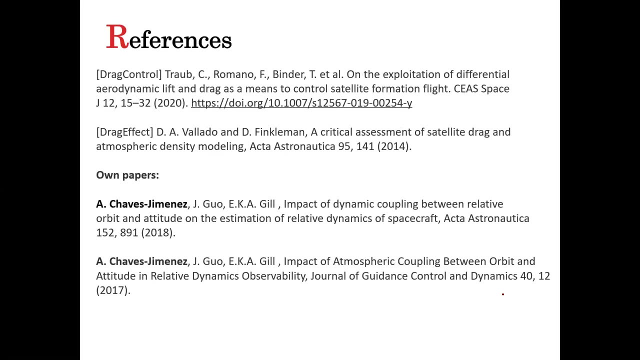 Because, which is very curious, because usually aerospace engineers, they know about this coping due to the aerodynamic part of their studies And, yes, it can be taken into account. I don't know if I answered this, your question. I get a little bit lost, I think. 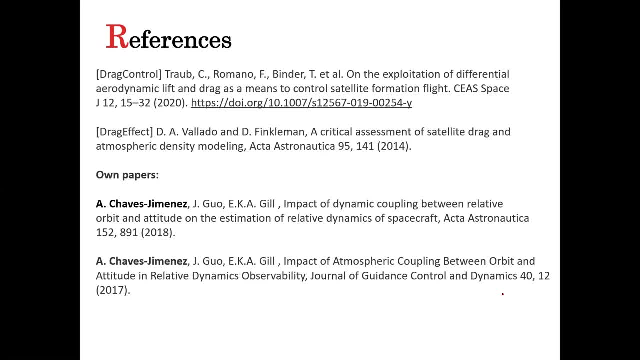 Yes, you did. Yes, you did. I can understand it can get very complicated for just one PhD to take into account several, But I want to Exactly Well what I'm trying to focus on for my PhD here in Q-Tech. 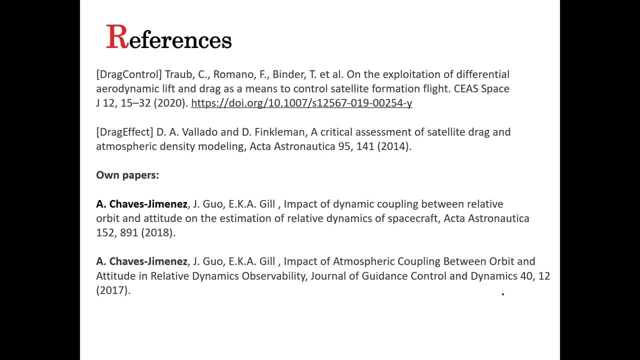 is. I'm trying to model different kind of platform disturbances. It could be atmospheric drag. It could also be micro vibrations in the satellite which can be generated by reaction wheels or maybe deployments of flanges or anything. any kind of vibration which causes a high amplitude movement like a GT. 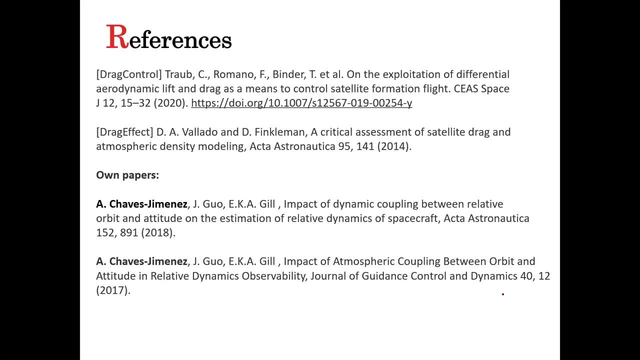 And then also we have a lot of data on the platform. So we have an optical bench with MEMS mirror, staring mirror and some optical devices that we're using to simulate that. So it'll be very interesting actually to keep in touch with you. 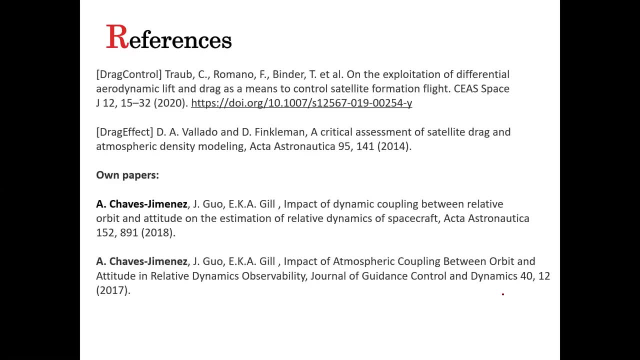 I'm not really an altitude control expert, I'm more of communications. So it's interesting to, at one point or the other, have more chat on this. I will be All be more than glad to cooperate with Q-Tech. I will be more than glad to cooperate with Q-Tech. 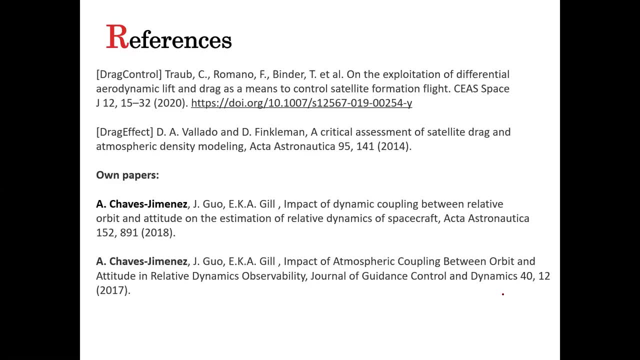 Q-Tech in these matters. Actually, I'm very glad of this talk because I can show what I know a little bit about and which could be a possible areas of cooperation, because we have been working in cooperation with Q-Tech in remote stations. 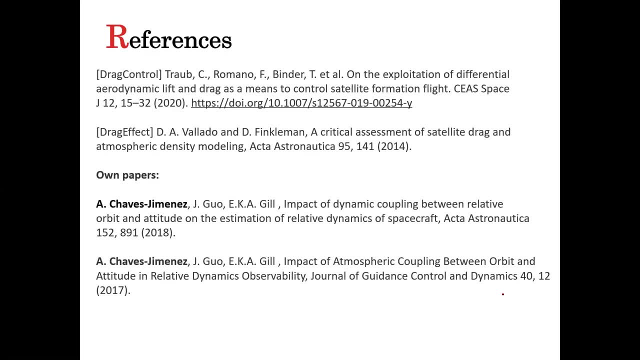 but I really want to cooperate in the control and estimation area. I'll be more than glad to discuss this with you. Yeah, thank you very much. You're welcome. thank you, Please, please do really. Ah, Dulani, are you still with us?